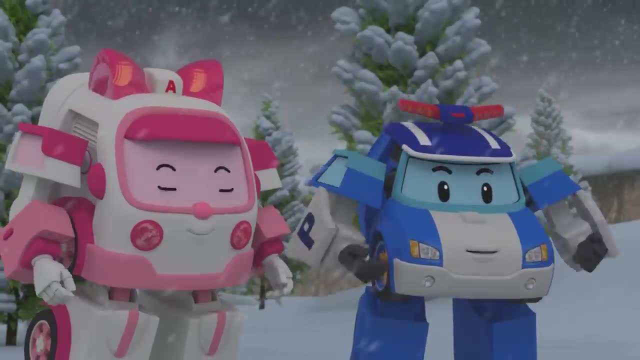 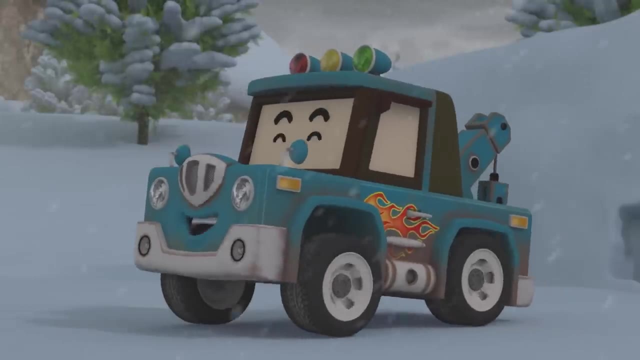 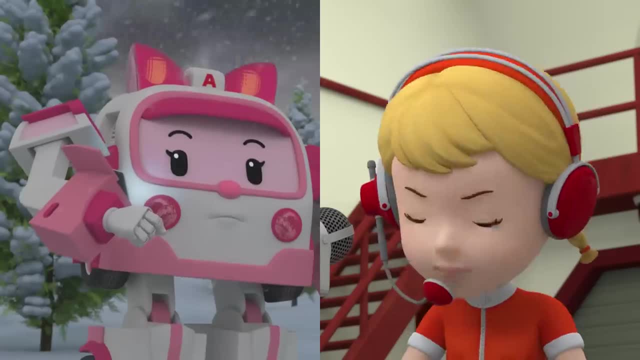 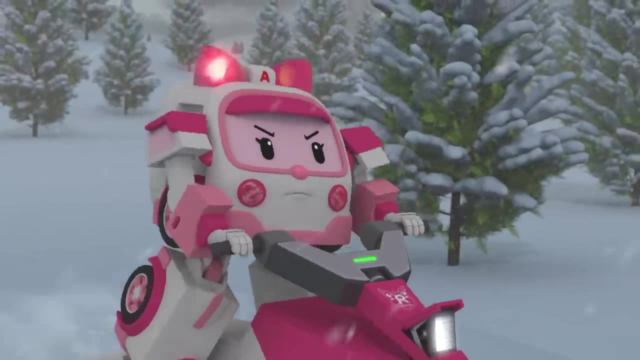 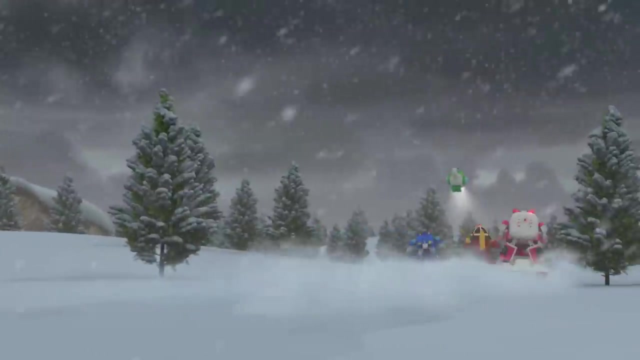 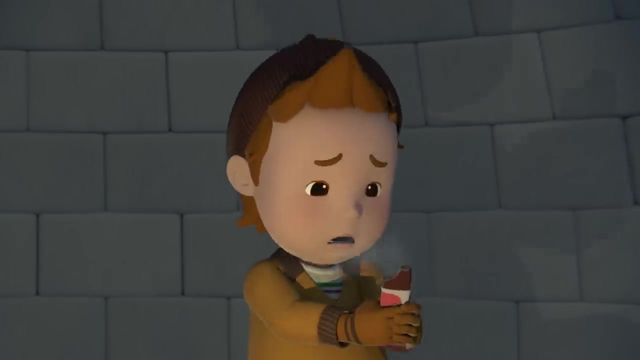 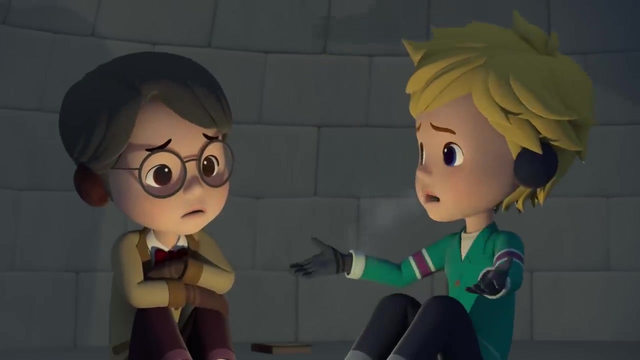 The kids were playing on Apple Street, but they haven't come back yet. Dispatch the team right now. Understood? Ooh, this is the very last of our food supply. oh, it's frozen solid. we're all frozen solid. what if we're not discovered for years like dinosaurs? 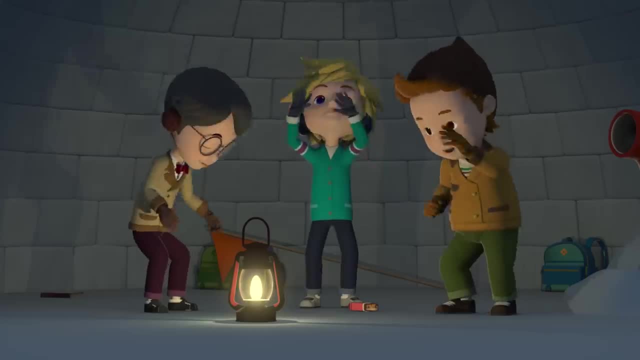 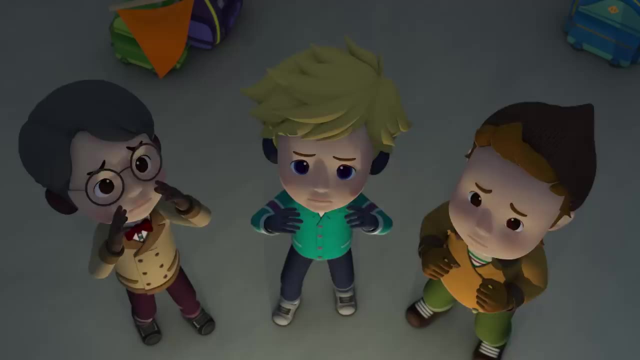 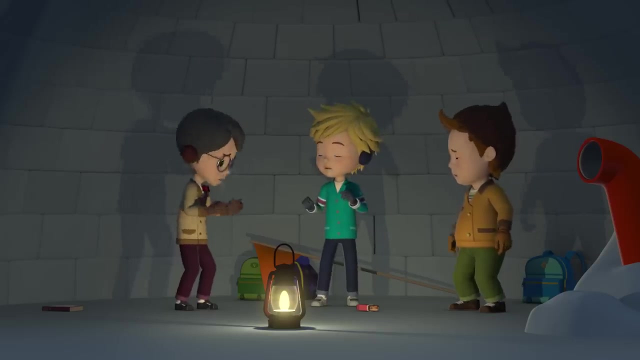 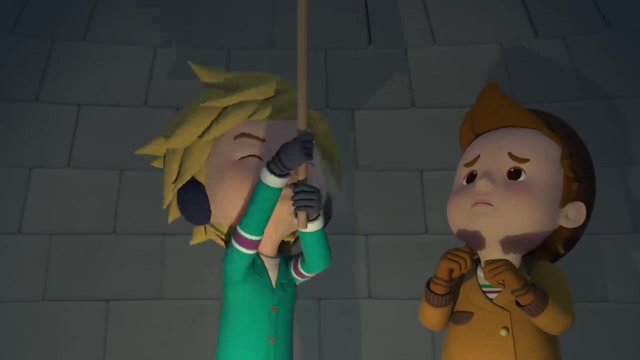 rescue team. we're here, peter johnny. charles, listen, if you hear us yell down here, can you hear us, peter johnny? i don't think they can hear us at all. this is the end. oh, oh, wait a sec. uh, we're down here, come on, hello. oh, what's that? 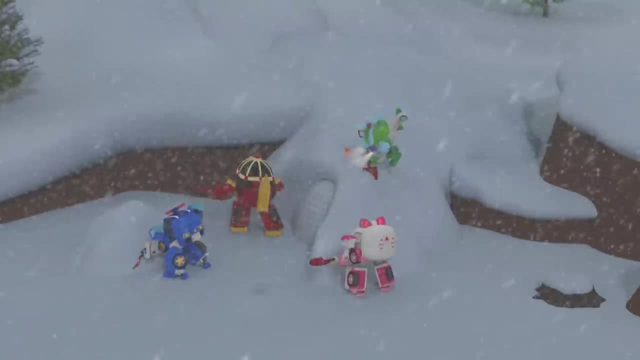 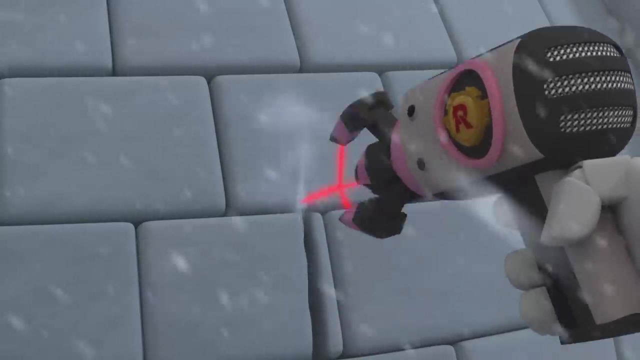 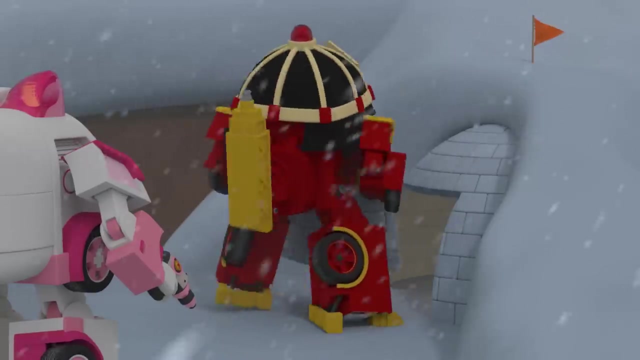 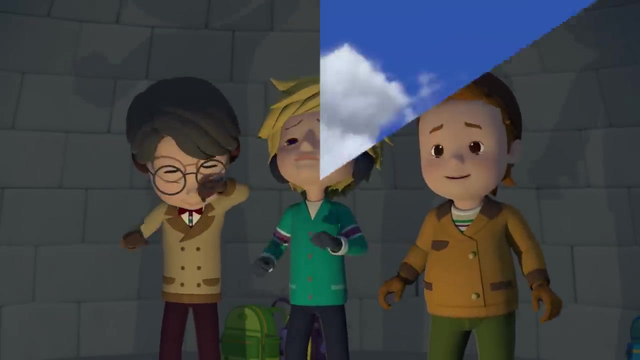 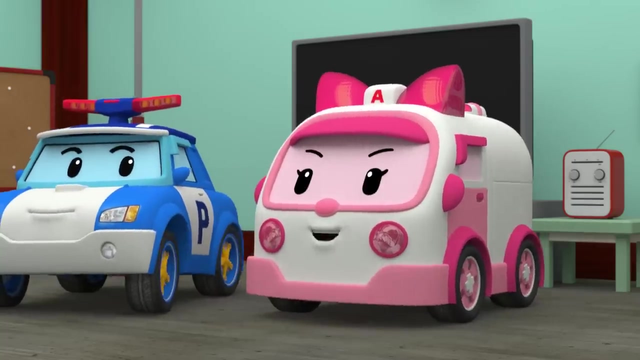 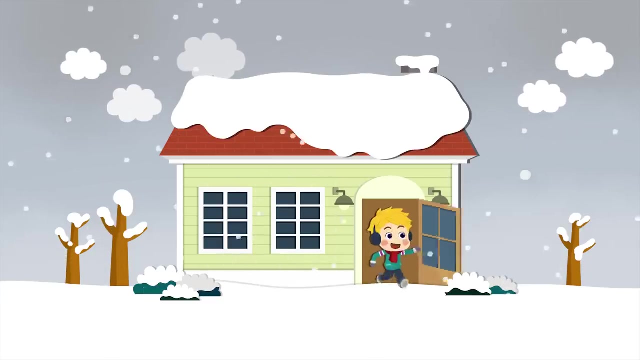 oh, i see them all right, stand back. hey, kids, you okay. ah, thank goodness you're all safe. thank you. when the snow is горяча, is heavy, there are some things to remember In winter. pay attention to weather forecasts to see how bad the snow is expected to be. 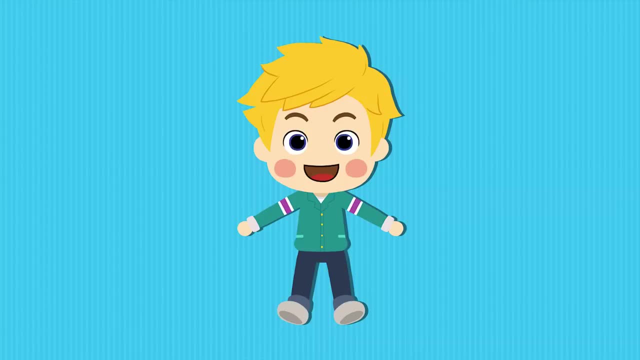 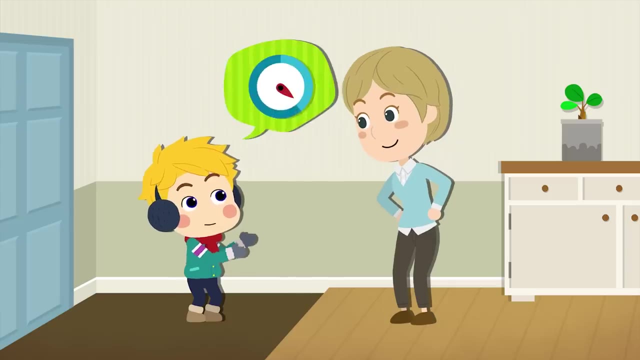 On days with extra heavy snowfall, it's best to stay inside, And if you do go outside, remember to wear your gloves, a scarf, warm shoes and something to cover your ears. Always tell your family where you're going and when you'll be back. 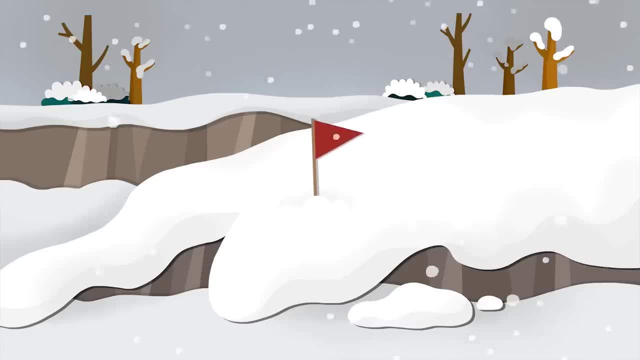 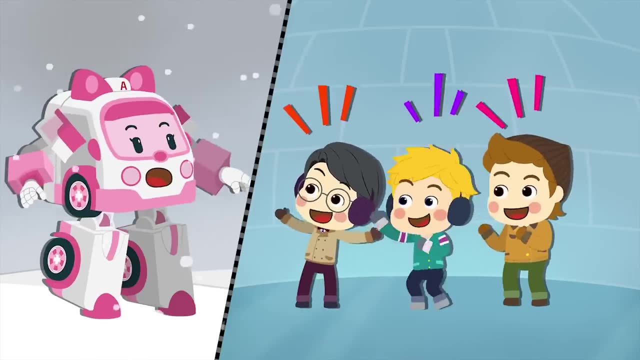 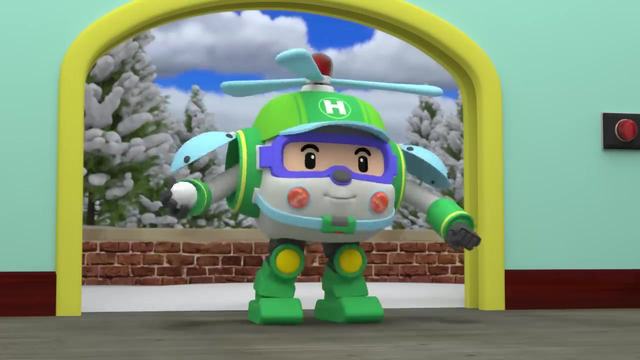 If something happens and you need help, try as many ways as possible to signal for help. While you wait for help, move around to keep your body temperature warm and remain calm. Got it? We'll do our best, You guys. It just stopped snowing. 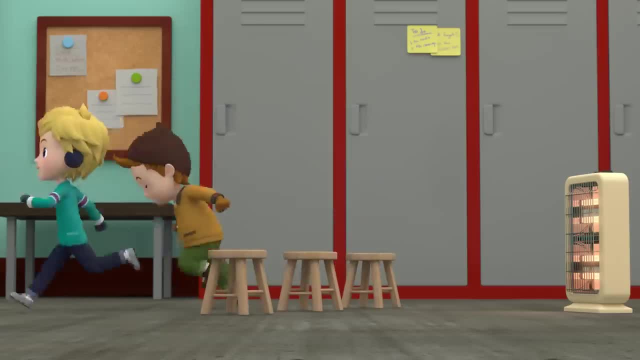 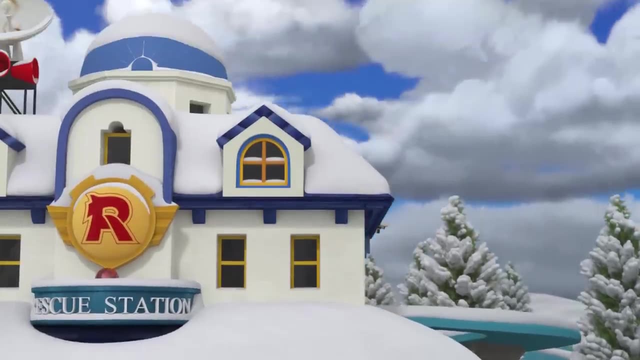 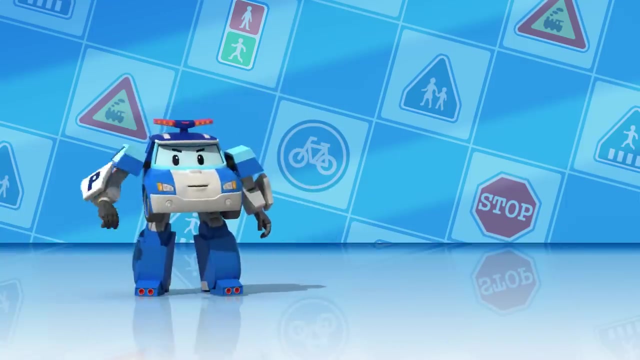 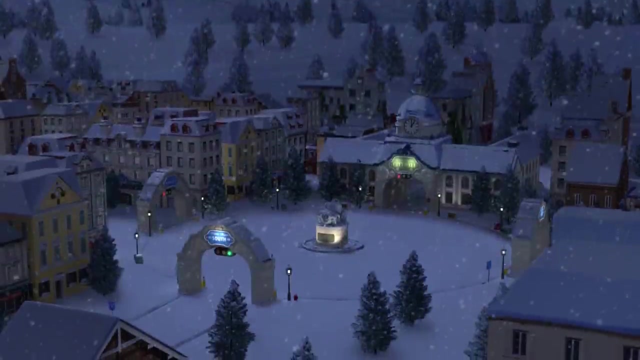 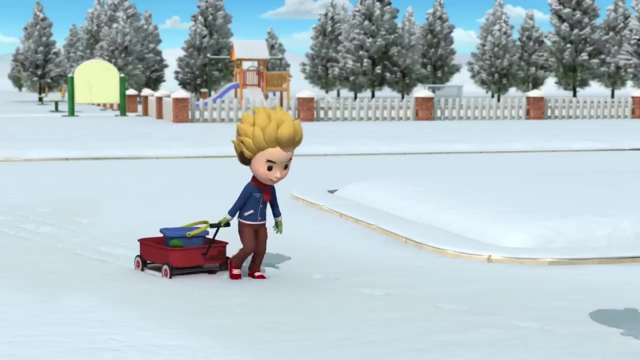 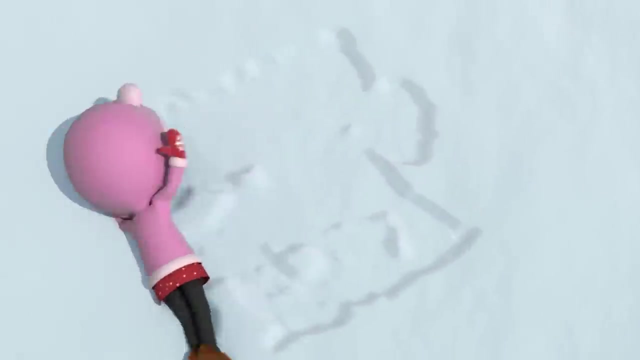 So snowball fight, Really All right, Snowball fight. Well, we do what we can, Hm, Oh yeah, Snowy Day Safety Rules. Hooray, Wow, Pretty snow. Huh, What's that for? 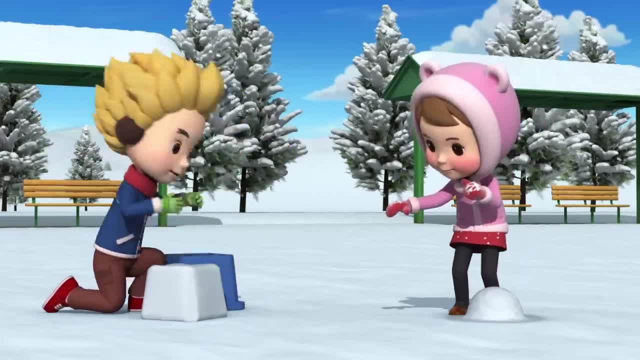 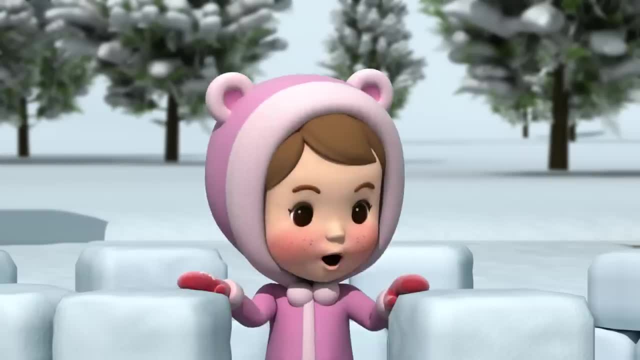 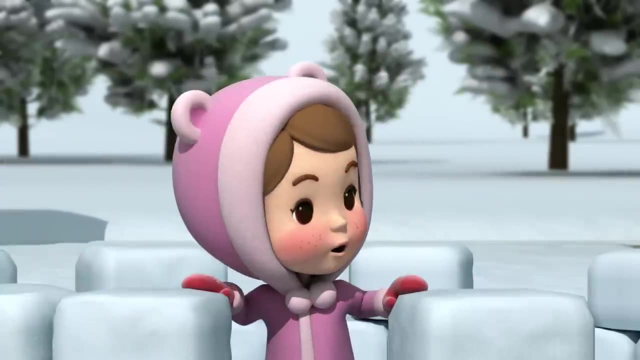 Oh Cool, What is it? I'm making a snow castle. You are There All done? Oh wow, It's awesome. It looks just like a castle made for a princess. Now, Now, what That looks fun. 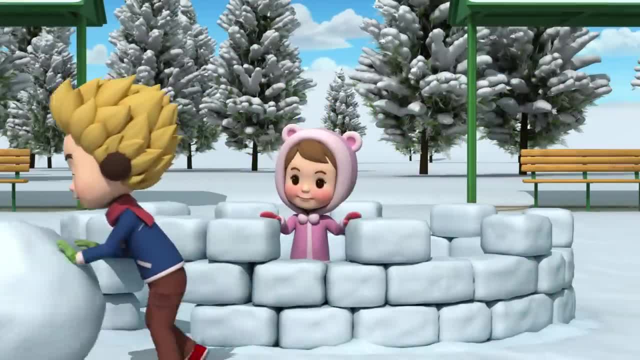 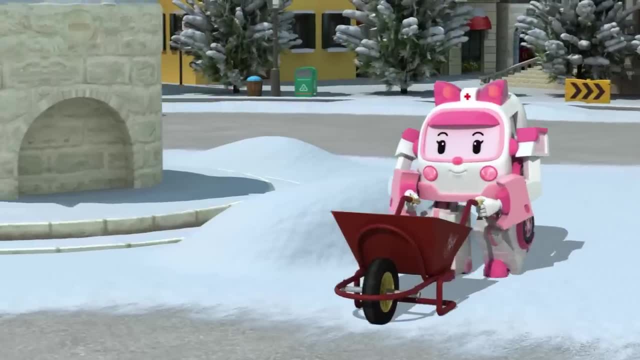 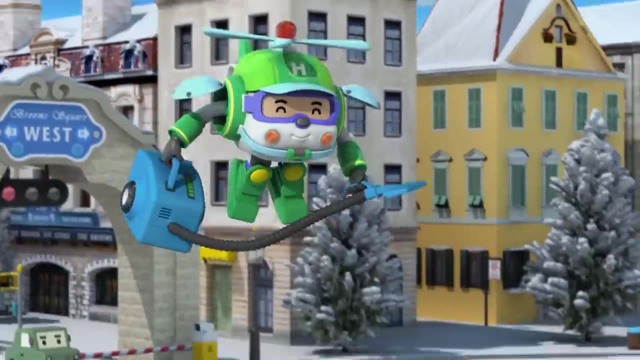 My next job is making a big snowman. Wow, I'll help Wait for me. Hi everyone, Huh, Hey, look at what I brought. Look, Whoa, Oh, Oh, Are you OK, Holly? Are you OK, Holly? 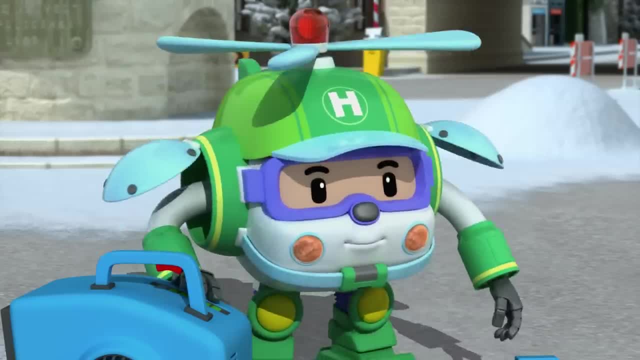 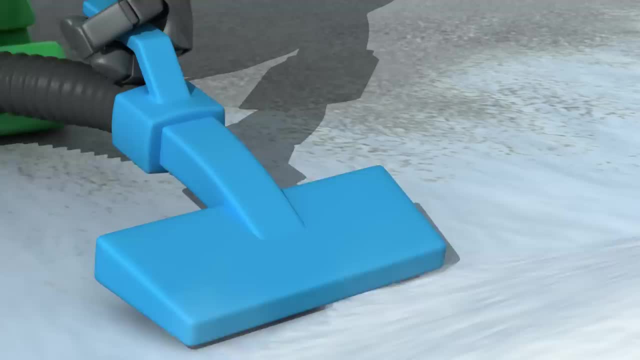 It's slippery, You've got to be extra careful. I wanted you all to see this. It's a new invention of Jin's. It's a snow cleaner. A snow cleaner. Yeah, Isn't it the coolest. It sucks up the snow and it works great. 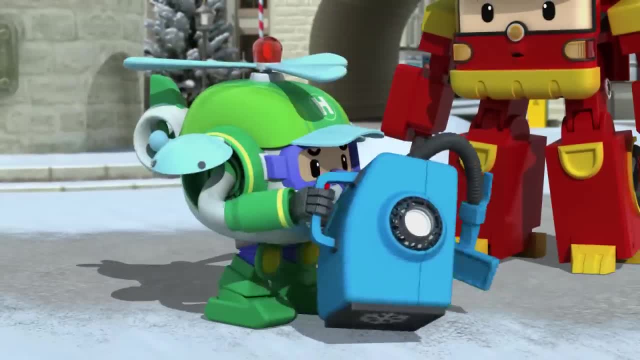 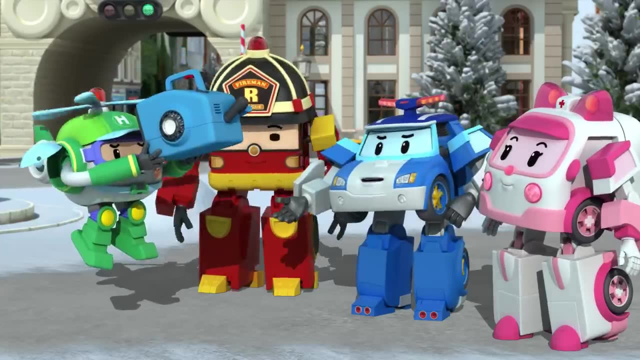 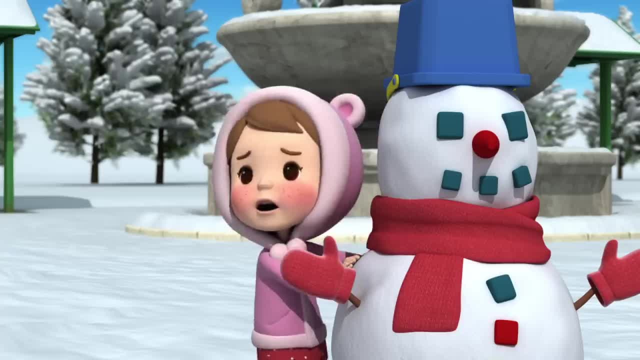 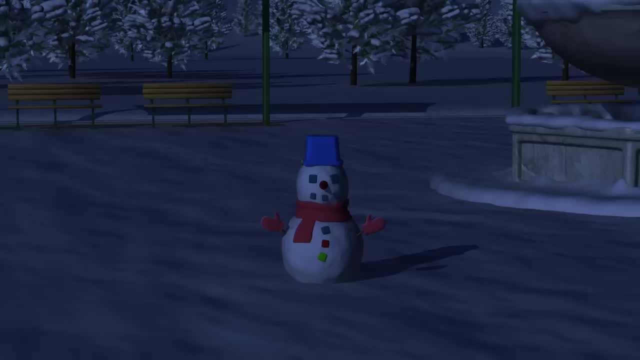 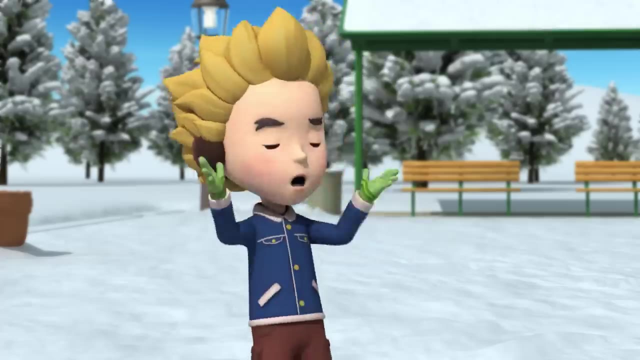 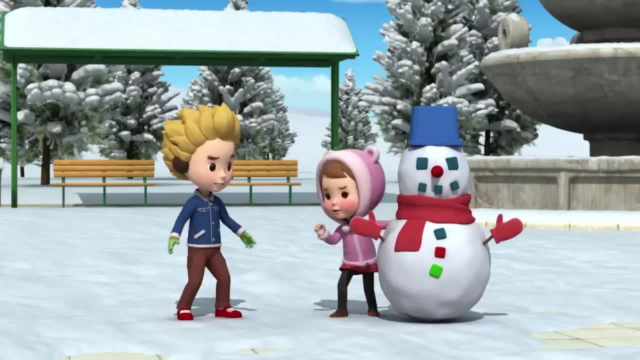 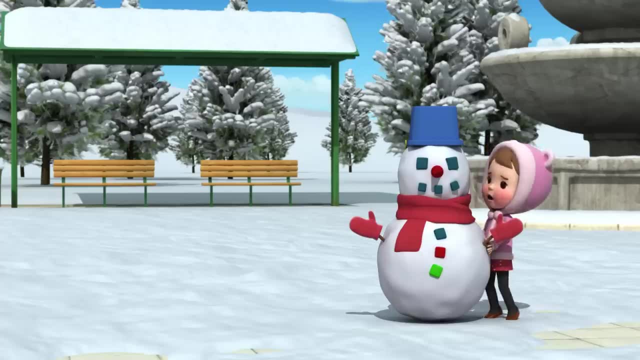 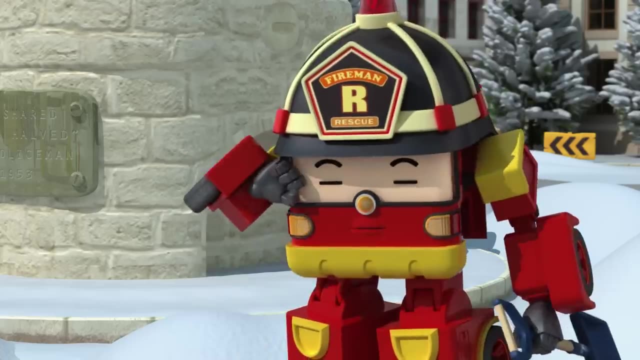 What? How are you going to carry a snowman? Then you just go home by yourself and I'll stay here with my friend. Fine, Do what you want, Bye My snowman. I think that should be just fine, Right? So now let's go and take care of the park. 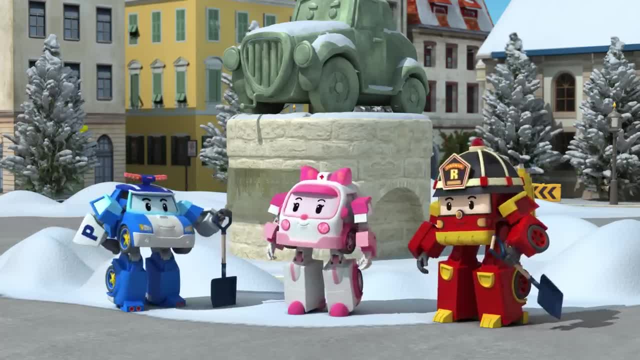 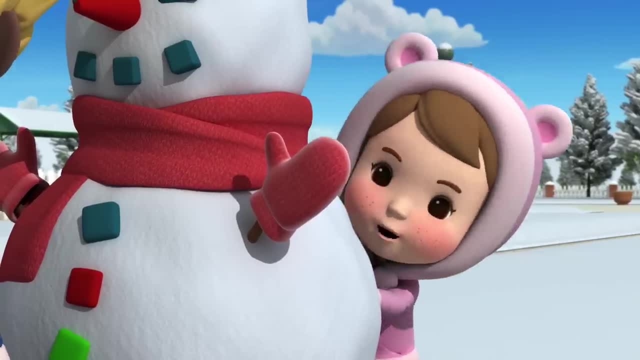 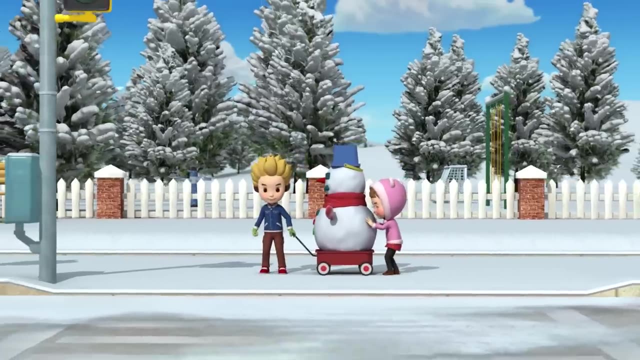 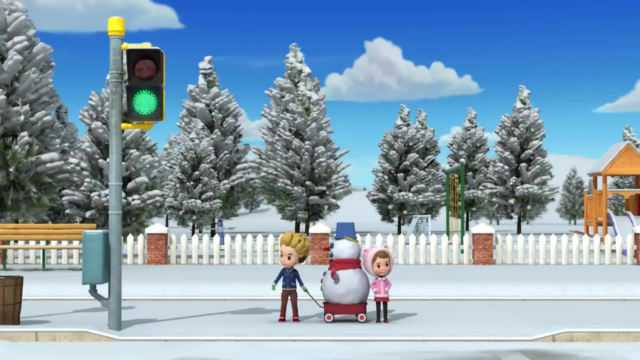 Good. Next stop the park, Right. I can't wait. Now our snowman will be safe in our house. Susie, he's going to melt if we bring him indoors. Really, It's so cold Time to cross. 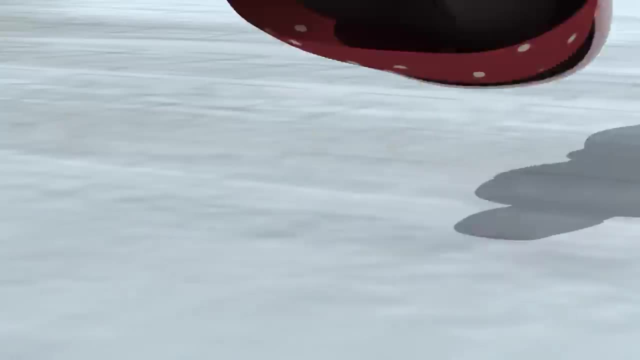 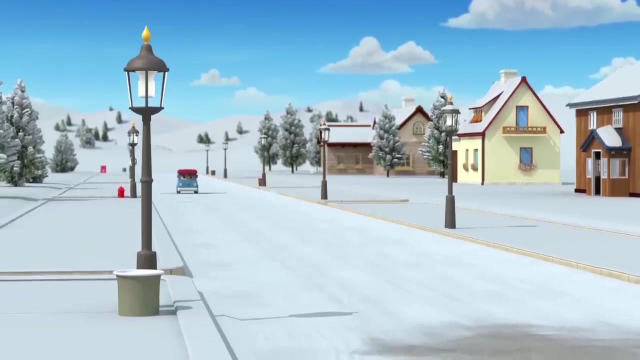 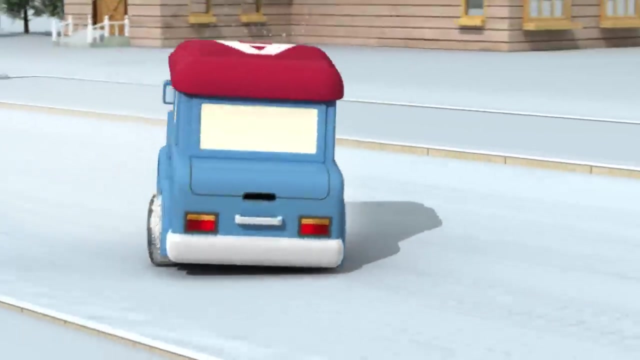 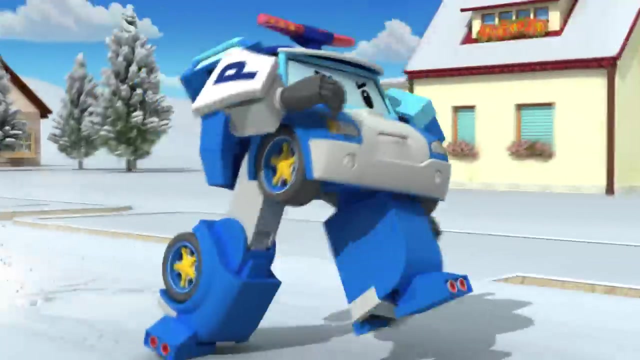 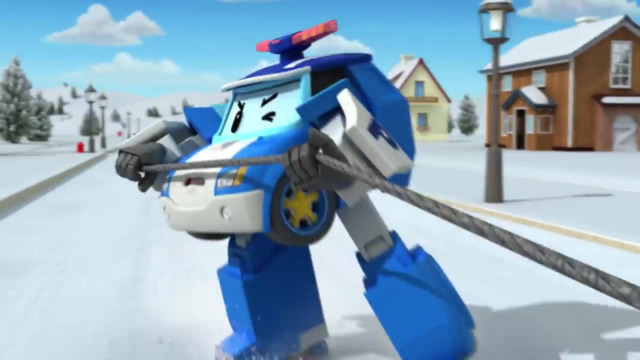 Okay, Here he comes. No, Susie, Are you okay? It hurts. Hey, A red light. Uh-oh, Whoa, I'm starting to skid. I can't stop Look out. Huh, Huh, Huh. 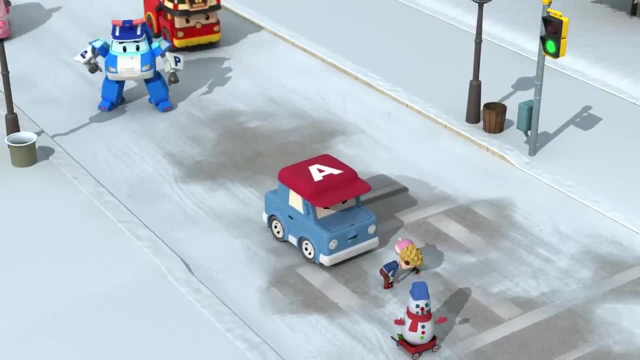 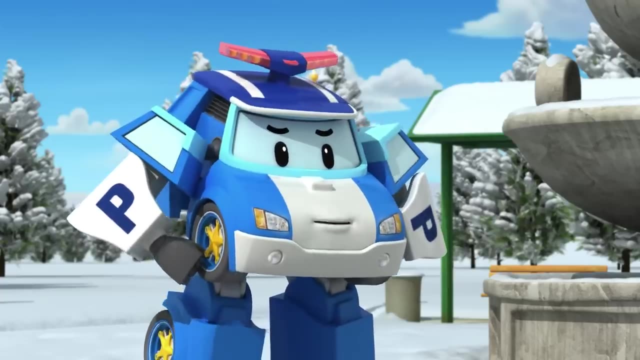 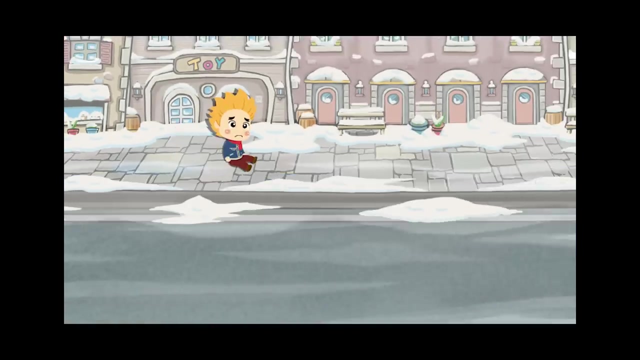 Holy, Thank goodness. Well, I'm so glad everyone's okay. But that certainly was a close call, Kevin Susie. when it snows, roads are very slippery, Cars and people can easily get into accidents. Cars can't stop quickly on snowy roads. 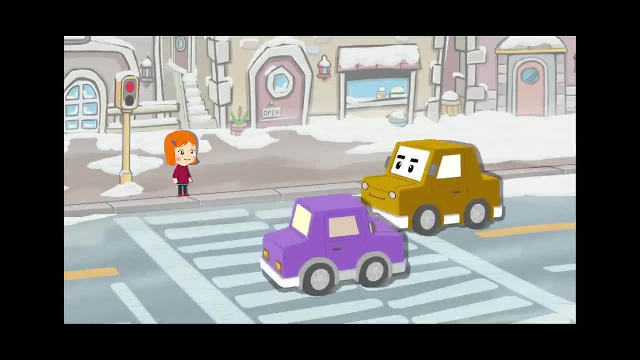 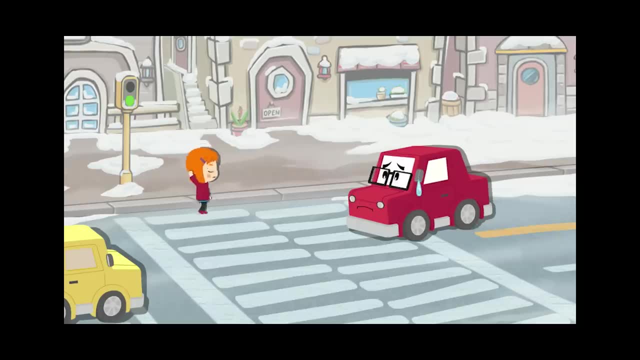 So you have to make sure to be extra careful when crossing on foot. You should either wait first for any cars to pass or make sure they've made a complete stop before attempting to cross the street, And if you walk with your hands in your pockets, that can be dangerous too. 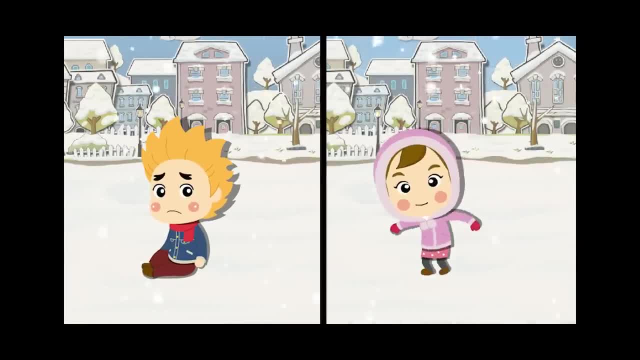 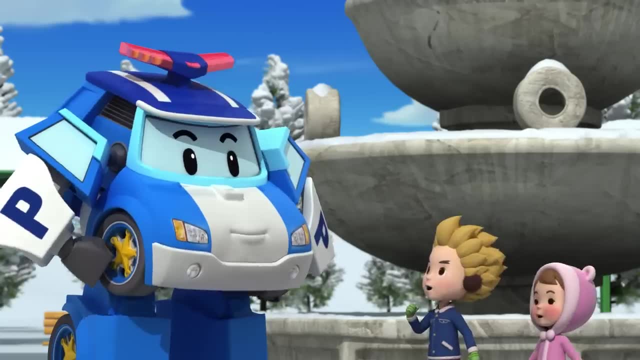 It's always a good idea to wear gloves. You should also avoid wearing white clothes. on a snowy day, You'll be seen more easily wearing colorful clothes. We'll do that, Polly. Hey guys, Huh, Now watch this. 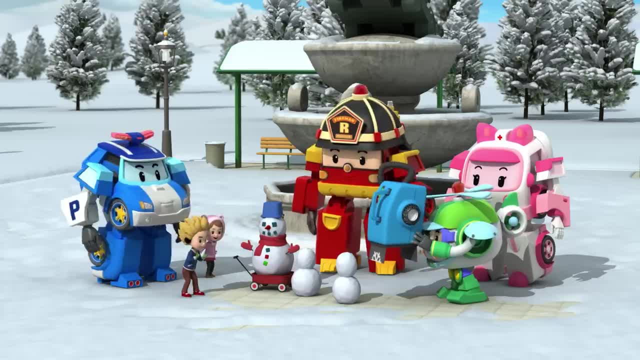 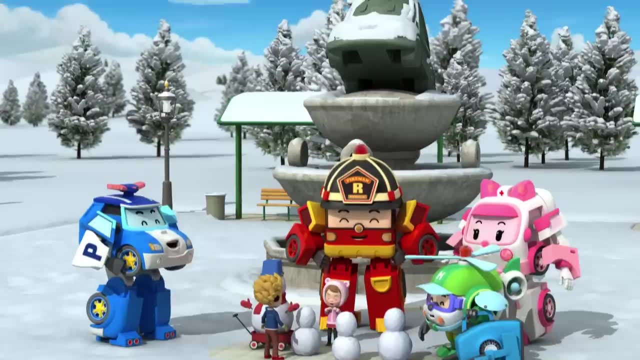 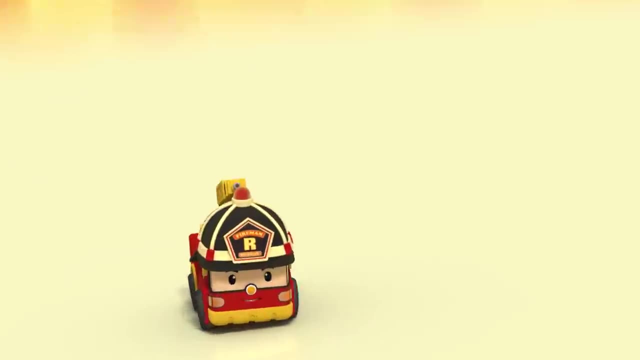 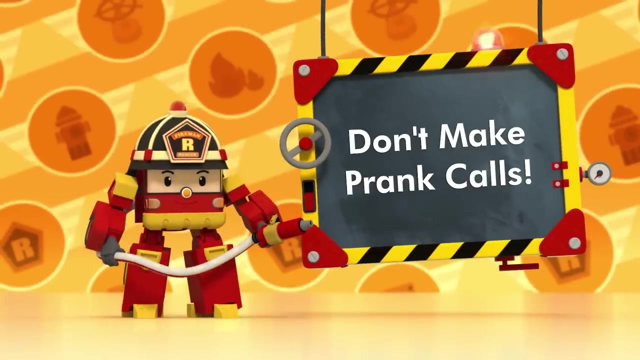 Whoa, More snowmen, More snowmen. Now our snowman's going to have lots and lots of friends. Your snowman won't have any time to be lonely ever again. Bye kids, Hope your school day's great. Oh Schoolby Huh. 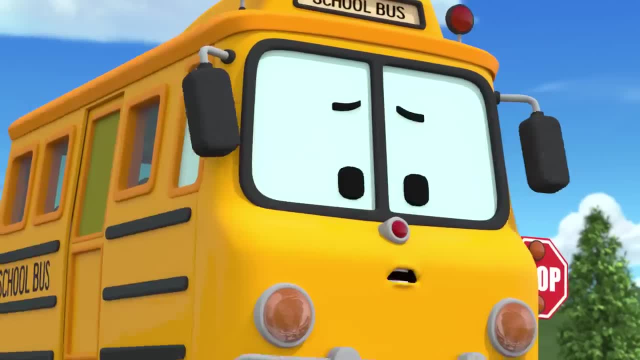 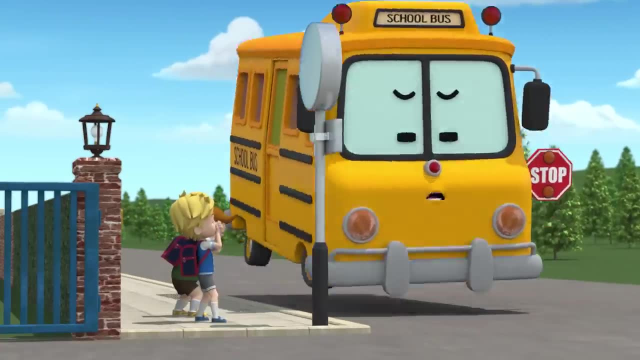 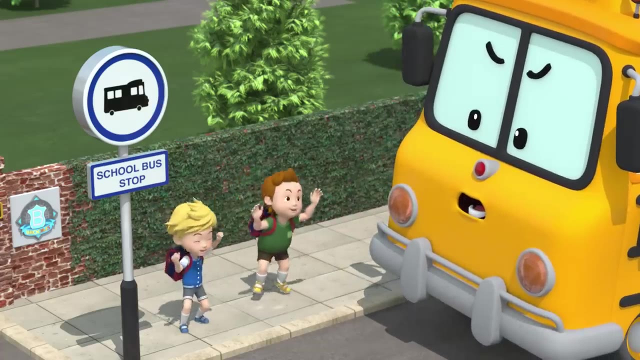 Yes, What's that on your bumper? That's bird poop, right, What? No way, Where? Oh, that's gross Schoolby. you should go through a car wash. Someone get it off. April Fools, April Fools. 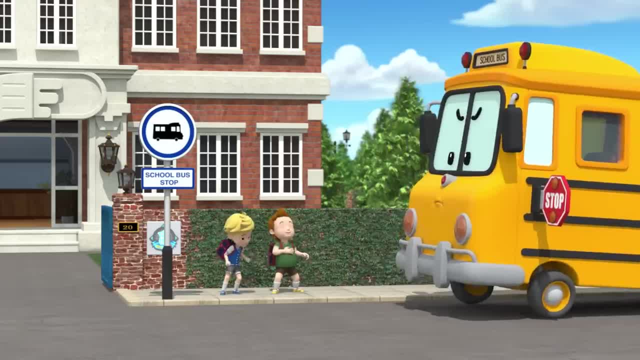 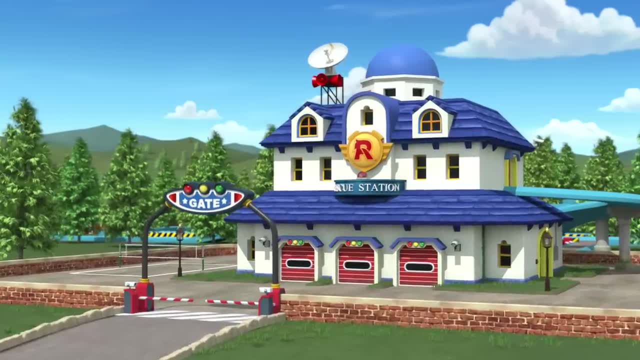 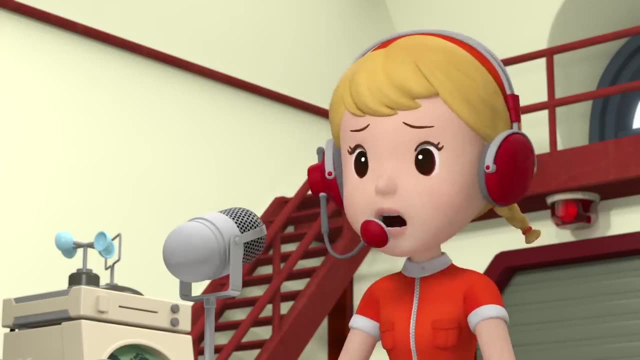 Silly. The bird poop wasn't real. Watch out for bird poop, Schoolby. We need help. Minnie shrank herself. Huh, What do you mean shrank? Help me, I'm tiny Minnie, how is that possible? 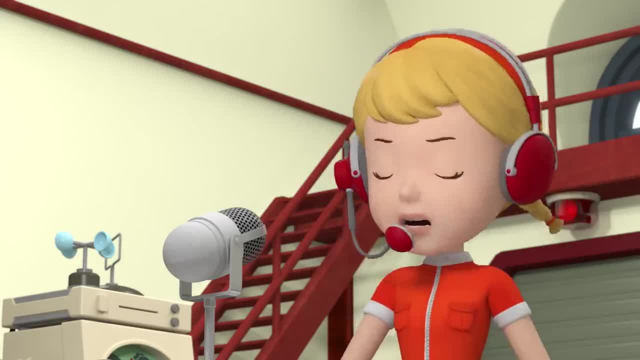 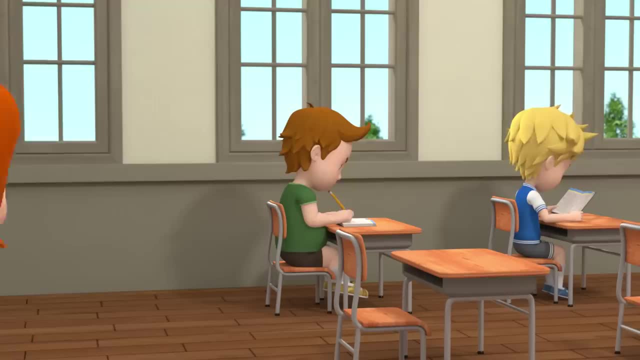 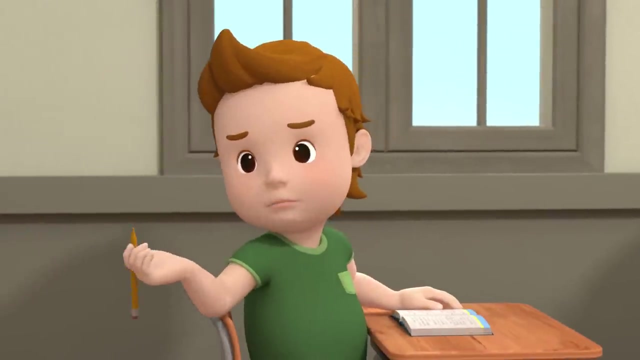 I got you real good Today's April Fools. What That's today? Here she comes. Shhh, Huh, You guys are studying. That's unusual. Yeah, it's for the test. Yeah, that huge exam today. 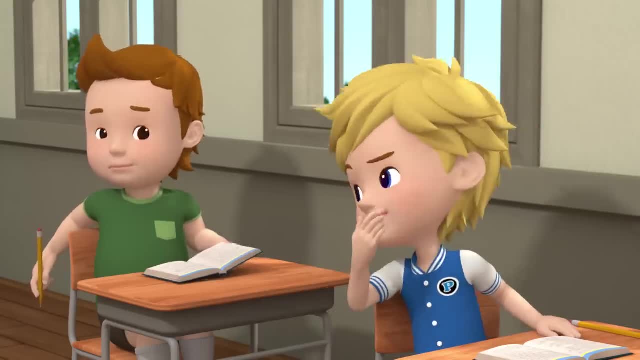 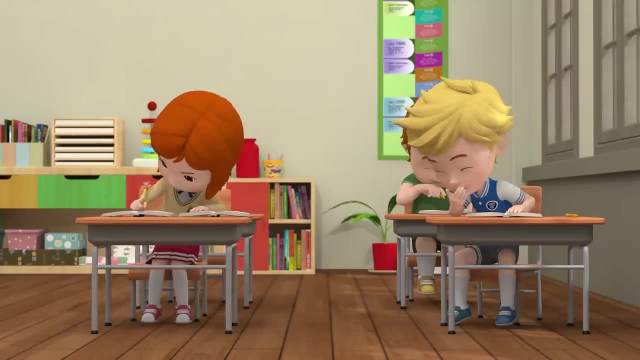 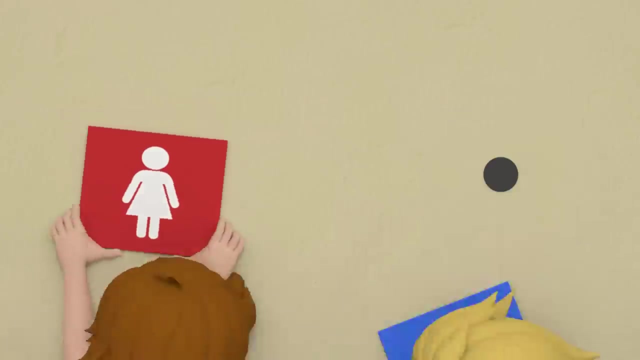 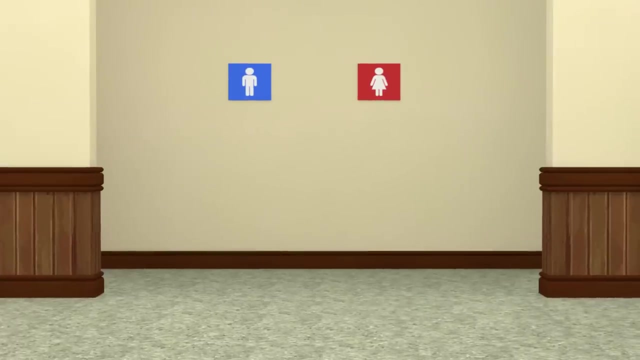 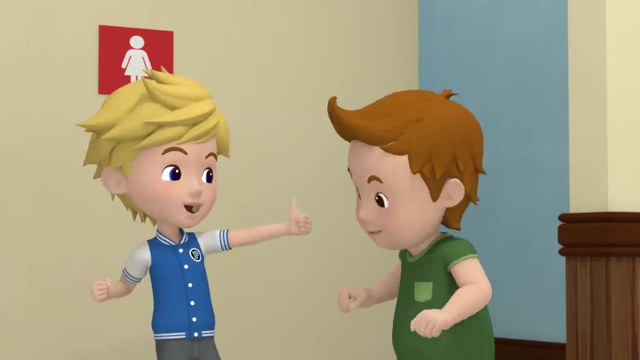 What Exam? Don't tell me you forgot about it, Right, Johnny? Ah, I never forget. Oh sorry, I thought this was Ugh Oof. Hahaha, That was the best one yet, Hahaha. 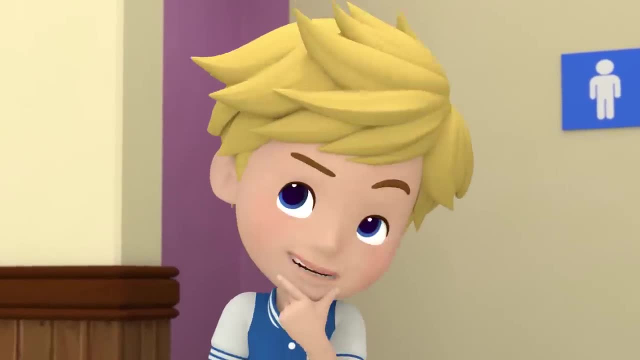 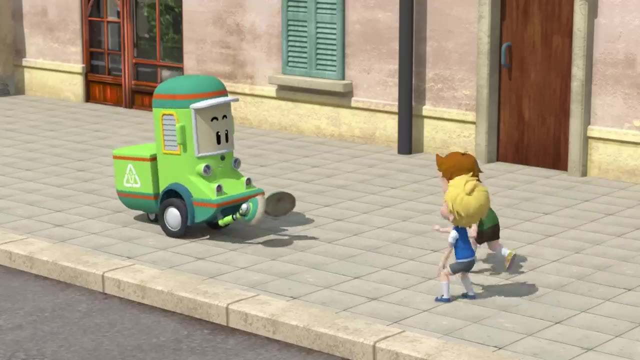 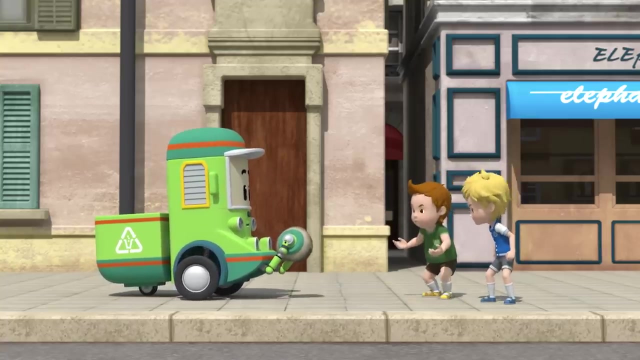 So who's the next person we should prank? I have an idea: Heh Cleenie, Hi guys, What's up? Someone tipped over all the trash cans in town. What Now? trash is flying all over the place. No, 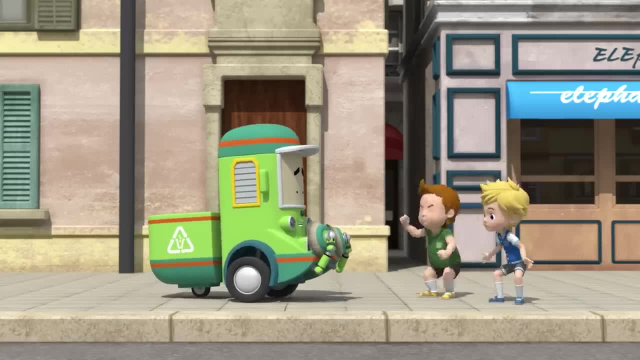 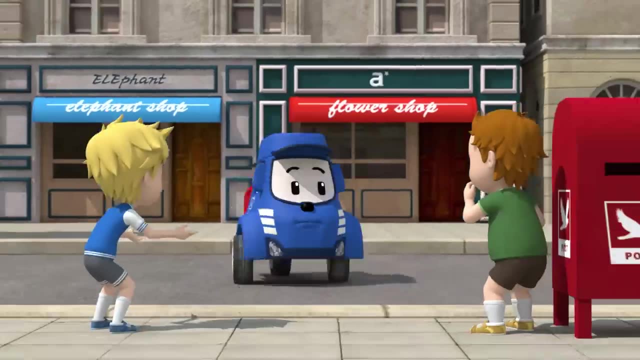 That's not all. Somebody ran over it, and now it's gotten even worse. I can't stand it. I'll fix it. Hahaha Ha, Destroyed the post office. Mm-hmm, Really, Tires as high as a mountain. 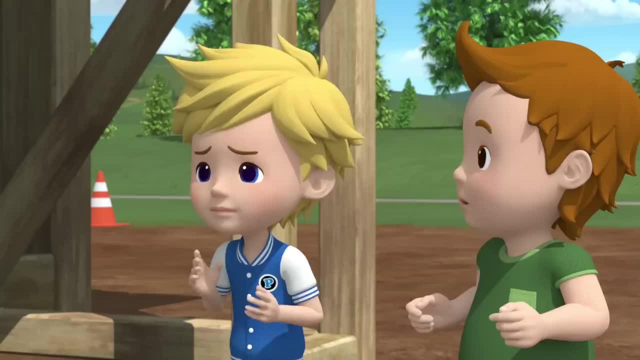 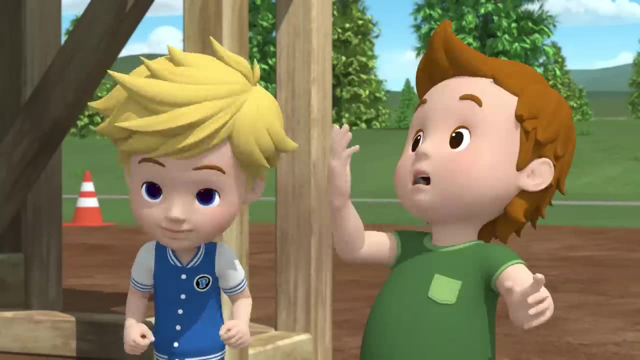 Mm-hmm- Seriously Free toys at the toy store. Mm-hmm Max was just walking and then something happened. Yeah, he fell off a tree and, uh, hit his head. Huh, How'd he climb a tree with tires? 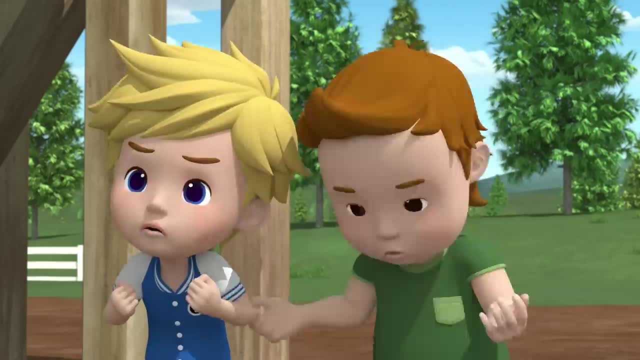 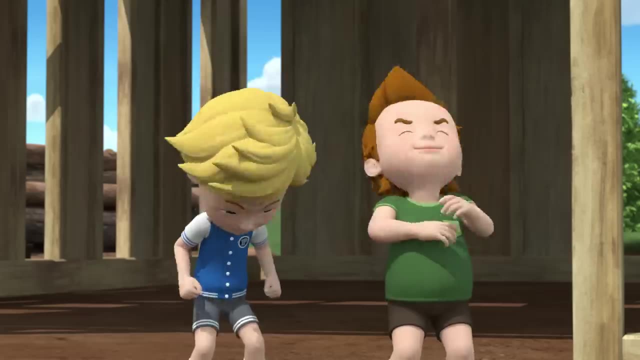 I mean, I mean he Drove off the road into the mud, Drove off the road into the mud. You mean again Mm-hmm. Oh man, Third time this month. Hurry, We're awesome. 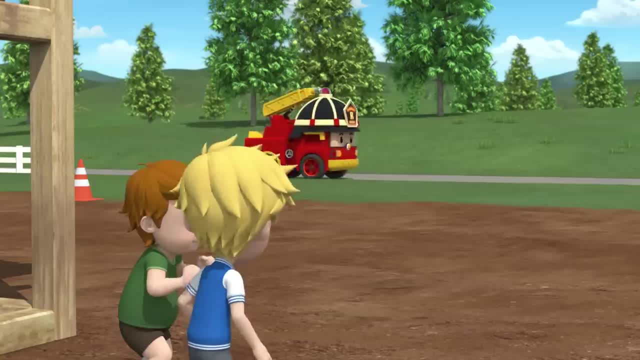 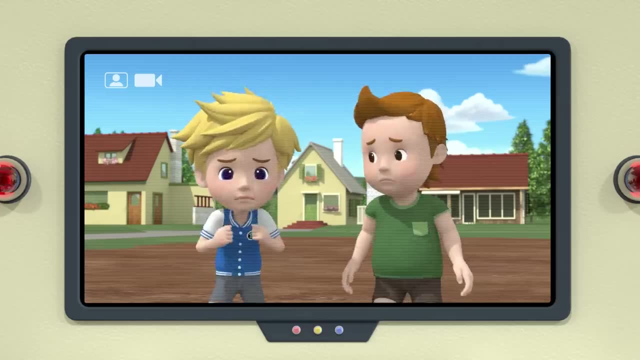 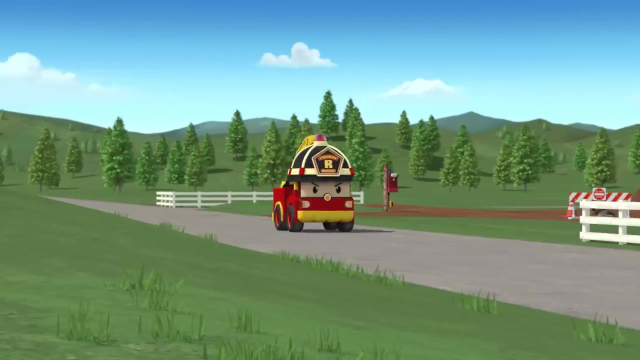 I think we pranked everyone in town. Huh, Hmm, Man too good A fire at the harbor. Yeah, It's all over the place. now You gotta do something. We're on it guys, Roy. Hahaha. 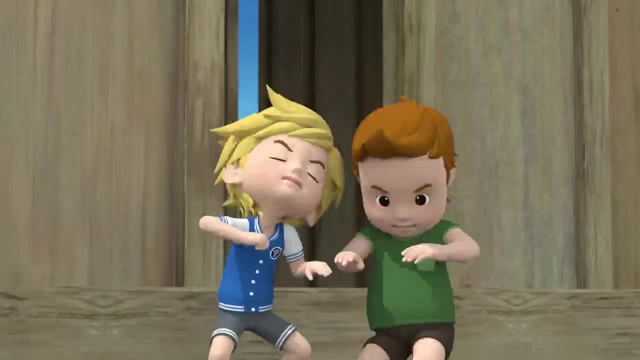 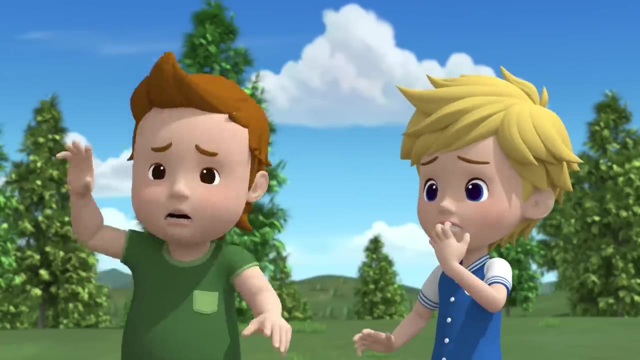 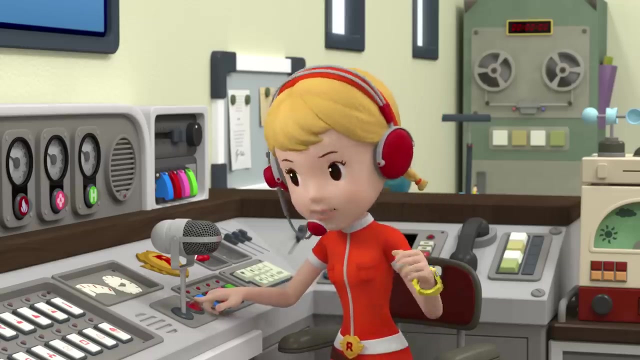 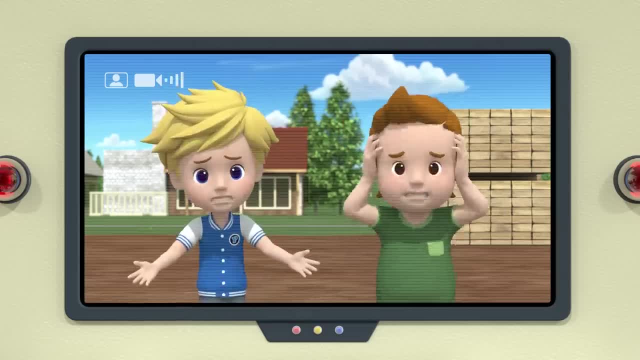 Johnny, This is a real one. This is bad. Oh geez, It's Jen. How can I help? We need help Here at the factory. A fire? Huh, Didn't you say the fire was at the harbor? 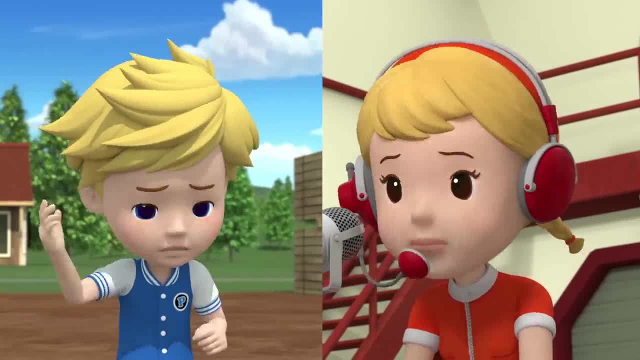 Uh, you see, that was a lie. What, Peter? don't you know how dangerous that could be? I'm sorry, but this one's real this time. I'm sorry, but this one's real this time, Oh, Oh. 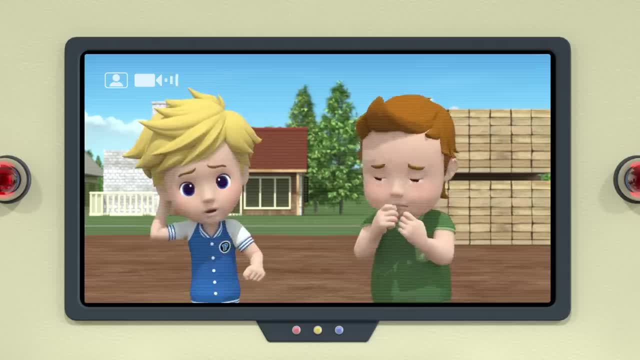 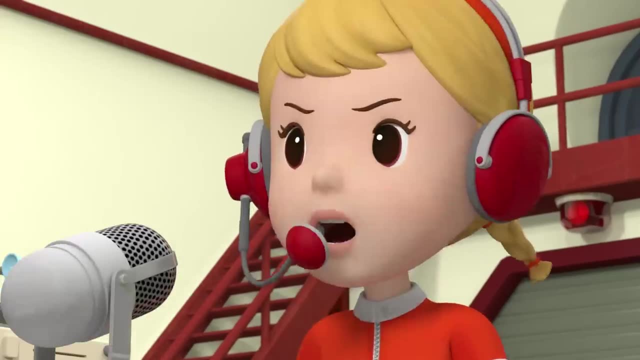 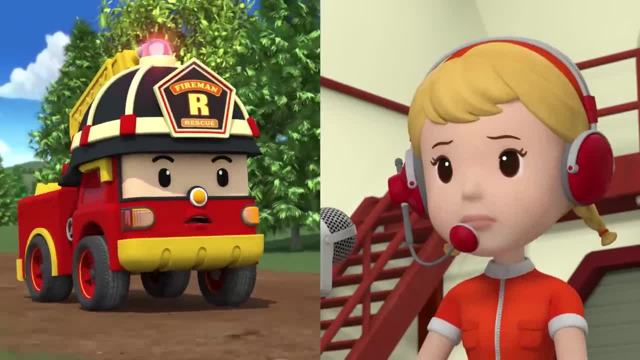 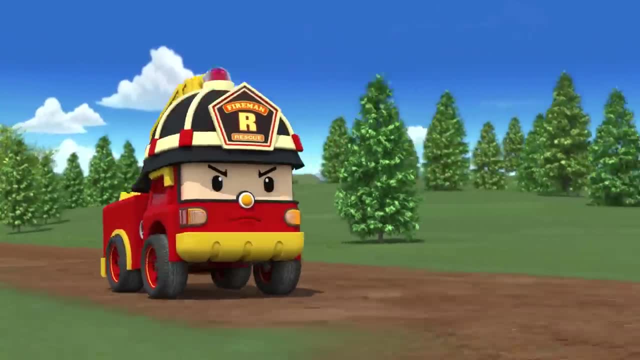 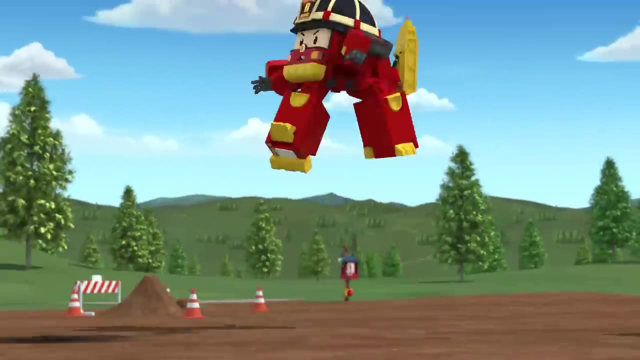 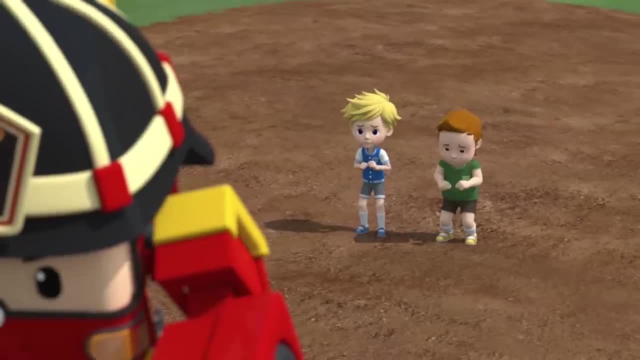 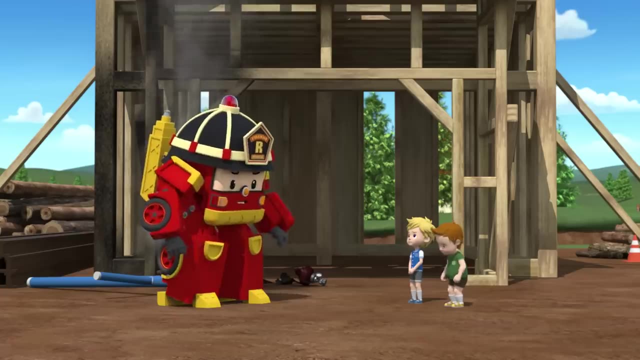 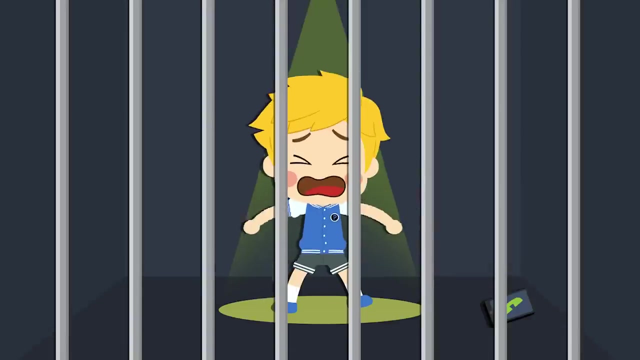 Wow, I'm real sorry about our prank Roy. We feel really bad. Kids. prank calls are mean at best and dangerous at worst. Prank calls aren't just illegal. If you prank call about a fire, firefighters will assemble where they're not needed. 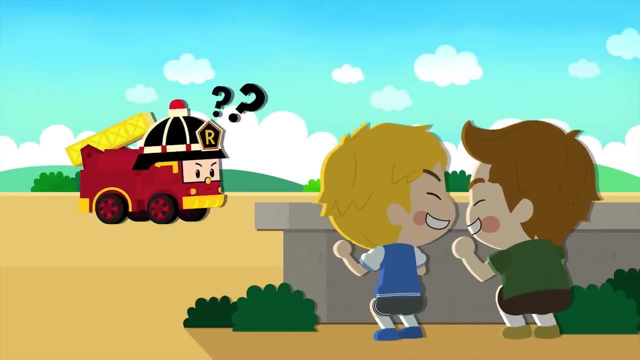 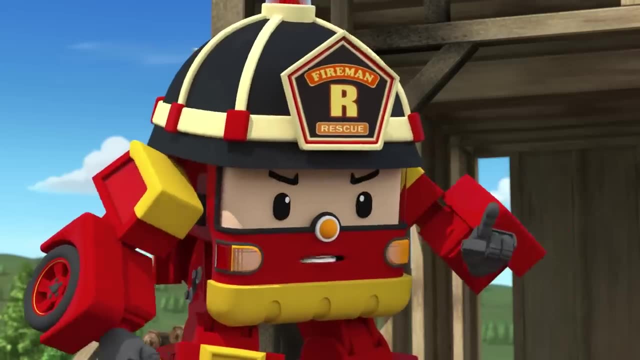 The problem with that is, if there's a real fire, then they can't get to the real fire in time And it could cause serious damage. One prank call can put someone's life in danger. Must have been why Jin was so mad. 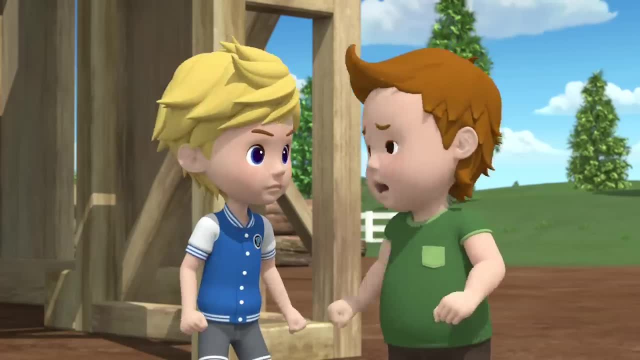 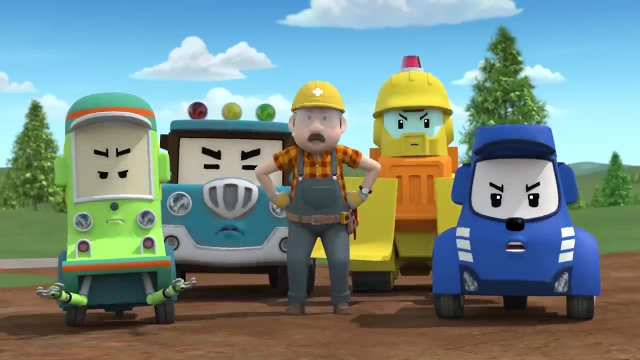 We won't prank call anyone ever again. Also, we won't lie about stuff. Yeah, Peter, Johnny, you've got some explaining to do. Yeah, Why'd you prank us? Huh, We're doomed. Huh, What's that? 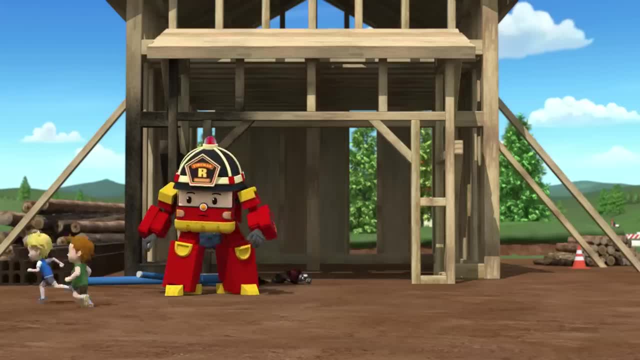 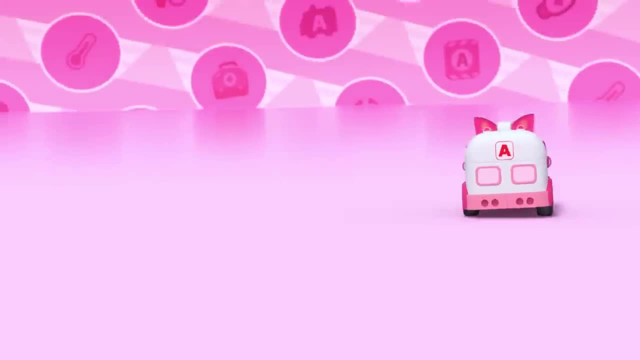 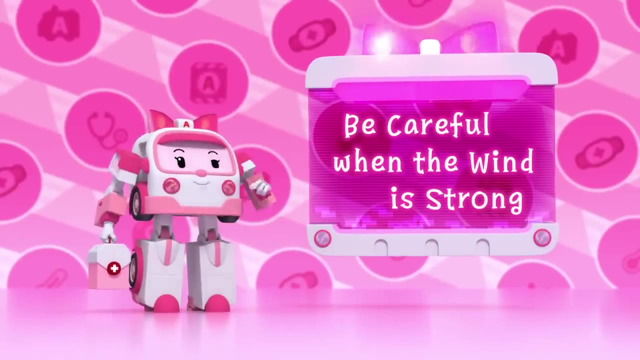 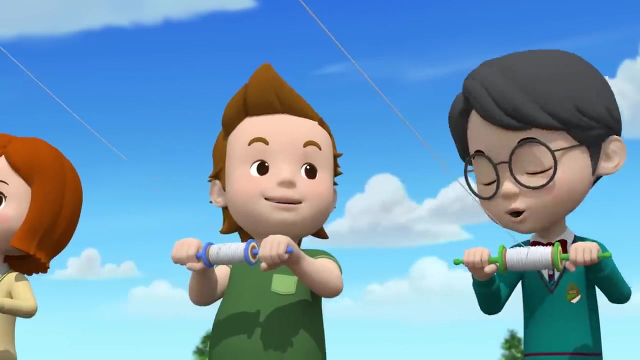 Huh, Why us? Sorry, Get back here, you pranksters. Ha ha, ha, ha ha ha. Be careful when the wind is strong. Wow, This hill is the best for kite flying. Wow, Johnny, How do you get your kite so high? 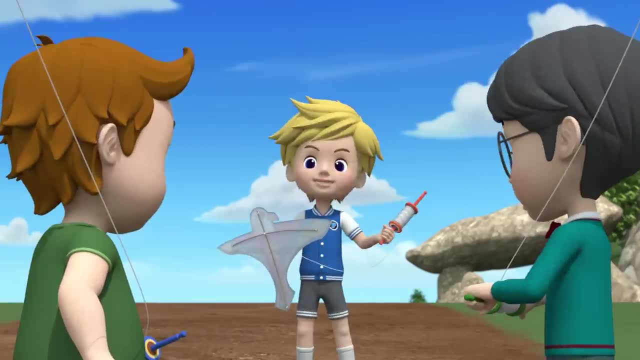 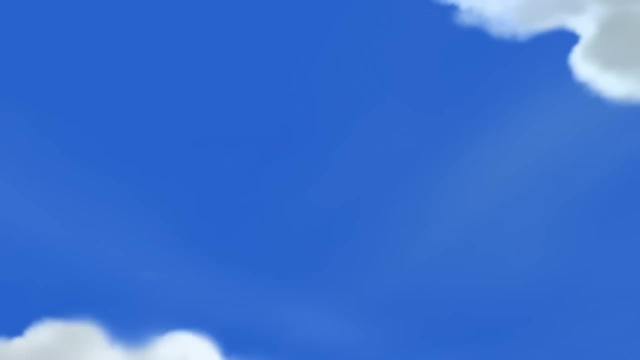 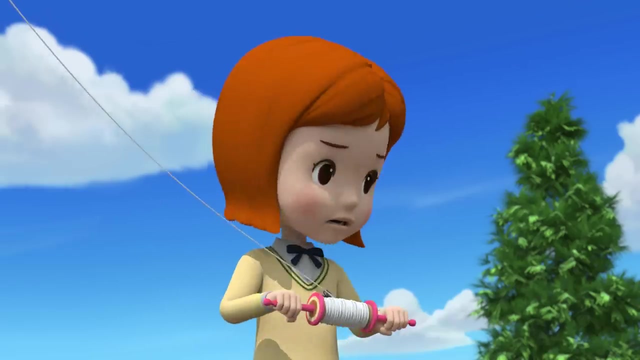 My secret: Are you flying your little kites? Well, take a look. No kite can outfly my eagle. Ya-ya Huh, Whoa, Ha, ha ha, The eagle's the king. Uh, Peter, your kite looks a little strange. 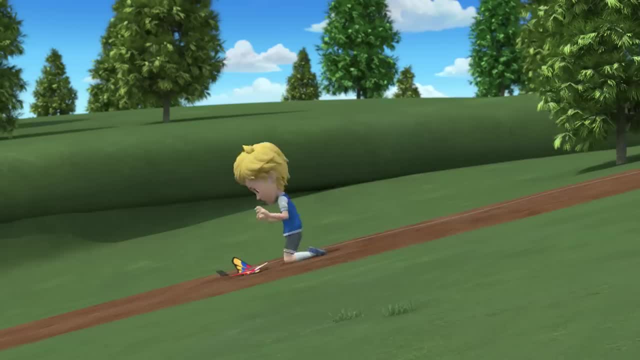 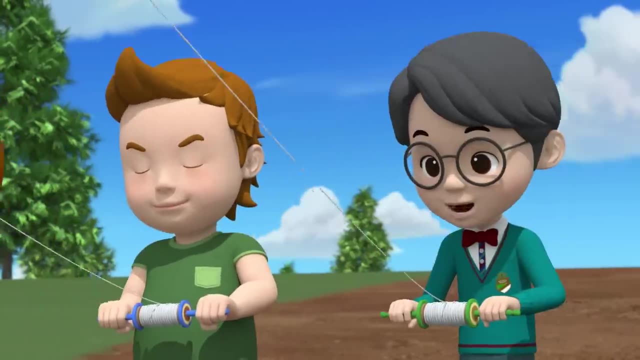 Huh, Whoa. No, The eagle has fallen. Peter, kites can't be just any cool shape. Yeah, Peter, If a kite isn't balanced, it's hard to fly. Peter, Do you need my help to make a kite that flies? 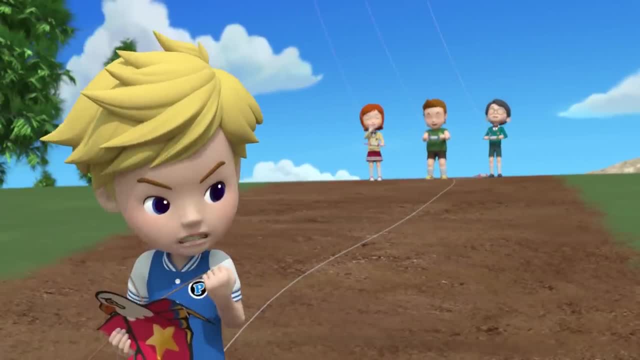 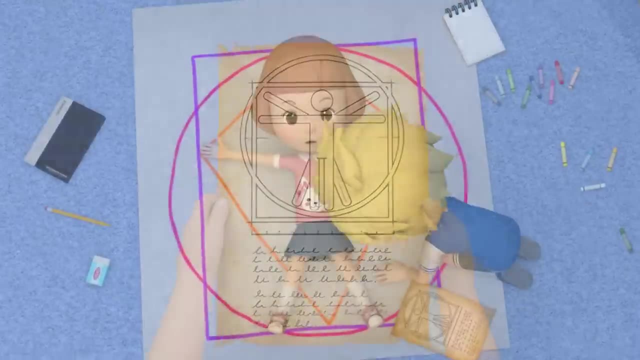 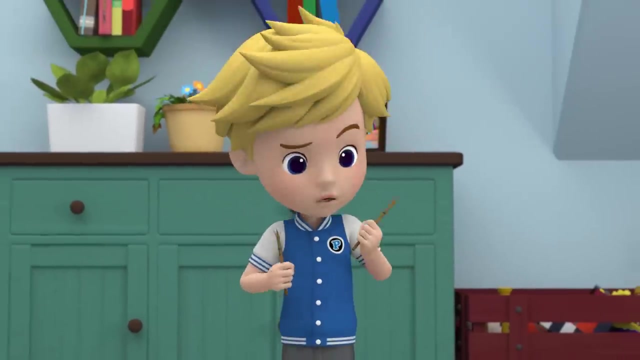 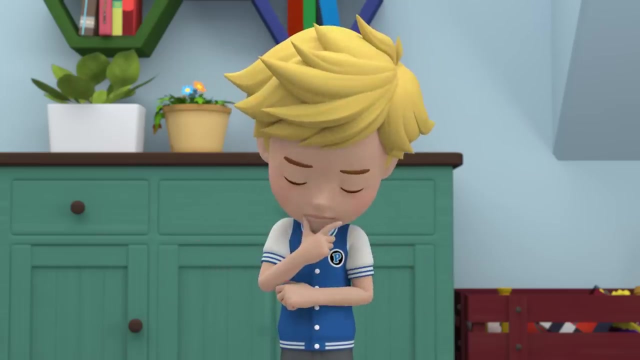 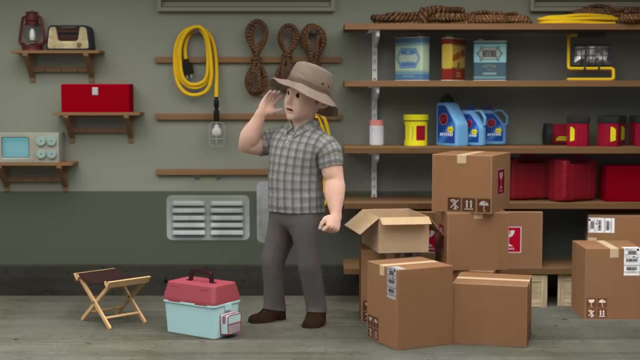 Ha, ha ha ha. Stop laughing, You'll see, This one is wrong. What's as strong as rock but as flexible as a bow? Ah-ha, I've got it. Huh, where could it be, Honey? you see my fishing rod. 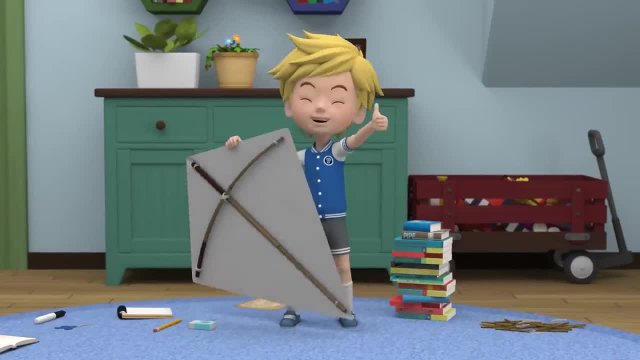 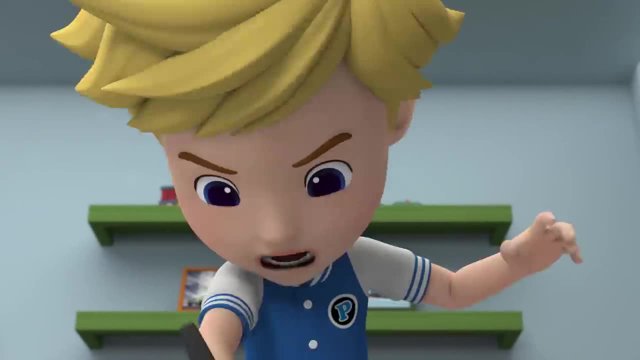 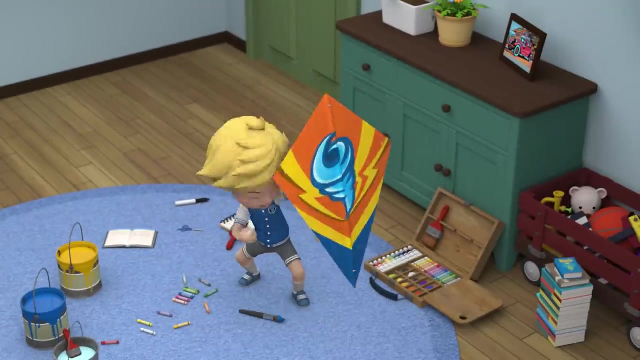 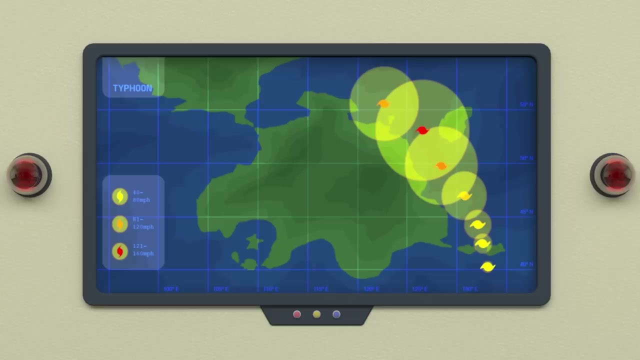 That's right. the fishing rod works great. My masterpiece is done. Superstorm Guys, we have a problem. A big typhoon from the southeast is headed for Broopstown. We need to make extra sure the town's prepared. All right, Jin. 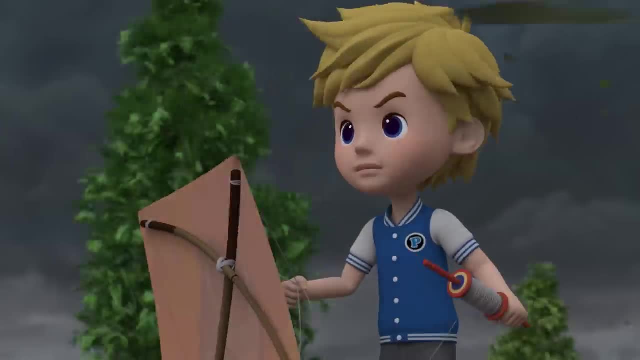 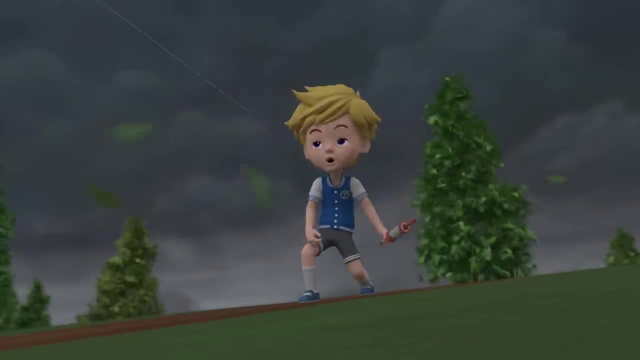 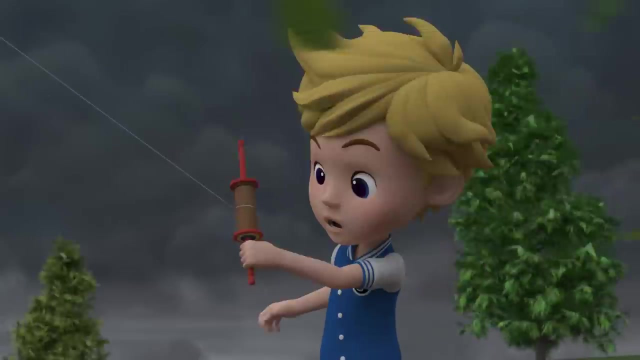 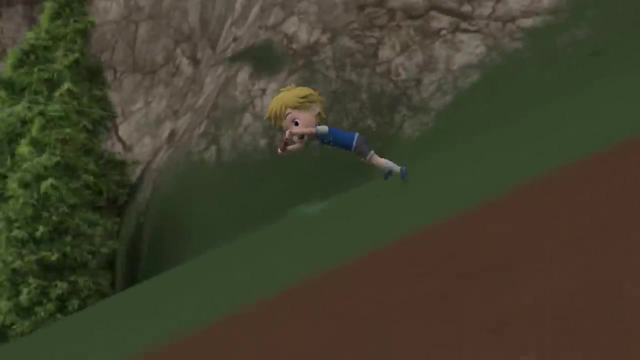 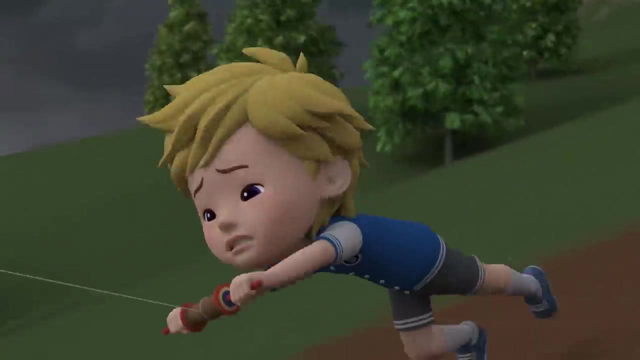 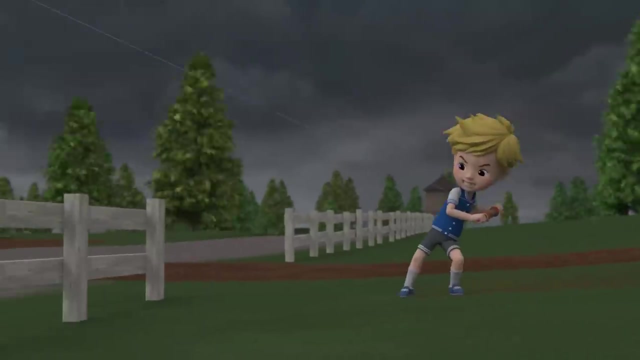 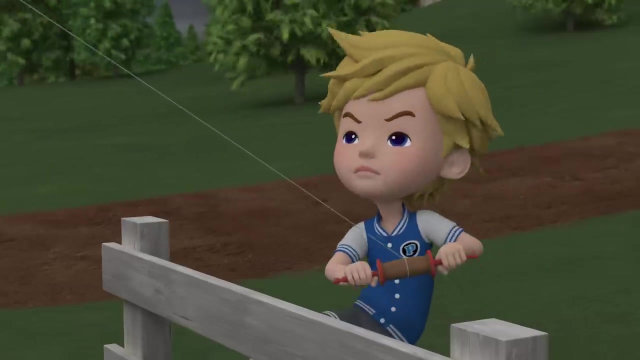 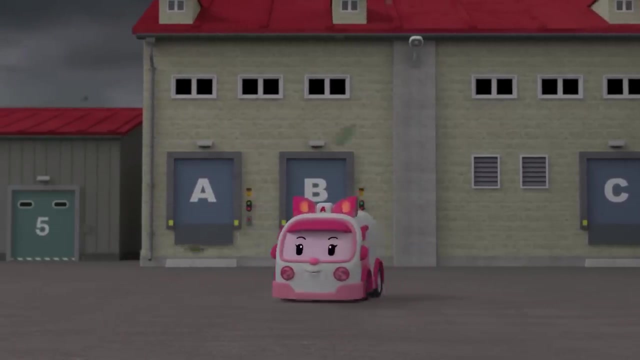 The weather's absolutely perfect. Best ever, first flight- Fly Superstorm. Oh, I did it. Best kite ever. Ha, ha, ha, No Help. Ah, Superstorm, We've checked the whole port. I'm heading back to town now. 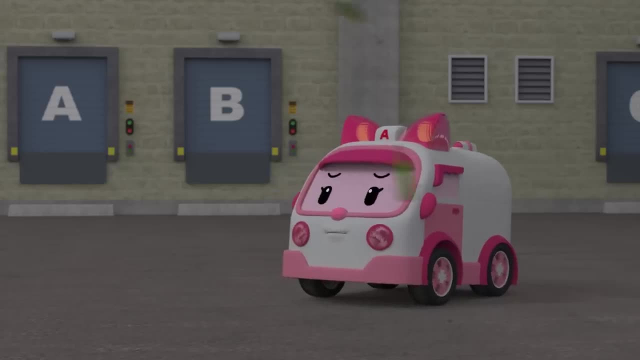 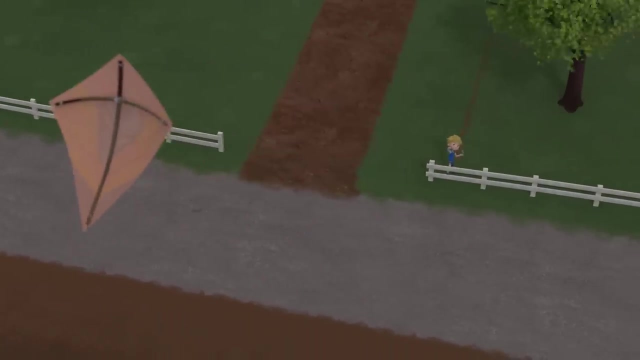 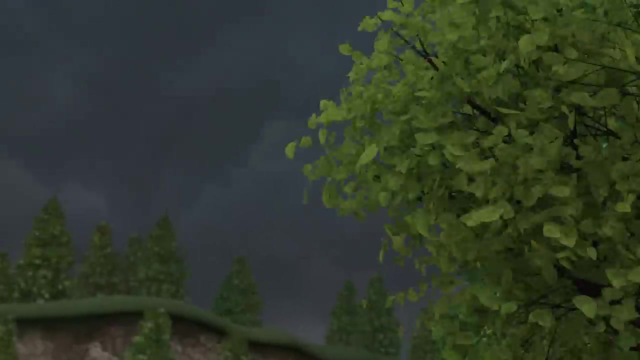 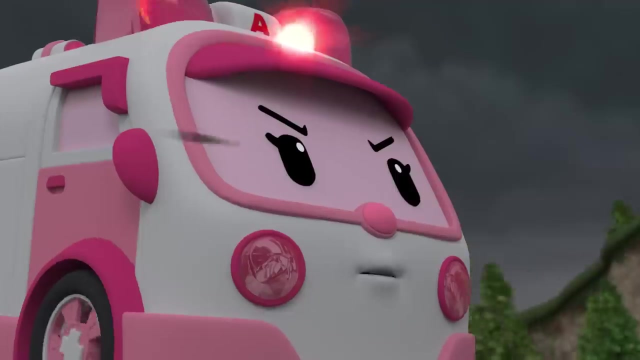 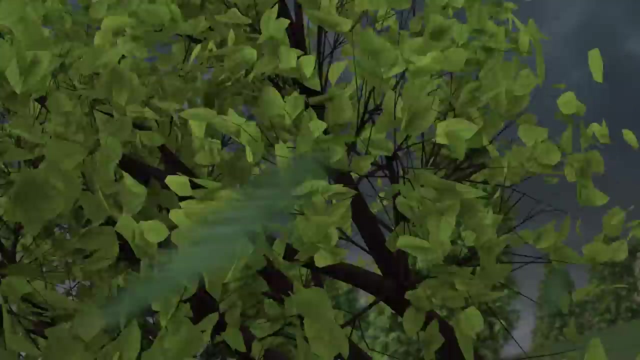 Huh, Is that a kite? Who's flying a kite in this weather? Huh, Little bit more, Little bit more. Gotcha. Look out, Gotcha, Gotcha. Are you all right? Yes, I think I'm all right. 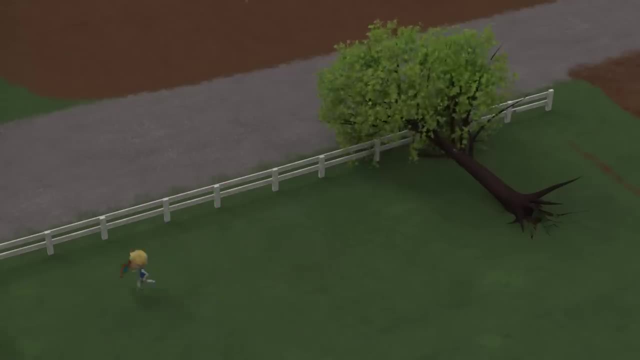 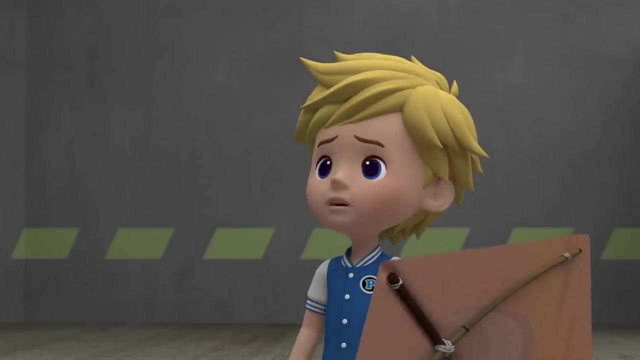 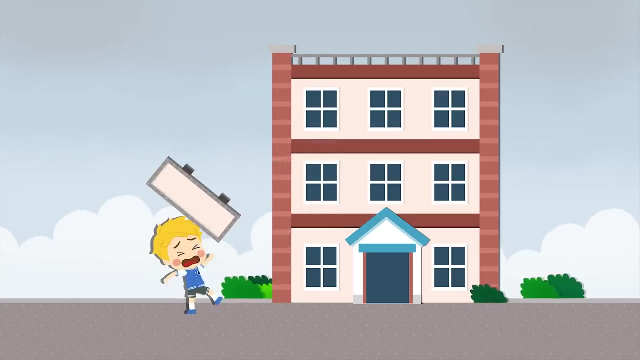 Let's move to a safe place. Yeah, Peter, goodness, that was a very close call, But I can't thank you enough. Listen up, It's dangerous To go out, to go outside. in strong winds, Signs can drop or trees may fall down. 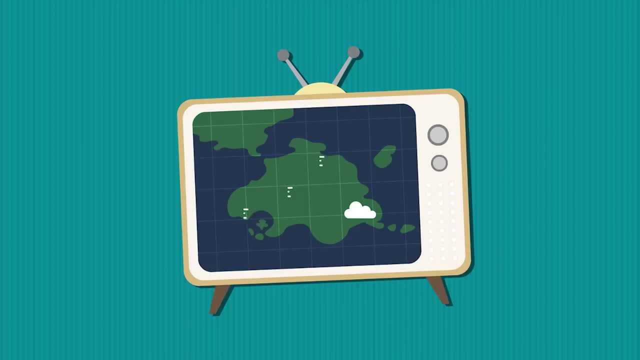 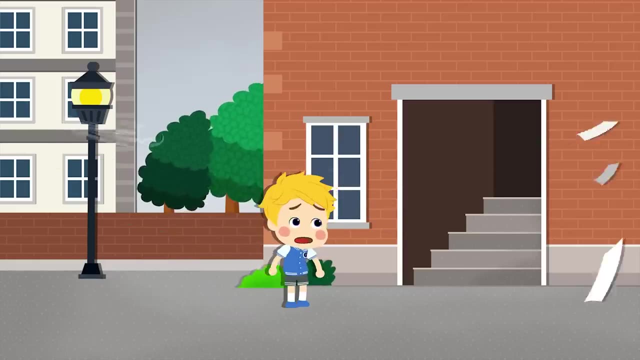 And you can get hurt by all kinds of flying stuff. So on a day with a strong wind warning, please don't go outside. If you are outside and a strong wind starts, you should take shelter in a safe building. Also, there's a danger of electric shocks. 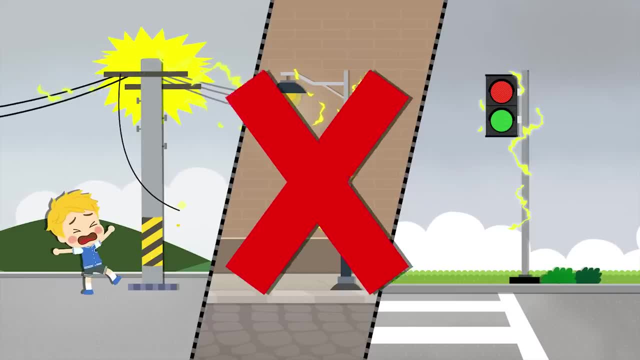 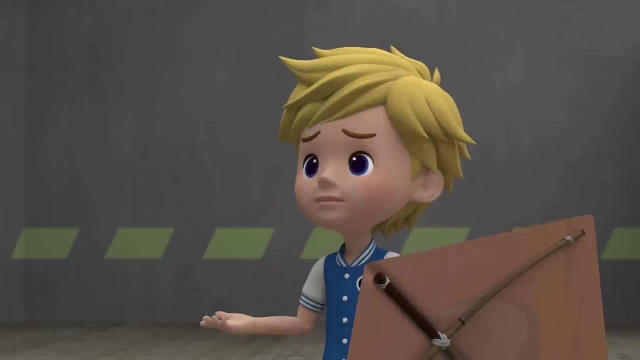 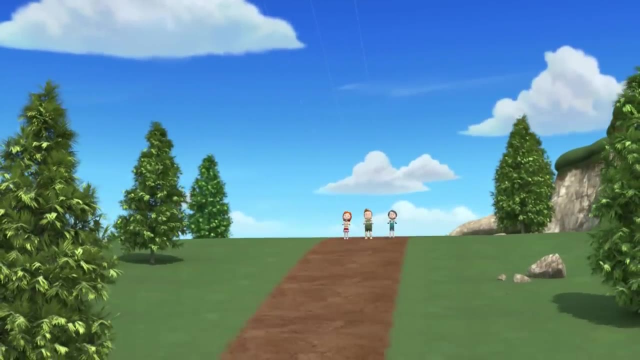 from electric poles, street lights or traffic lights. Avoid touching them. All right, Peter? Yeah, I promise. I promise not to go outside whenever there's a strong wind. Very good, Wow, Looks like Johnny's got the highest kite again. 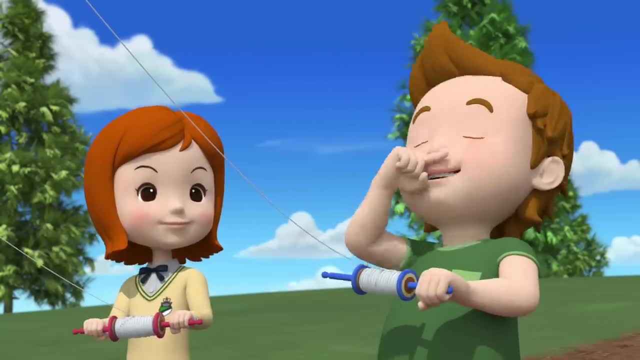 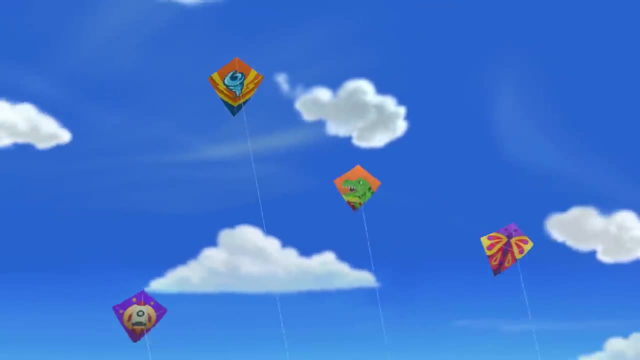 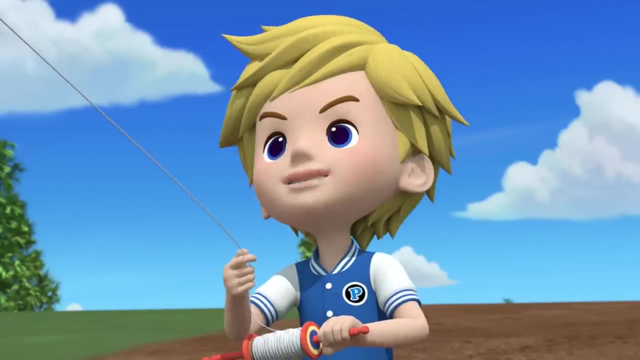 Johnny, what's your big secret? Well, the secret is It's called Superstorm. Yeah, Wow, Peter, Your kite flies crazy high. Looks like it's perfectly balanced. Superstorm has no rudder. Superstorm has no rudder. 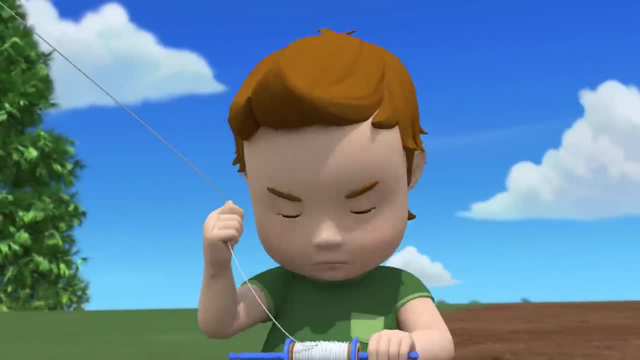 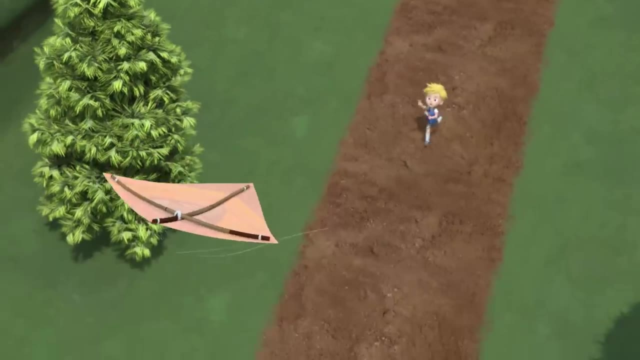 And it's a rival. It survived in the strongest winds. Um, yeah, it's all right. Ah, No, My Superstorm. Aww, Ha ha ha, JET AND JETTLE, JETTLE, JETTLE. 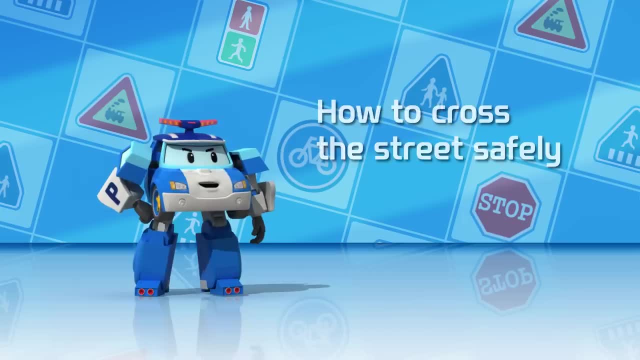 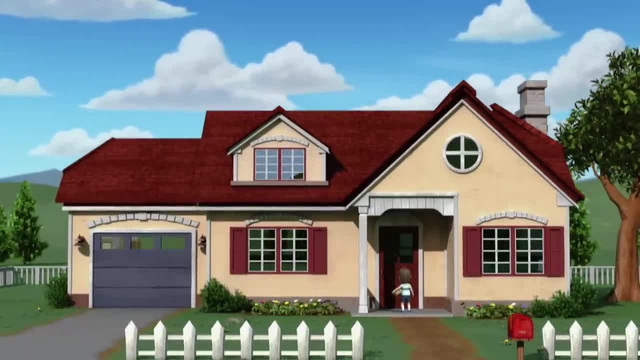 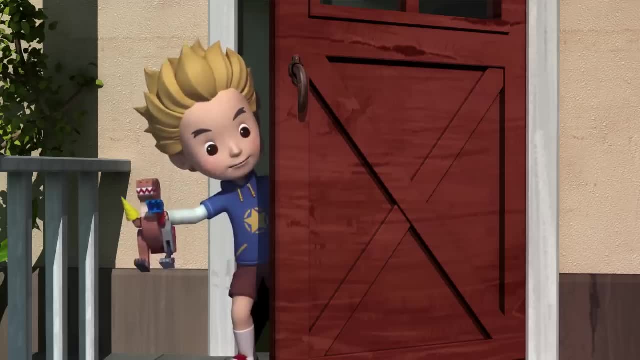 JETTLE, JETTLE, Kevin, Kevin, we're late. Hurry up, Hurry up, Roar. Whoa, Whoa. Hey, Doug, I made Jenny this dinosaur myself. Well, she's not going to like it. 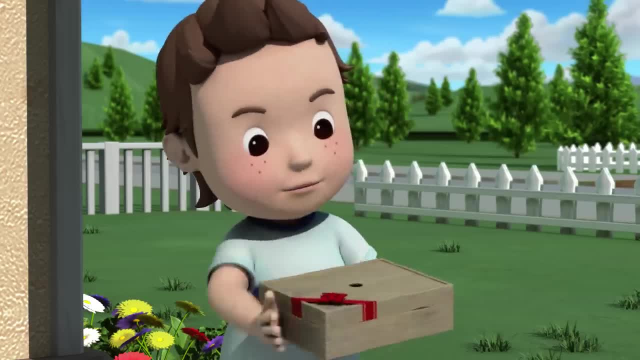 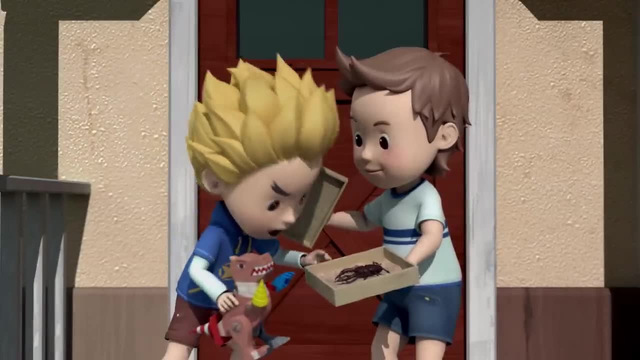 Oh yeah. Well, let's see what you got her. Sure, I got her a present that any girl would love to have. Show me Whoa I want it, Can you? Oh no, This is a birthday gift for Jenny. 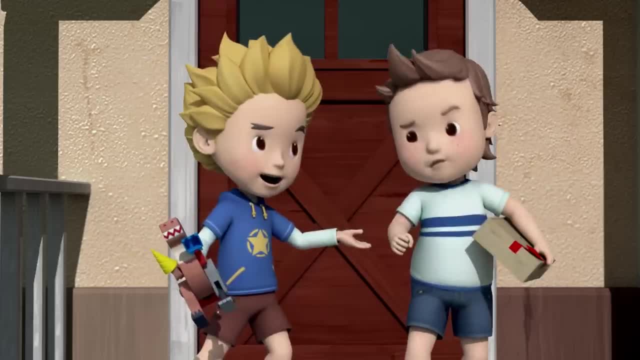 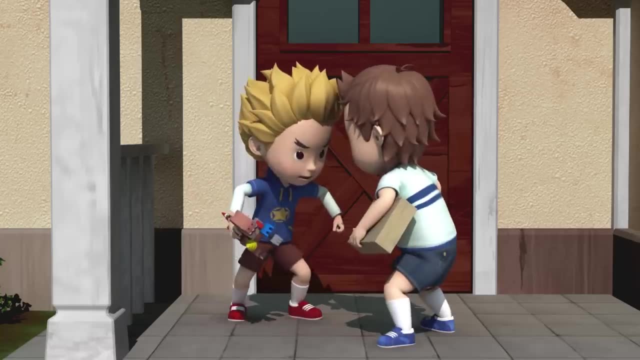 But, Dougie, Jenny won't appreciate a beetle as much as me. I bet she likes it more than she likes your dinosaur. Are you serious? I am. Why don't we go ask Jenny which present she likes better? OK, I'll show her mine first. 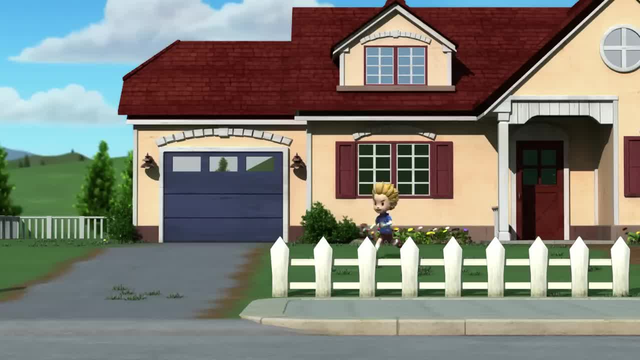 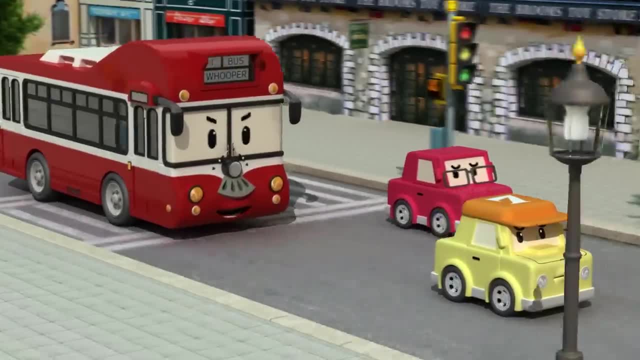 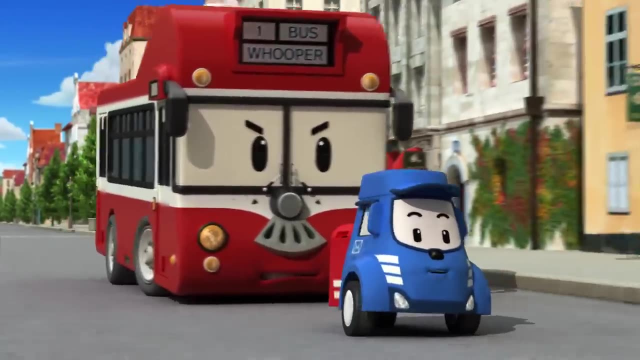 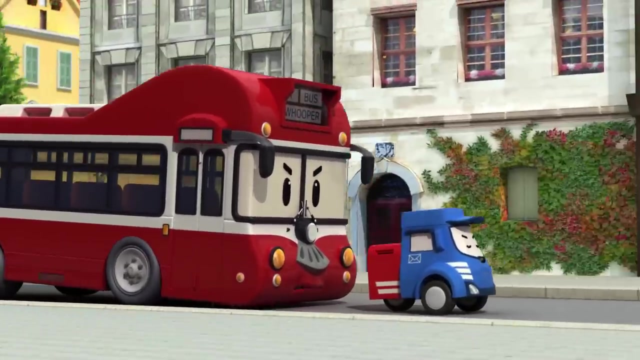 Hey, wait for me. Wait up Doug Coming through. boys, Move aside, please. Hooper's on the road. What a busy day, So many deliveries. Let's go, Guy, I don't have all day, That's your problem. 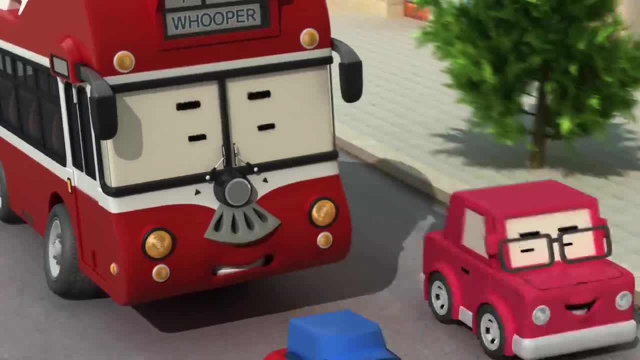 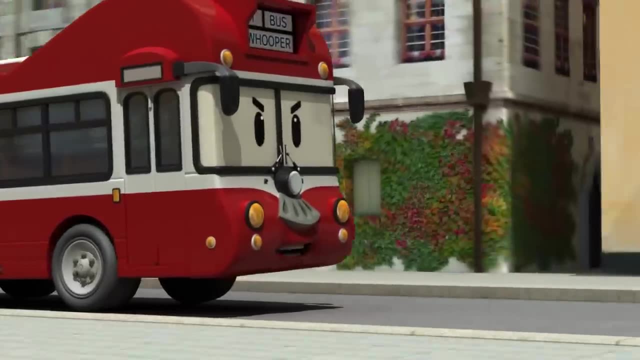 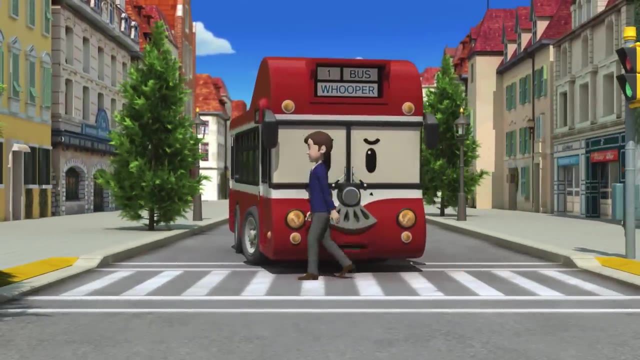 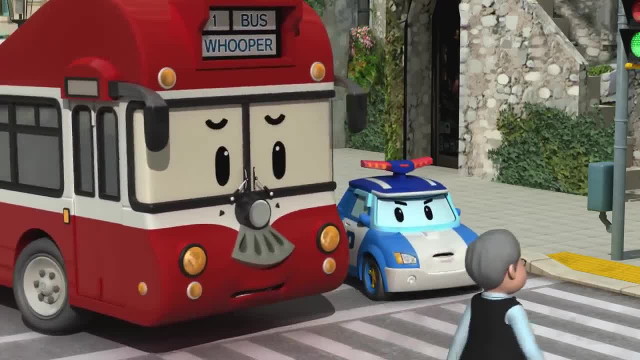 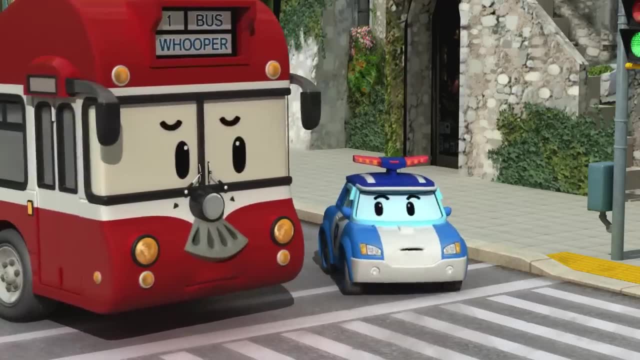 Oh, Oh, Hurray. Well done, throws home. Hooper, You've gone past the stop line. Oh, Polly, What if someone had run into the crosswalk? Sorry, My bad. Whenever you come to a crosswalk, 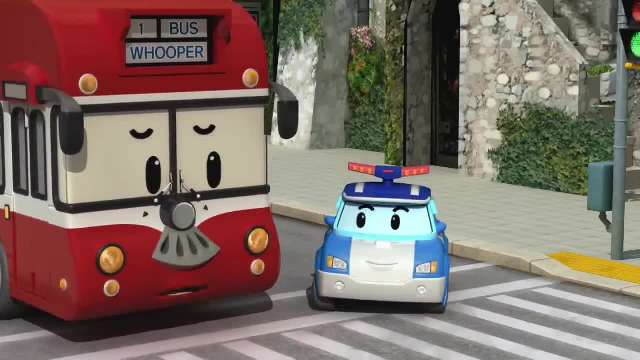 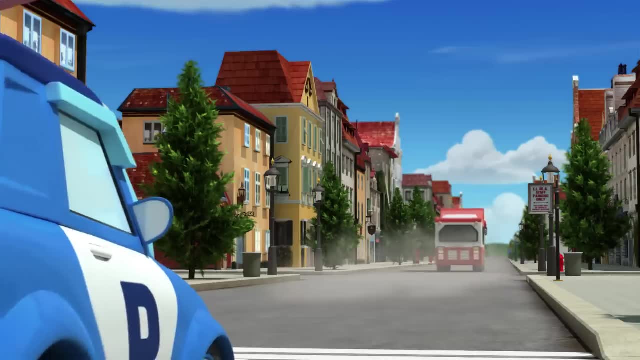 Slow down. OK, Hooper, I will Polly Green light. I'll see you later, Polly Hooper. Awww, I'm not sure he's learned his lesson. Jolly, I'm ready Help me. you poor thing. 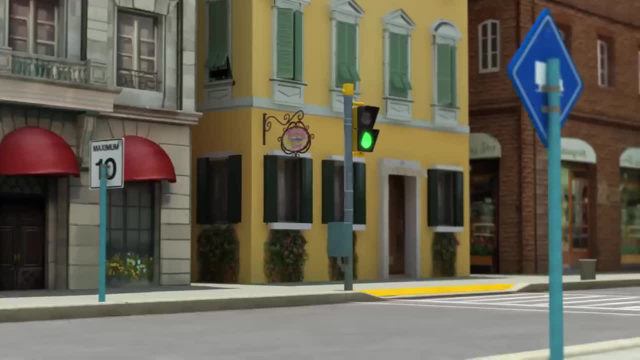 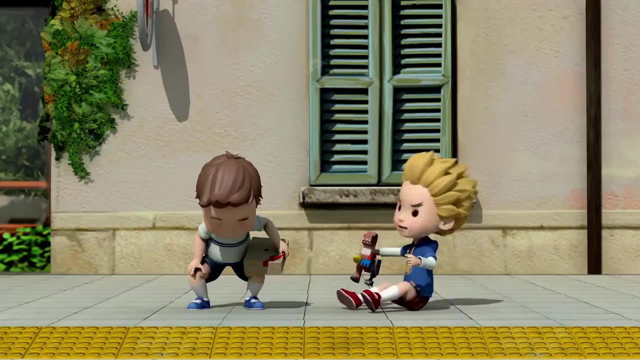 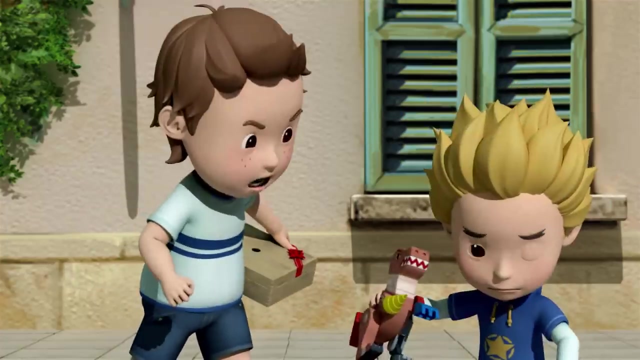 Out of my way. Okay, That should be. That's Jenny's house across the street. Hey, what did you stop for all of a sudden, To wait for the light? You stopped because I was running faster. Excuse me, I was way ahead of you. 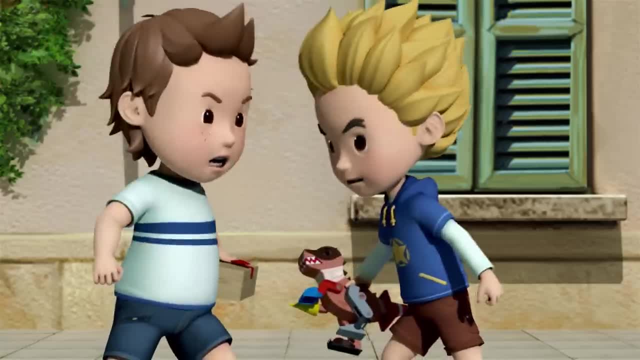 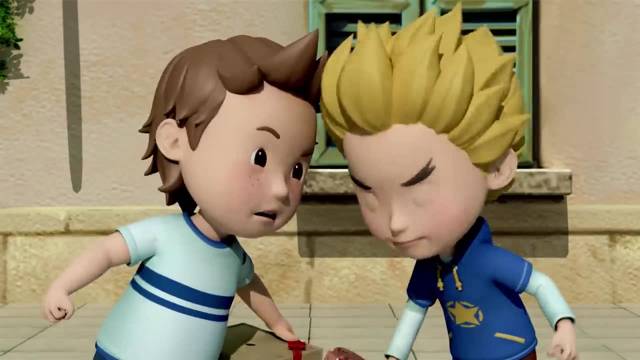 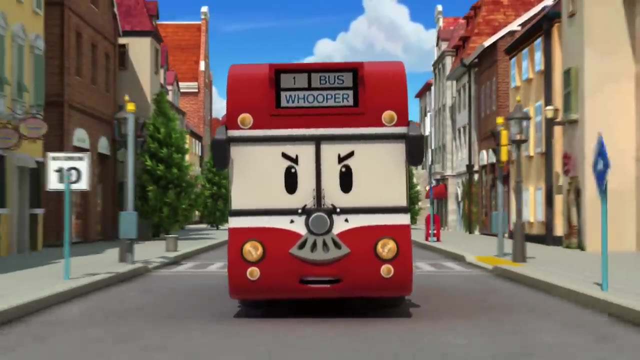 Yeah well, I was just going to pass you. Oh yeah, Fine, let's see who's the fastest one. Great, but it's not going to be you. Yeah, that posty, He's always putting me behind schedule. 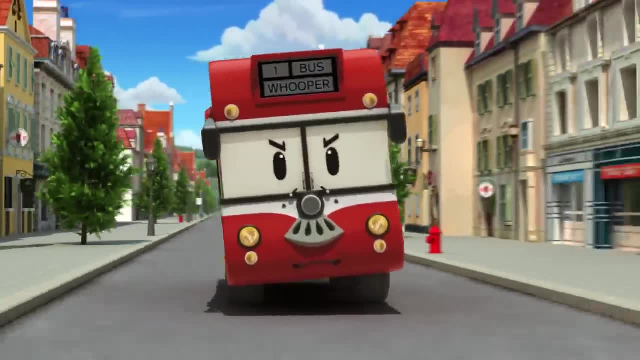 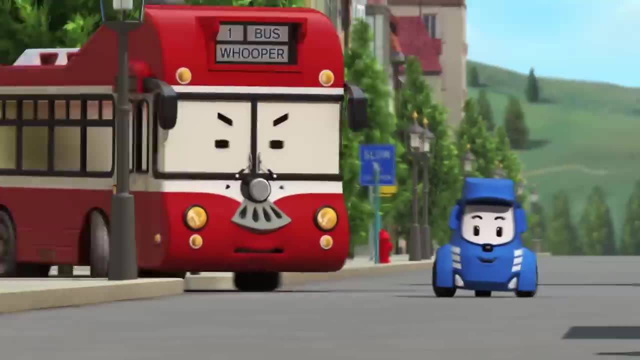 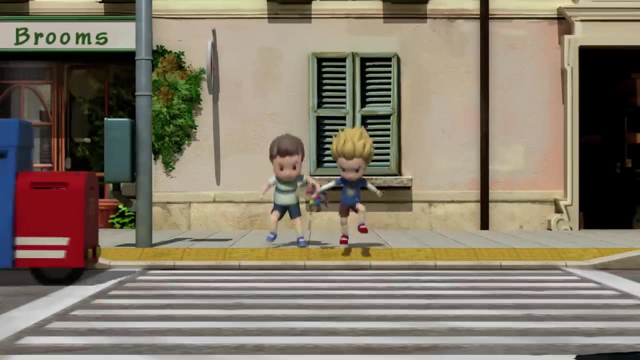 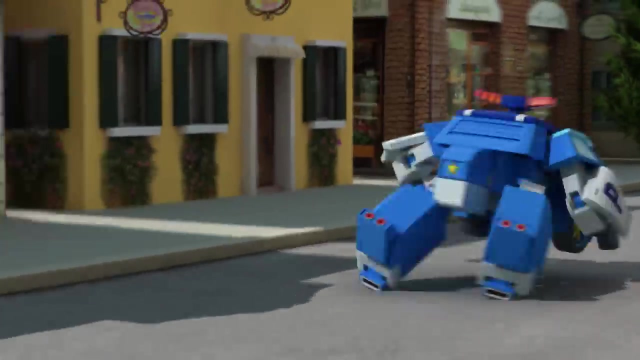 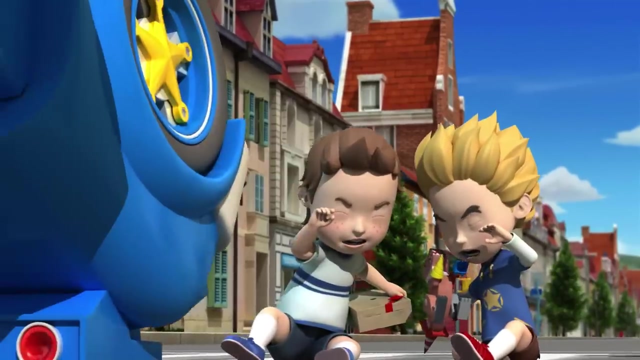 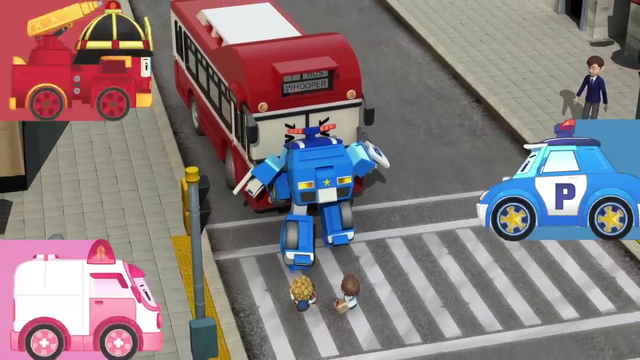 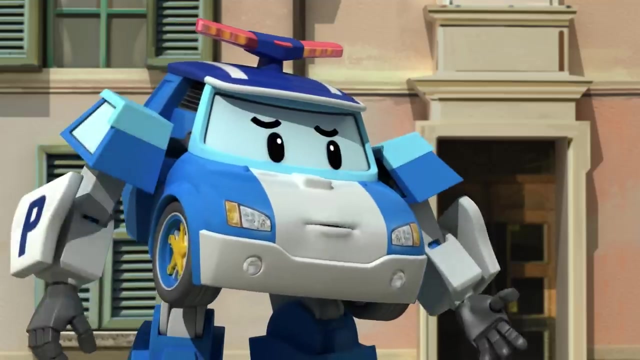 There he is. He won't block me this time. This could get really dangerous Green light go. Hey, Ah, Polly Wooper, you should have slowed down. Oh You boys, okay. Yes, Kevin Doug, you should never run across the street like that. 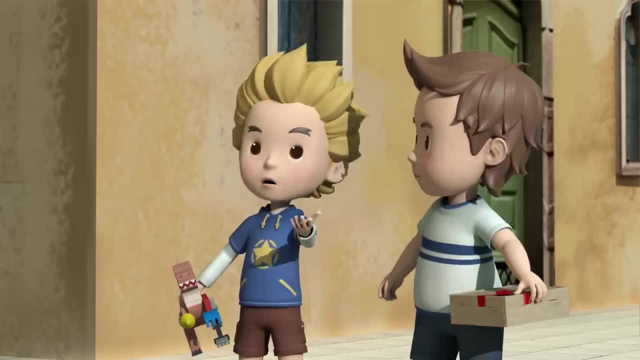 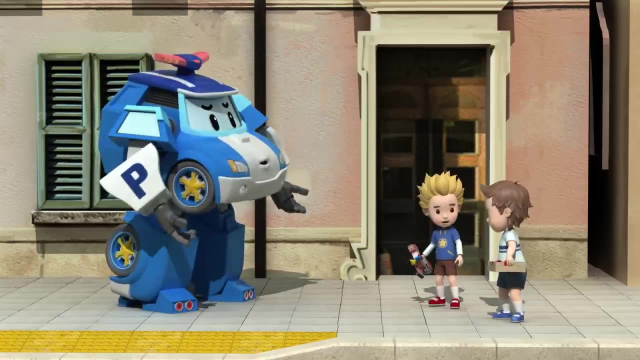 even when the light is green. But, Polly, I thought it was okay to cross when it's green. Yeah, me too. Green means go, but just because the light's green doesn't mean it's safe to run across. Some cars might miss the light change. 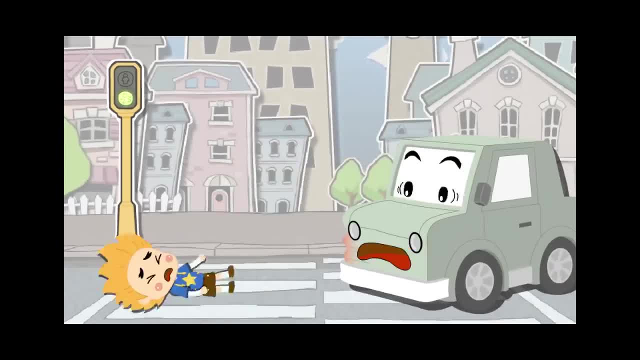 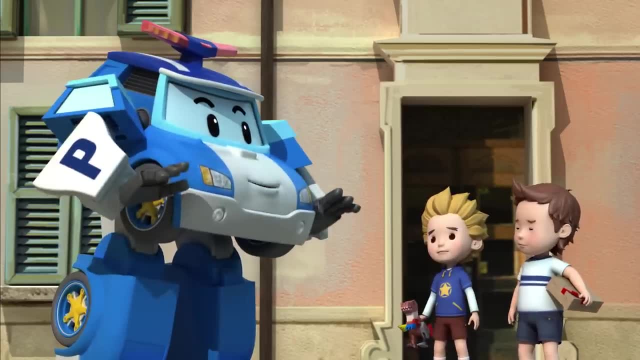 and not be able to stop in time. Then what are we supposed to do when we have to cross the street? Polly, We'd fly if we could, but we can't, I know. Just remember three steps and you can cross the street safely and easily. 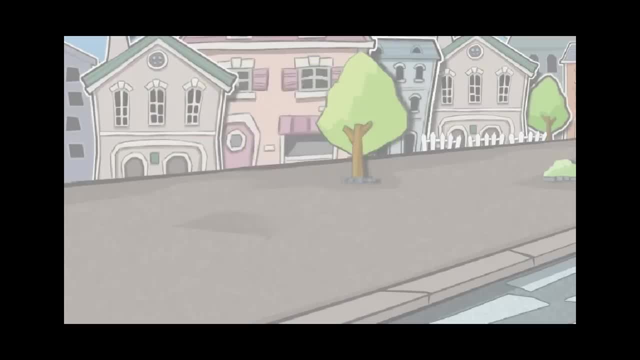 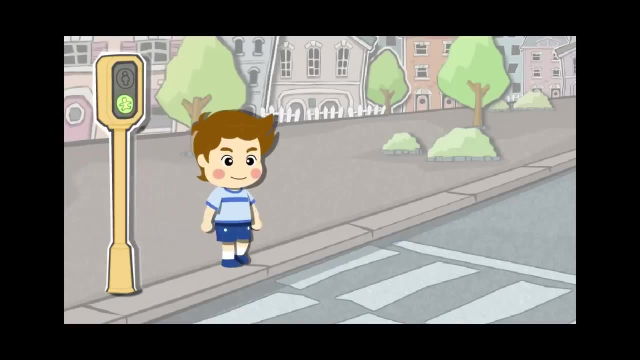 Three steps. Step one: always stop at the curb before you enter into a crosswalk and wait for the green light. And even if the light is green, stop and look in all directions first. Step two: make sure all cars are stopped before you cross. 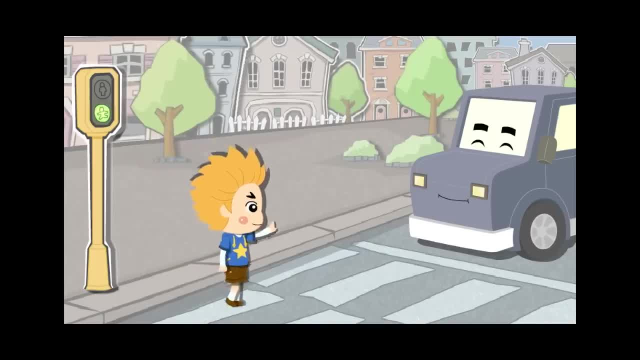 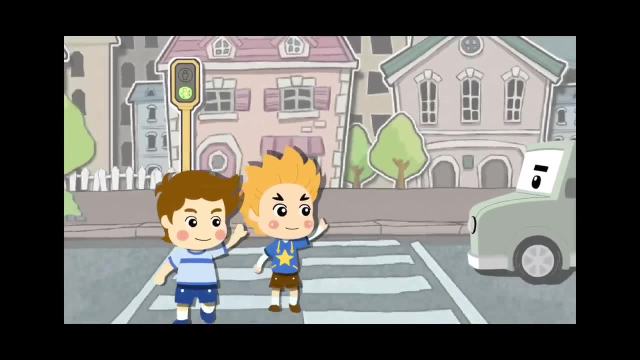 Make eye contact with the drivers and check that all cars are stopped as you cross Step three: don't take your eyes off the cars while you're crossing. Always keep watching to make sure that you see the cars and the drivers see you. Okay. 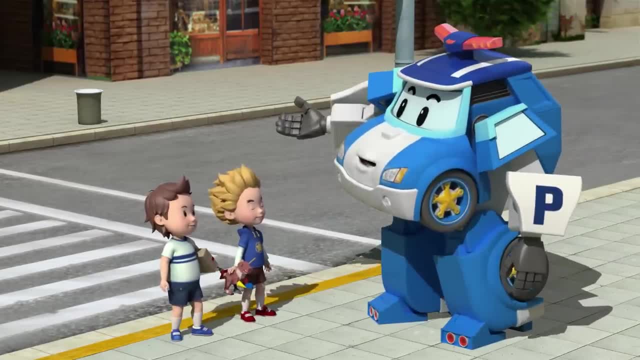 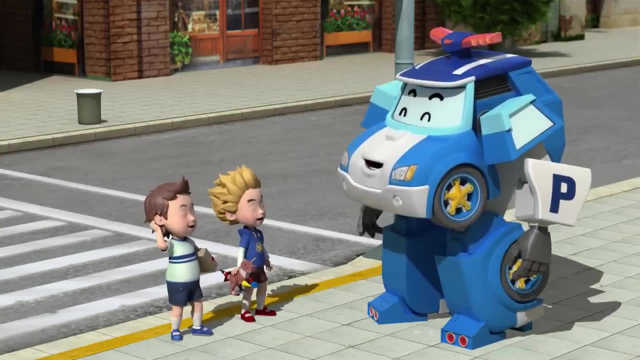 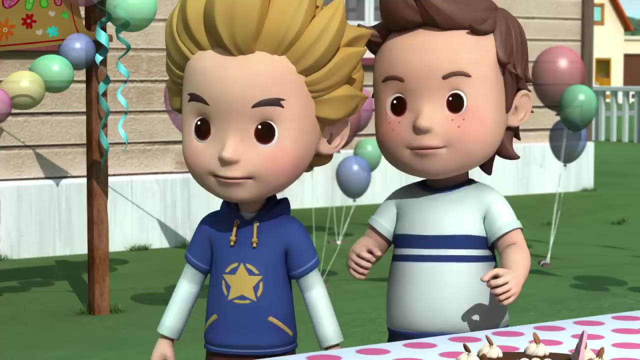 Pretty simple, right guys? Yeah, Just remember, it's not about how fast you cross, it's about how safely you cross. Got it, Got it, Polly. Happy birthday, Jenny. Thanks guys, Jenny, I got a birthday present for you. 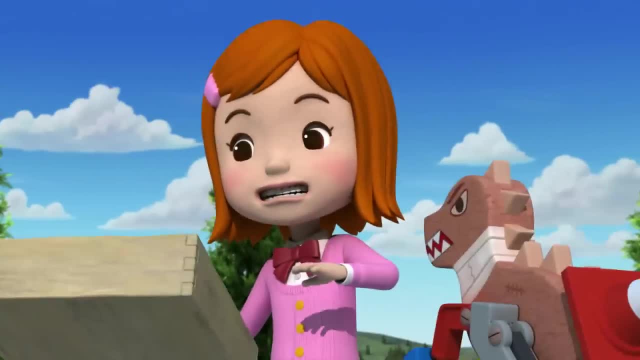 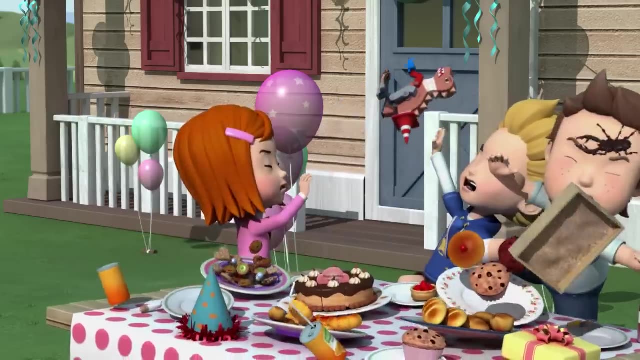 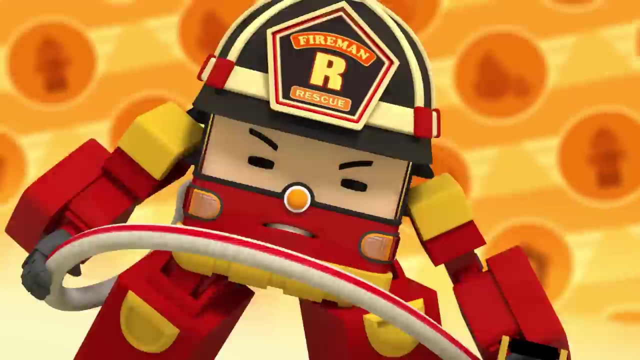 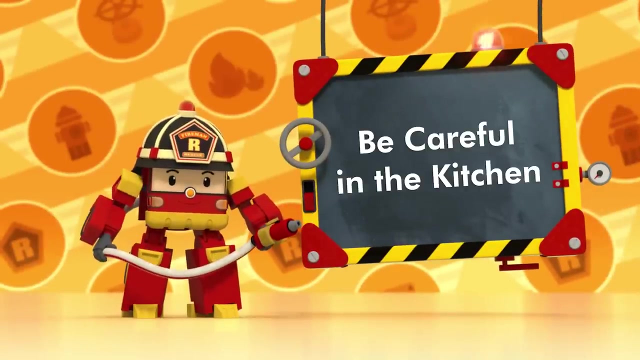 Which one's better? My dinosaur's better. right, A beetle that's alive is way better. It's a tie. What do you mean, Jenny? I hate them both. Bye, See you later then. Bye, bye, mom. Have a great time honey. 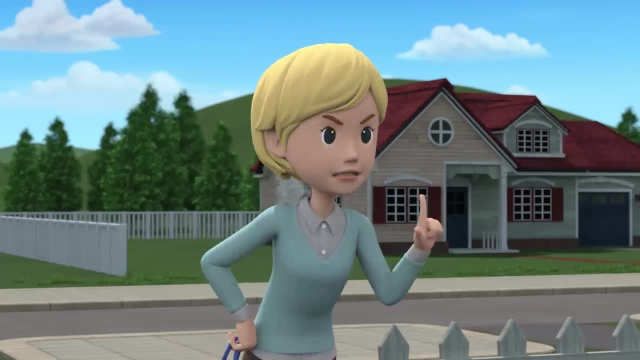 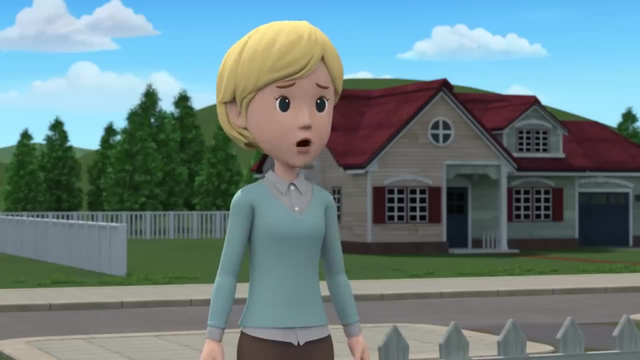 You seem too happy. I'm leaving You better remember everything you promised me: Get all of our homework done, Don't leave messes anywhere, And I will not let the children starve. Please don't give them only junk food, alright. 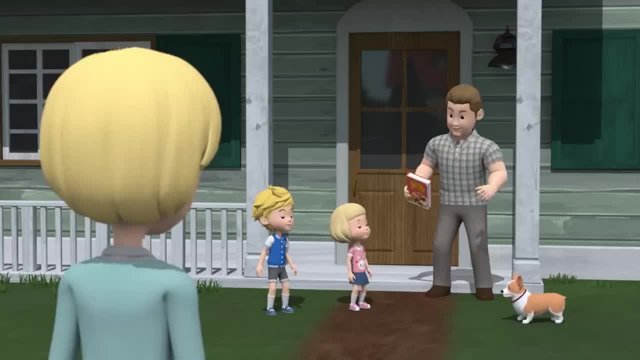 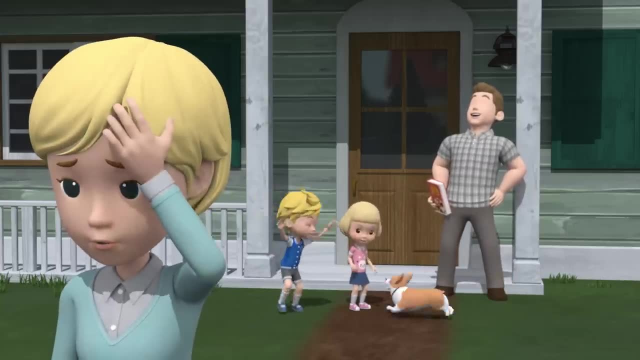 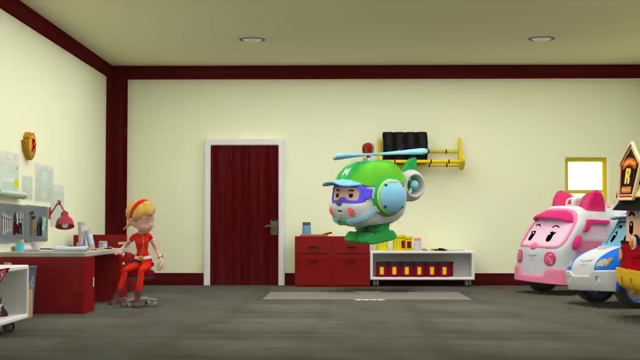 Not gonna happen. I'm making something from the book. Look, I'll make you whatever you want, as long as it's in here. Wow, Dad, that sounds awesome. Yahoo, I'm finally done. Jin, What's that? Jin? 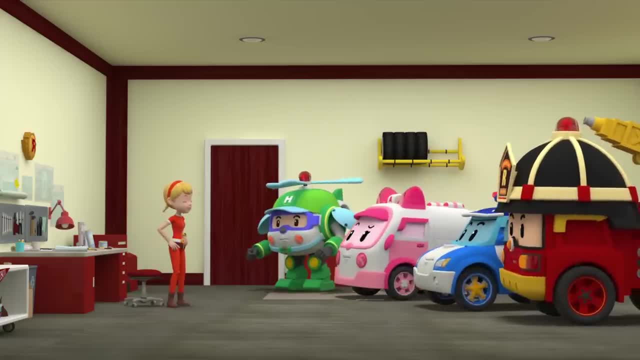 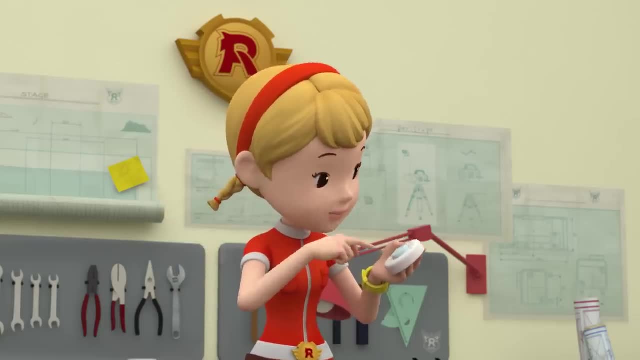 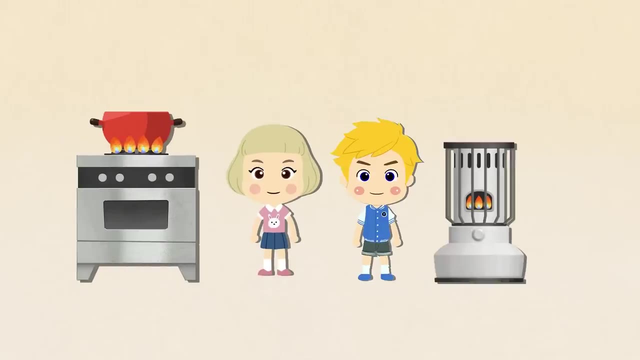 This is called the three-step alarm. Three-step alarm. I've never heard of that. That might be because I just invented it. It rings when children cross into what should be a child-free area. Child-free area, Yeah, a child-free area is a one-meter zone around things that can cause an accident. 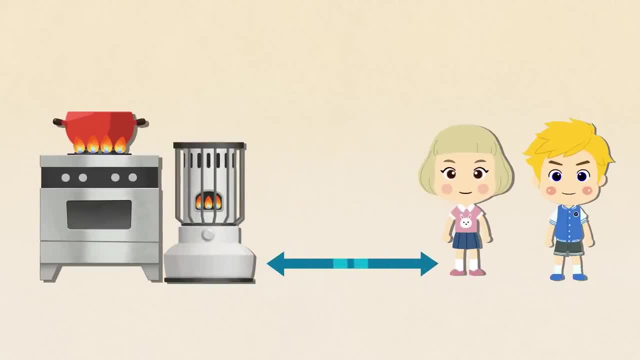 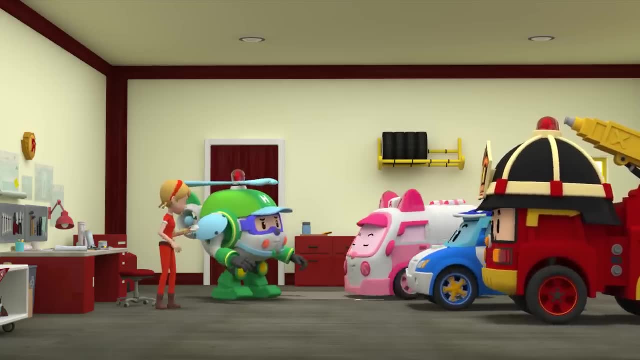 like a stove or a heater. Children should be kept from entering that zone. Very smart Huh. Why is it ringing Jin? Well, a child walked into the area, didn't he? I am not a child. Just because you're big doesn't mean that you're an adult yet. 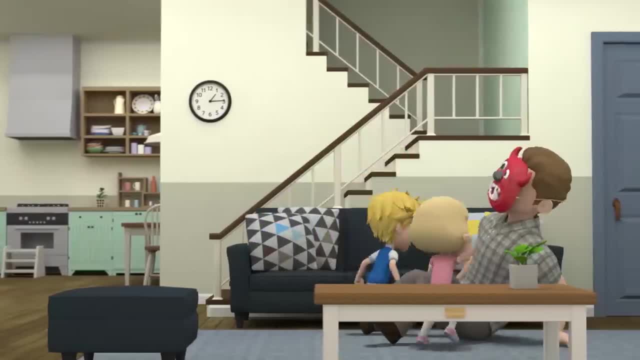 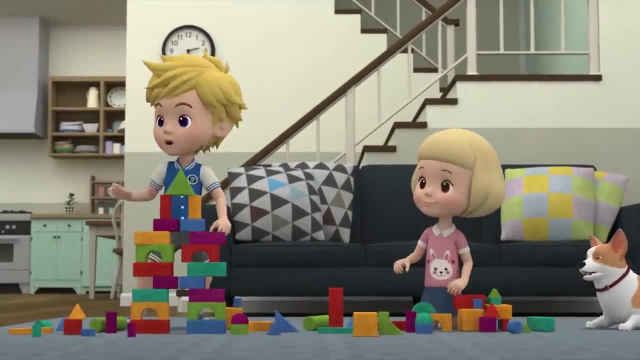 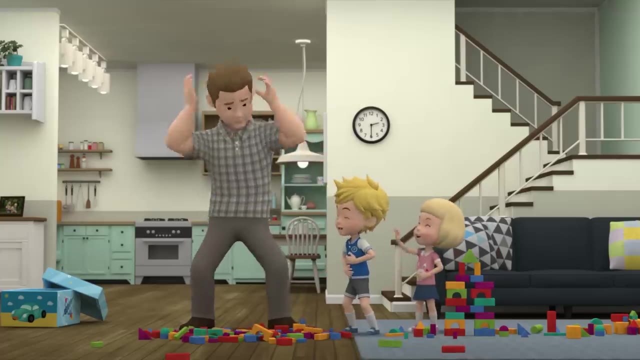 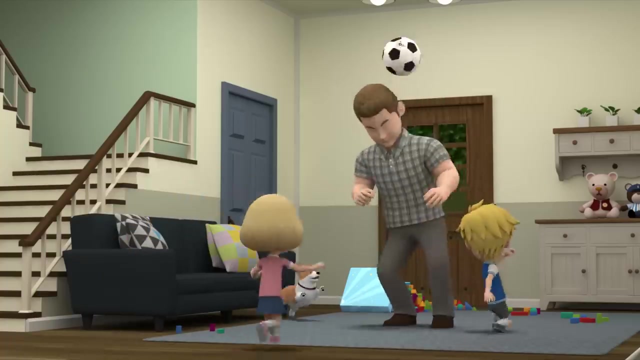 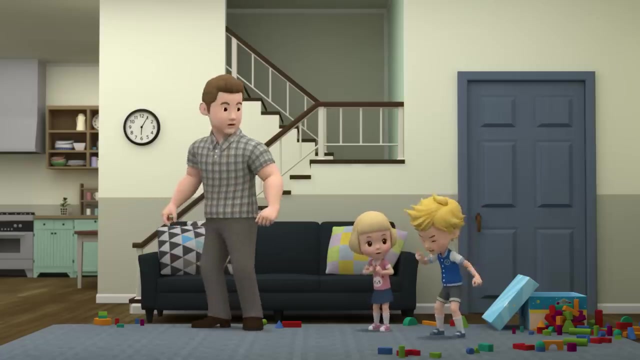 Roar, Go away monster. That's amazing. Dad, It's done. I'm funny. Not a chance, Not a chance. And he shoots: Sweet, You're out, Dad, Dad's out, Huh, It's Mom. 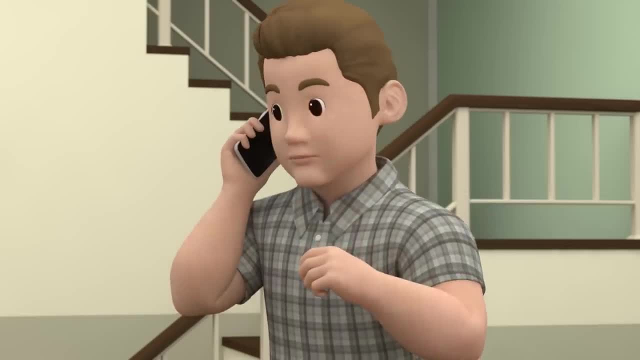 Shh Hm, Shh Ahem. Hello, Everybody's fine. Peter, Of course he's doing his homework. Lucy, Oh yeah, She's picking up her toys Dinner Yup, Almost done. It already smells great. 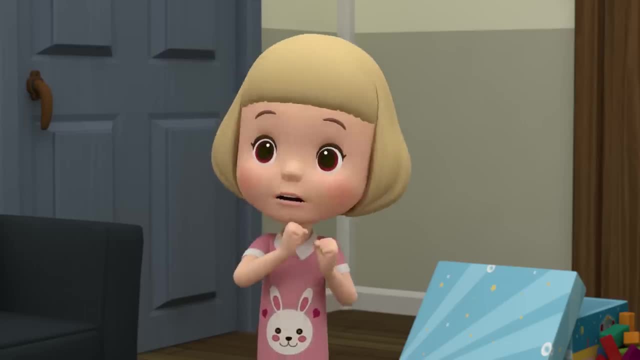 Guess I'll move along now. Please don't forget to install your new three-step alarm. We'll install it. Thanks again, Buh-bye, Roy. Next stop is Little Peter's house. It's a nice little house. It's a nice little house. 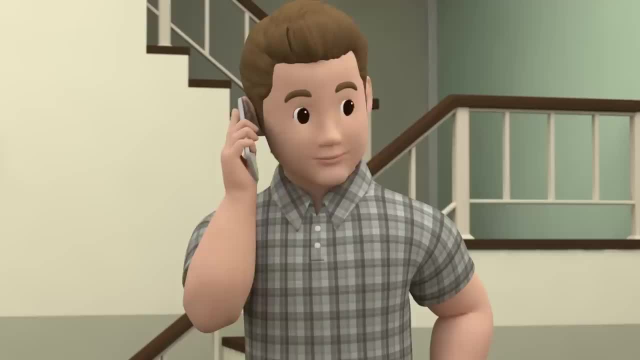 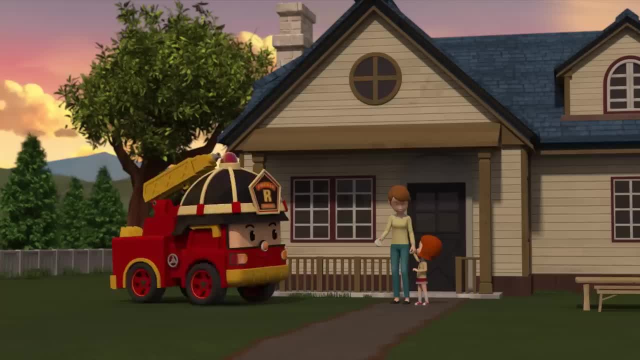 Right, First we chop all the onions up. This is how you do it, Like this: Come on, Dad, Let me slice a few. Come on, Dad, Let me slice a few. Come on, Dad, Let me slice a few. 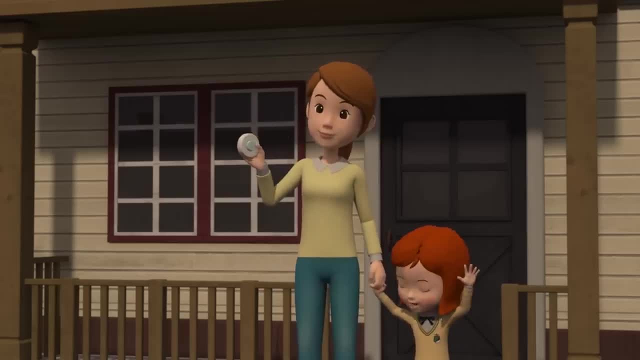 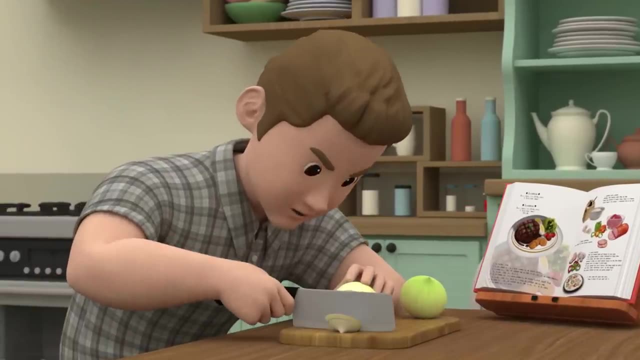 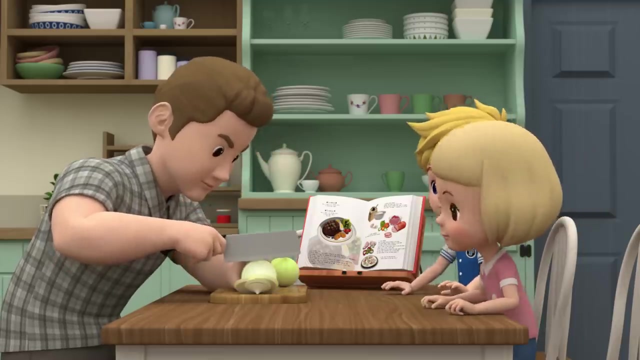 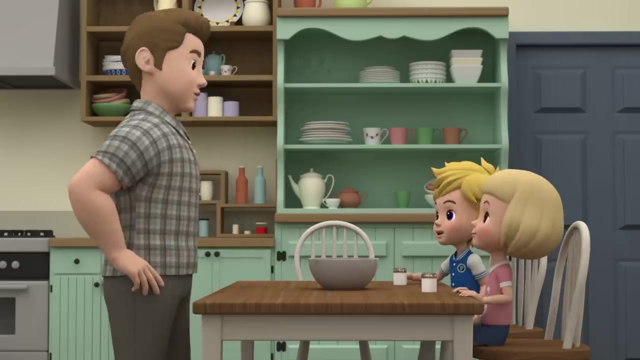 No, no, Knives are dangerous. Oh, Oh, Hmm, Oh, My knife Ow, My knife Ow Dang it halls Raven, ihen Reynolds, Undyne Tootsies. Now, who wants to sprinkle the salt? 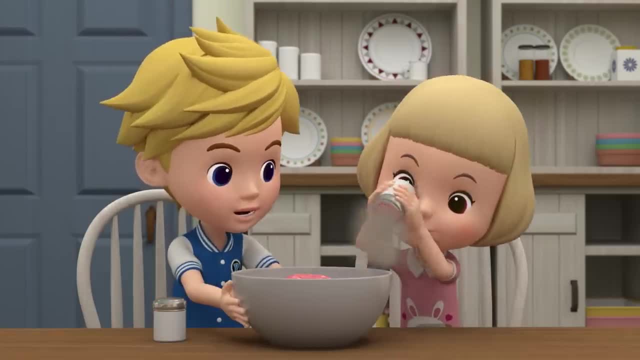 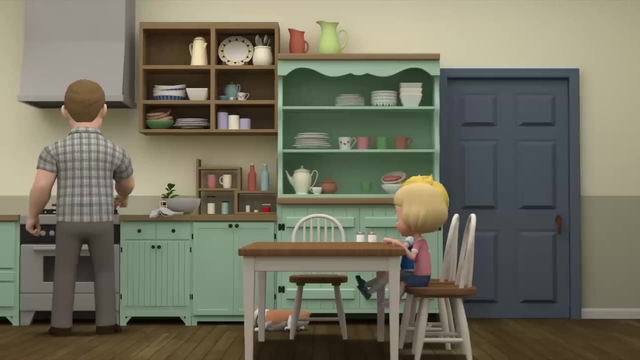 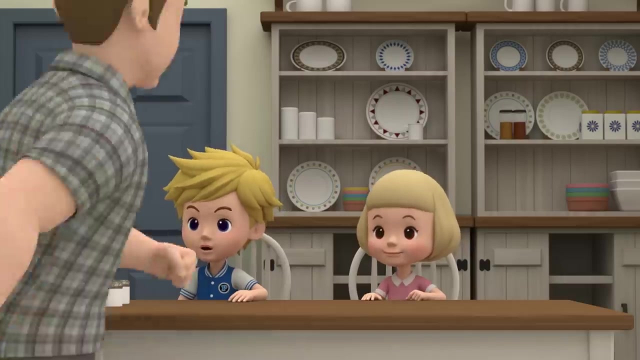 I do Take that. Now. the pepper: Adieu, Adieu, Whoa Smells great. It's almost done, Bet, that's Mom. Hang tight for a second. kids, Hello, Hey, honey, what's going on? 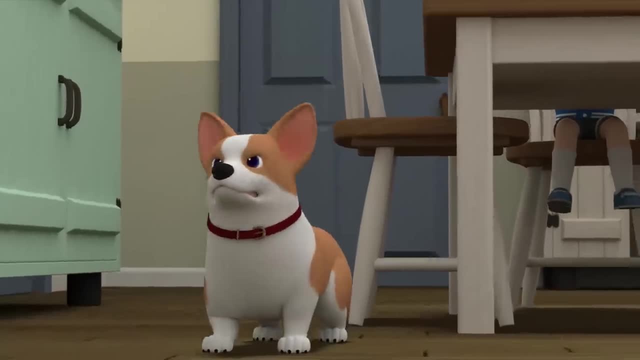 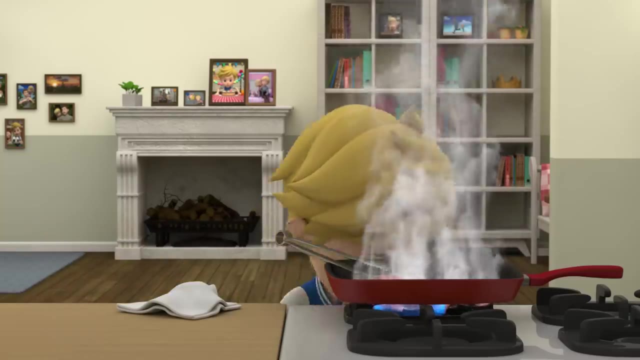 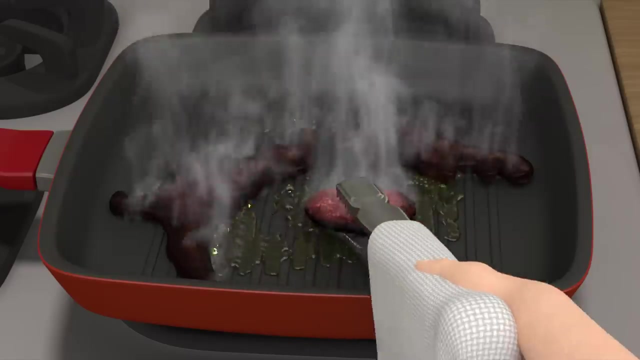 Me too. What is it, buddy? Oh no, The meat's burning. Peter, what are you doing? The meat's going to burn. It needs to be turned. Ow Hot, Oh, I just turn other side. 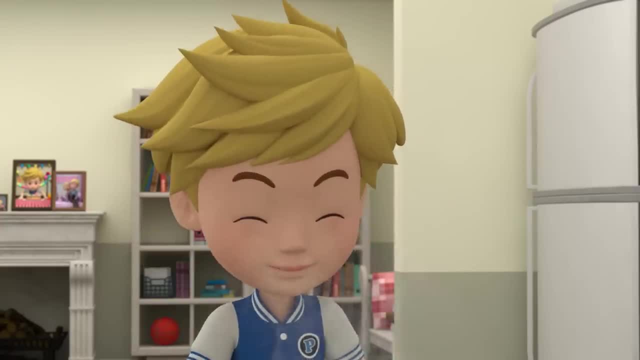 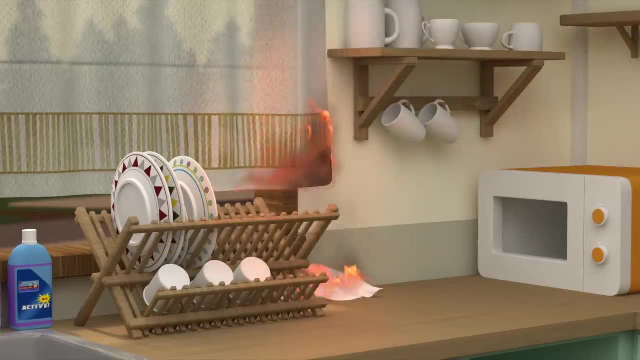 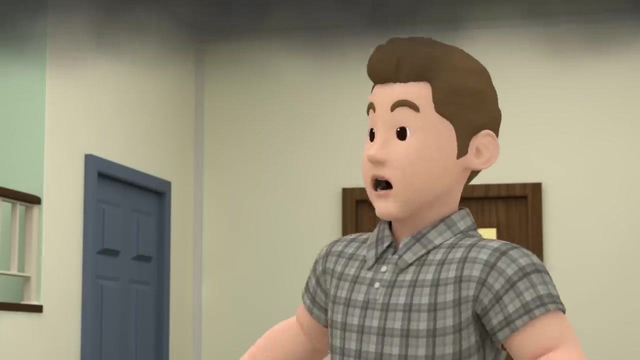 and done. Peter, Peter, Peter, Lucy, why do you keep screaming? Just look, Just look, Fire, We'll have dinner any minute. now, Hurry home Children. Huh, Smoke's coming out of Peter's house. 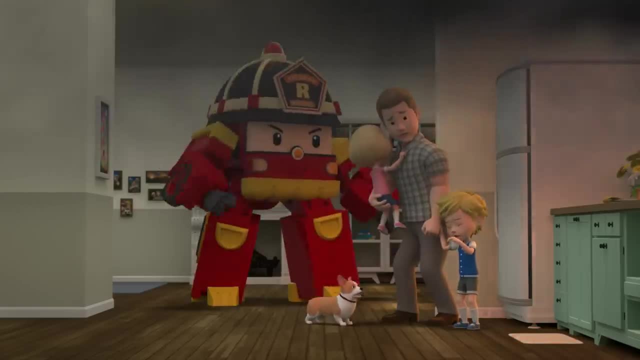 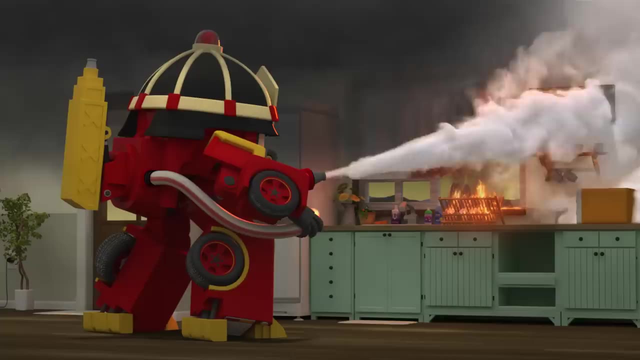 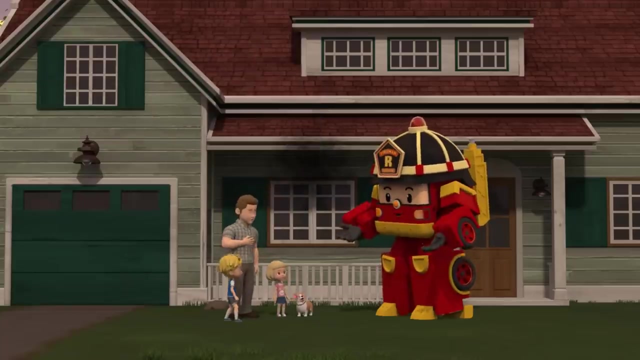 Peter, grab onto my hand. Okay, Children, Robert, You all need to get out of the house, Right, Sure, Huh Huh, Just thank goodness, Just thank goodness that nobody got hurt. Thank you, Roy. You saved all our lives, I'm sure. 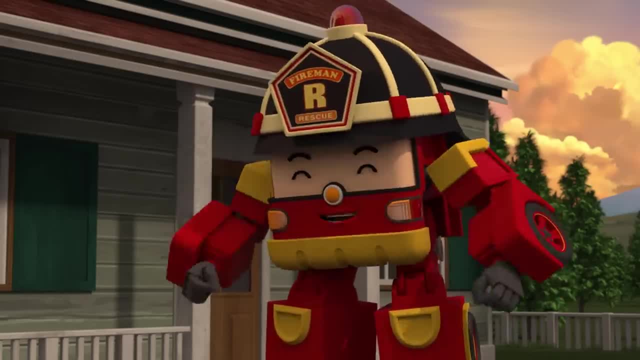 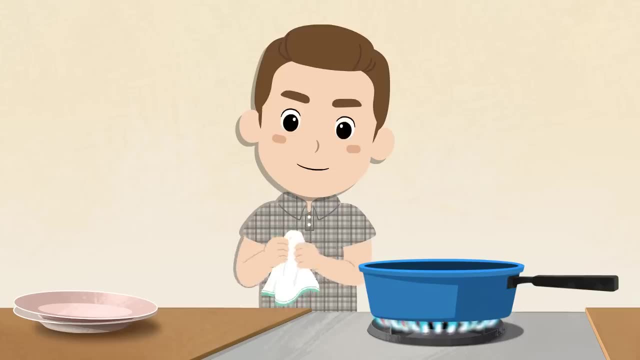 To make sure that this doesn't happen anymore, I've got some safety tips for you When you're cooking. never leave the kitchen while the stove is on. A fire can break out at any time. Also, put nothing flammable, such as towels or paper. 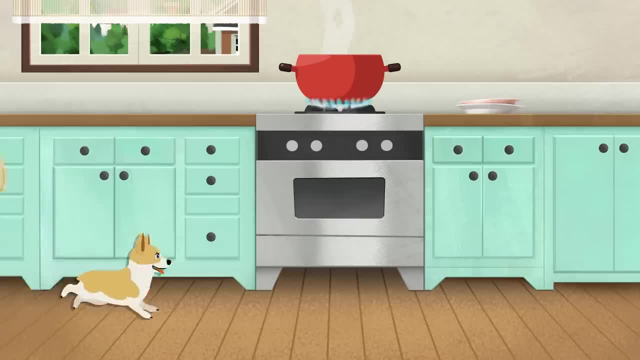 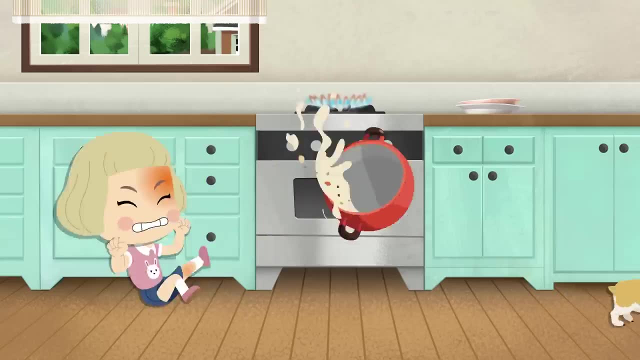 near the stove's flame because these can easily spread fire, And don't let pets or children get near the flames or the hot food. They might have an accident and, since they won't know how best to deal with it, they could be seriously injured. 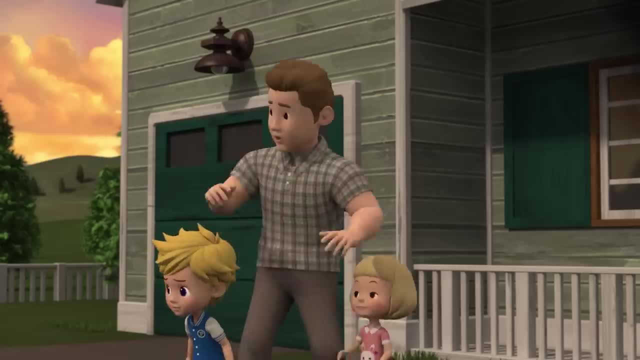 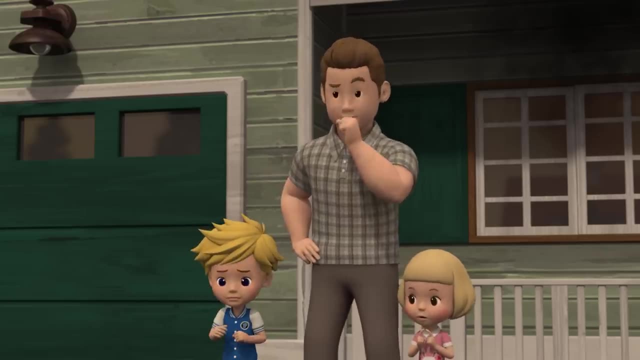 Yes, All right. What's going on here? Huh, It's Mom. I'm home because you said dinner would be ready. now Why are you all outside? Uh well, Ahem. Well, honey, you know about the dinner. 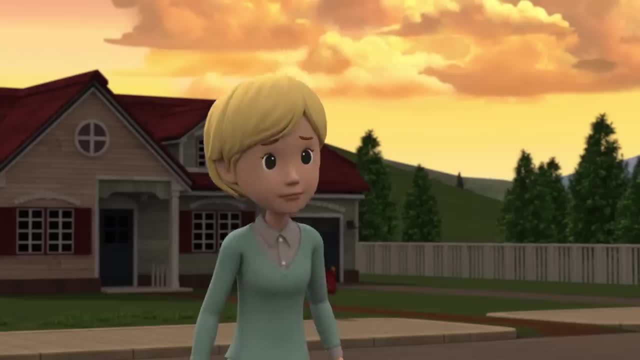 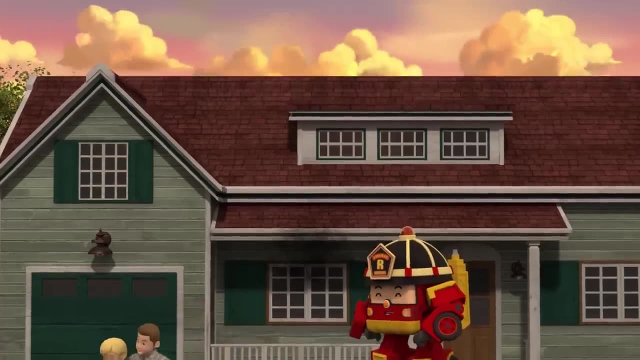 the thing is, uh, we're eating out instead. What are you talking about? I just thought we'd go out to eat. Yay, We're eating out. All right, I got a new book: Eating out. Eating out. 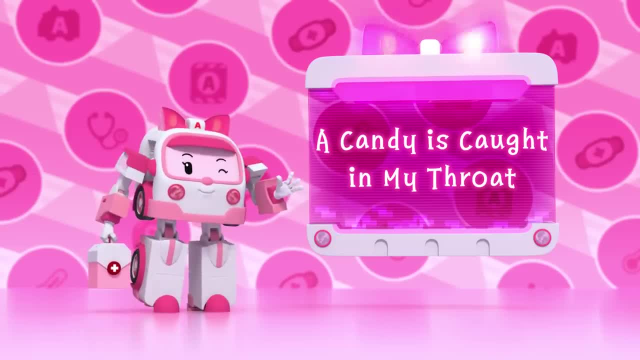 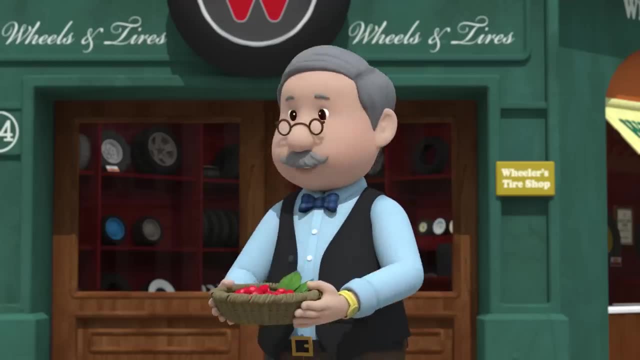 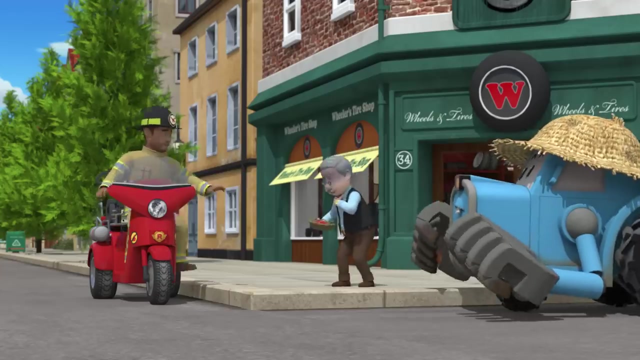 A candy is caught in my throat. Hello, Mr Wheeler, Hi Tracky Morning, Tommy, You're just in time. Have one of these fresh raspberries. Tracky gave them to me. They're just heavenly, Mr Wheeler. 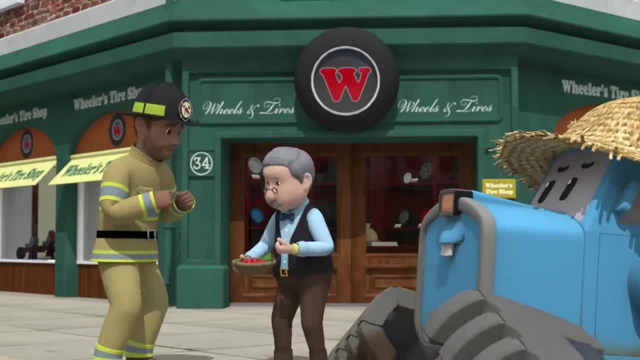 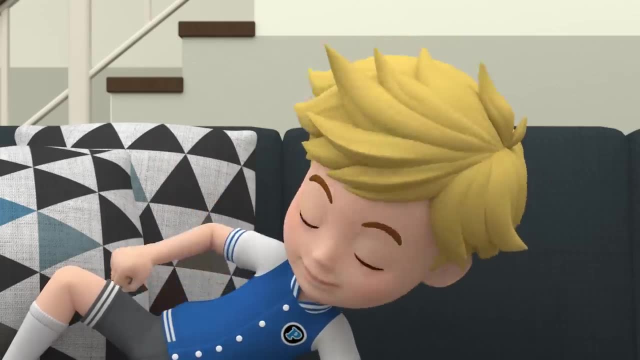 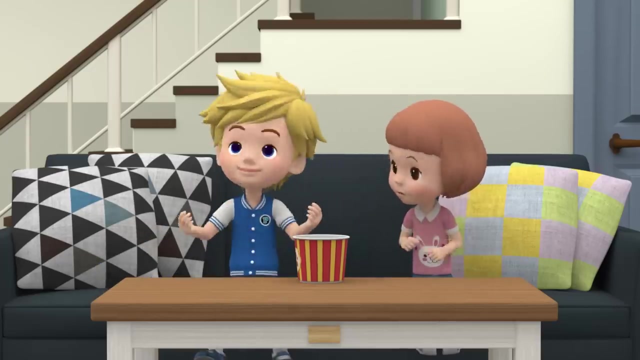 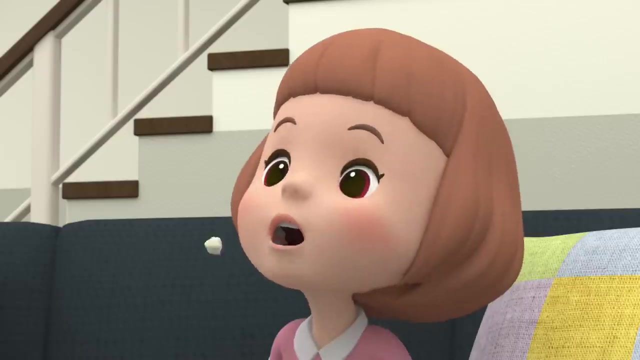 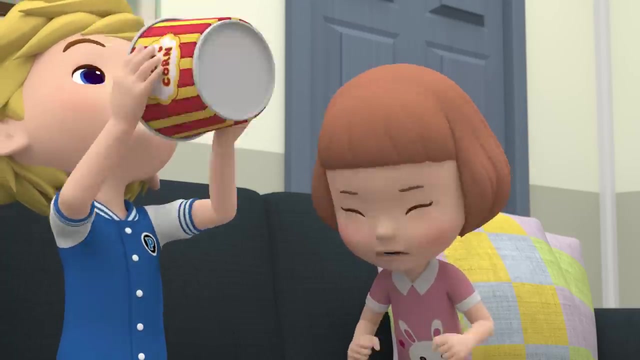 I'm all right. Thank goodness, you're fine. Lucy, check this out. Who's the best? Wow, I want to try it. Watch what I do. Ta-da, I'll do it this time. All right, Peter, How could you eat all the popcorn? 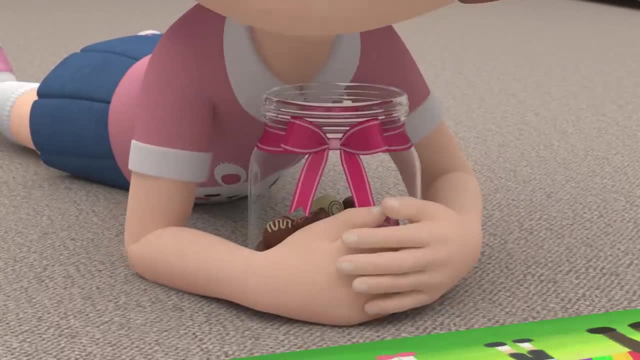 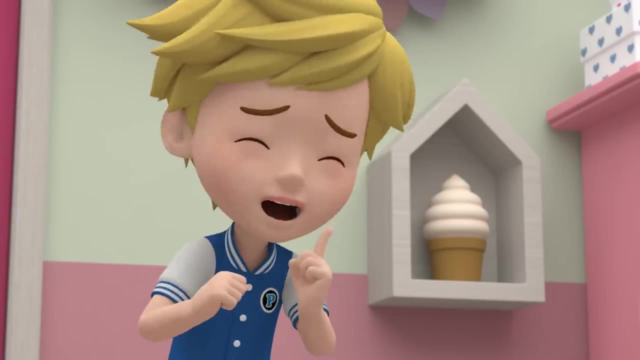 Lucy, can I have one little chocolate? Sorry for before Now. just one, Hmm, Nope, That's not gonna happen. Only one, I'm begging. Fine, You can have one. Hmm, Thanks, sis Peter Ha. 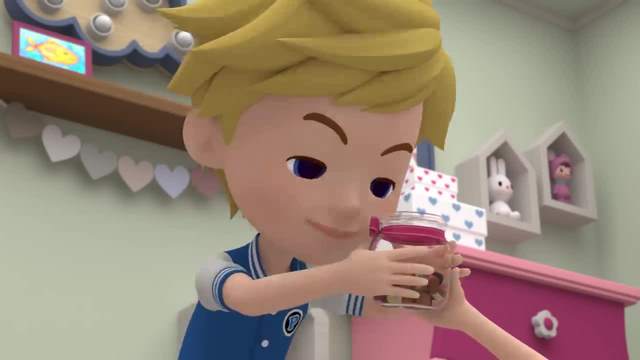 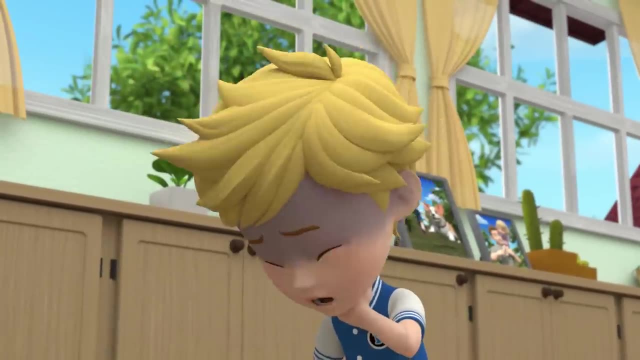 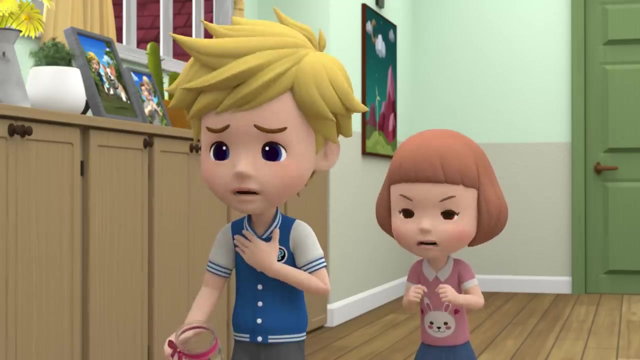 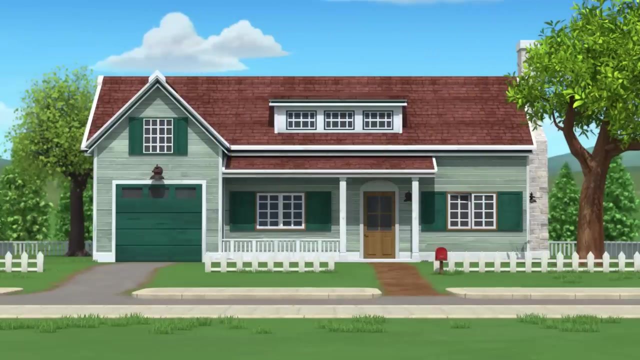 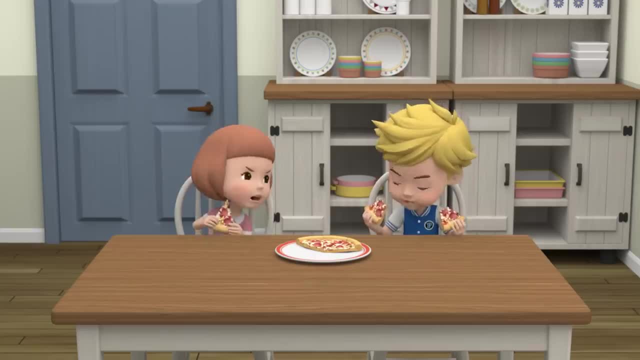 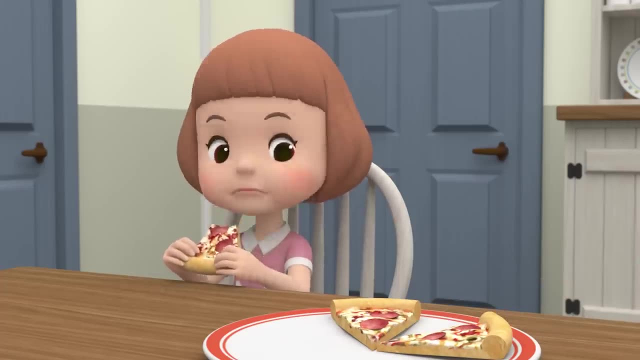 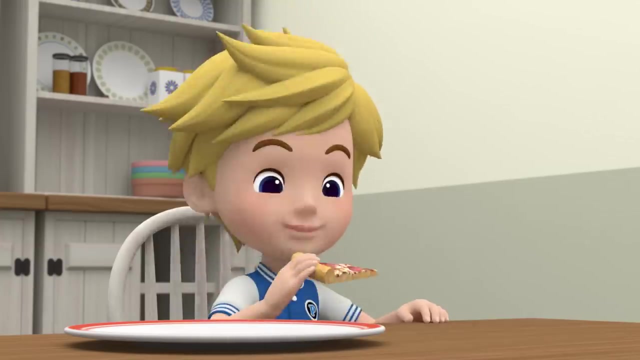 Huh, Ew, that's gross. Kids Pizza. Yes, Peter, you eat two pieces at once. Stop, You can eat just like me if you want. Huh, Last piece is mine. No Fried dough, You're the worst. 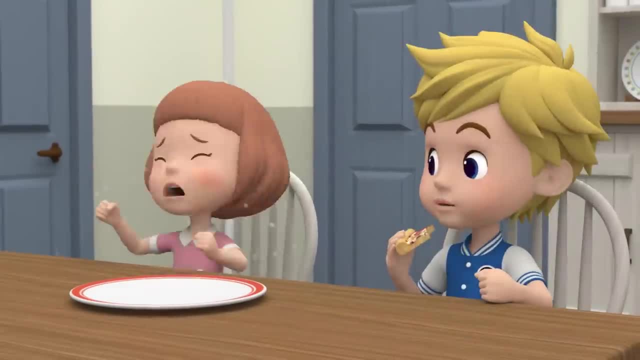 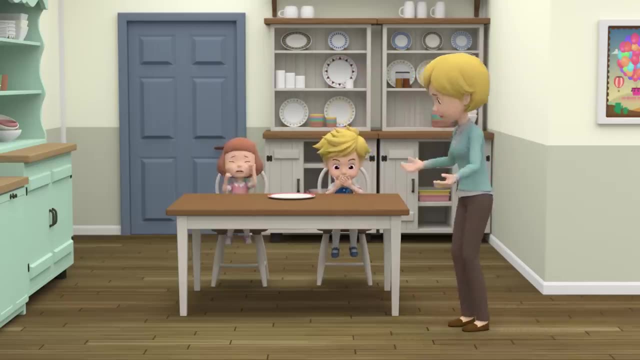 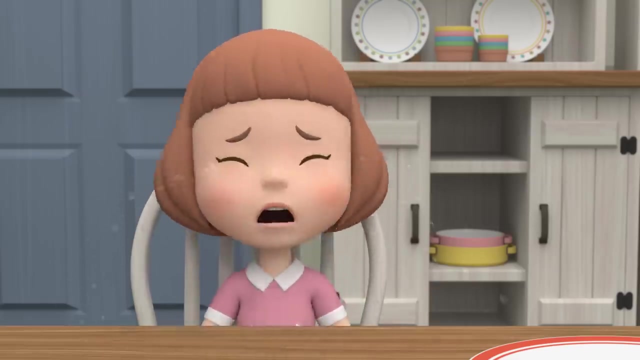 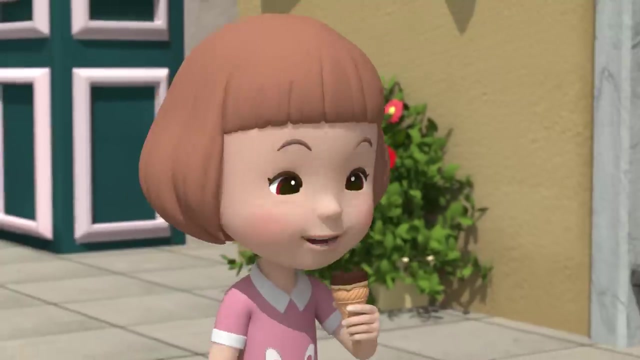 Lucy. What's wrong, Peter? Well, Peter hogged almost all the pizza to himself, Peter. Uh well, it's just, you know, Lucy, Lucy, Lucy, Lucy, Lucy, Lucy. is it good? Uh-huh Yeah. 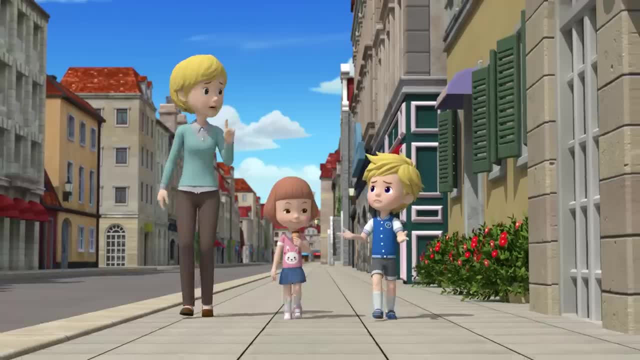 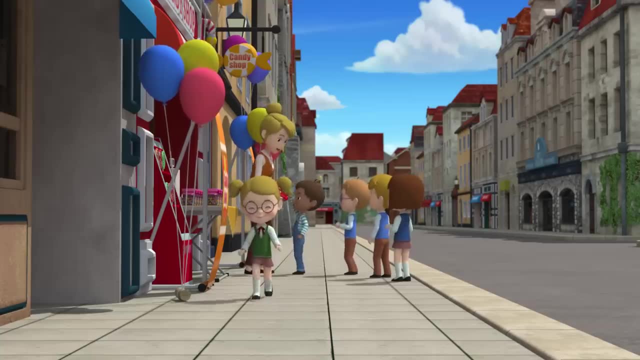 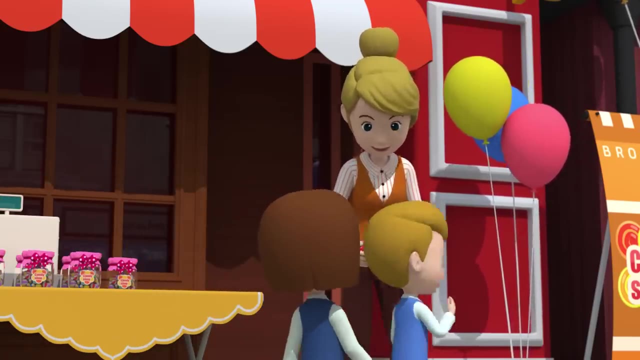 Come on, I want some ice cream too. No, sir, You ate too many snacks already. Hmm, Free candy, Free candy for our grand opening. Yummy, Can I have one? Me too, Of course, Here. 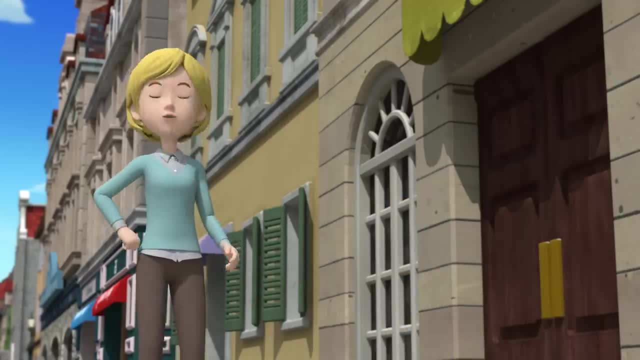 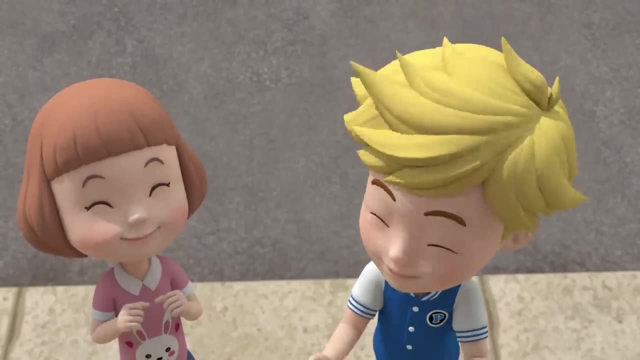 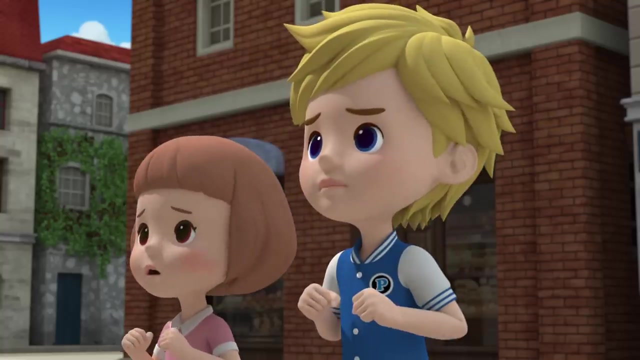 Whoa, Free candy, And they're off. Welcome, Help yourselves. Oh Yummy free candy, please, ma'am, Me too. Oh dear, It looks like there's only one piece left, Only one. This is mine. 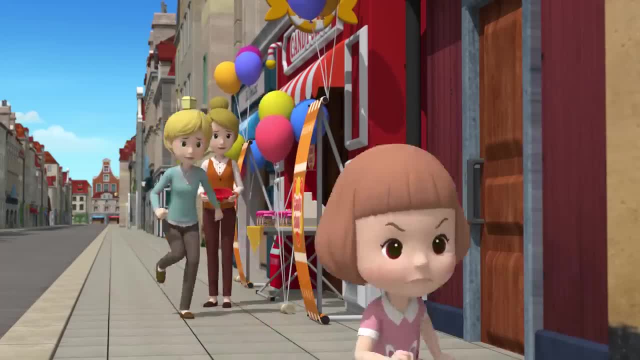 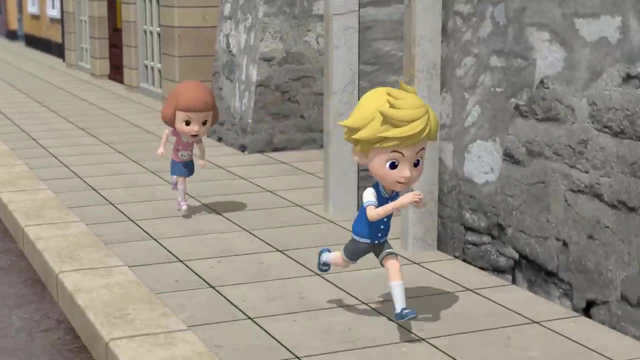 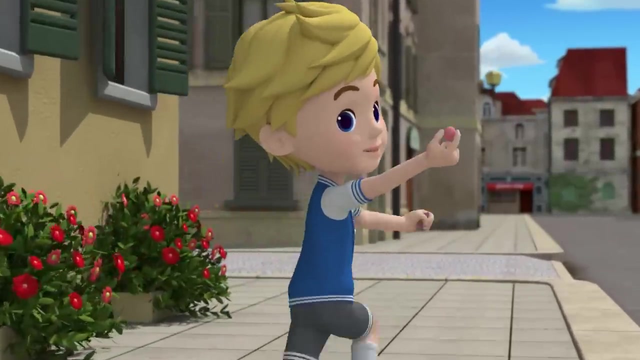 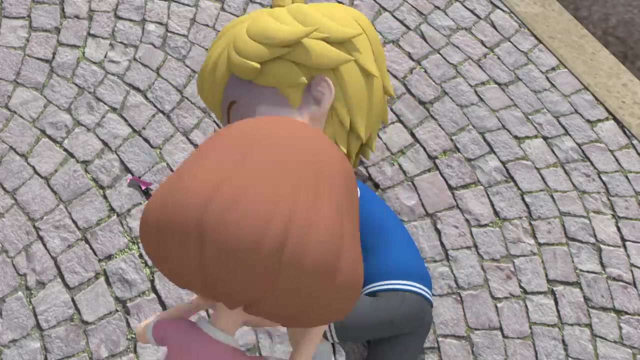 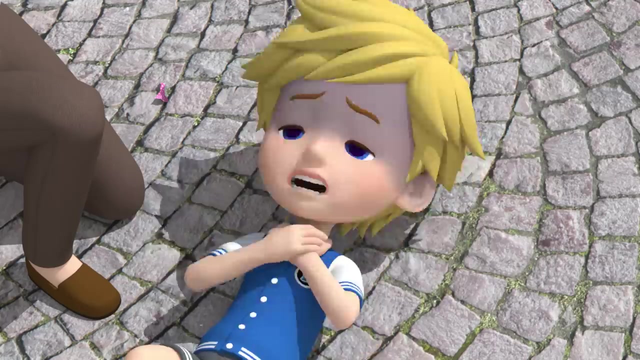 Peter, Peter, Lucy, Stop, Peter. What's this? Hey, Stop. That piece of candy is mine. That's fine, Honey. then why is it in my mouth? Serves you right? What's wrong, Peter? What's wrong son? 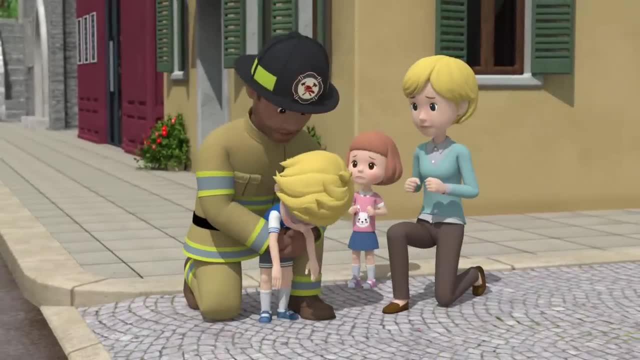 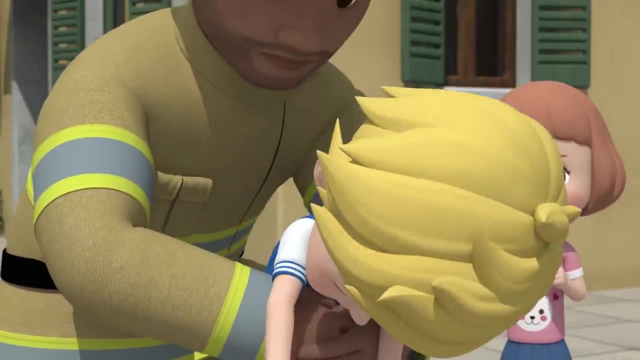 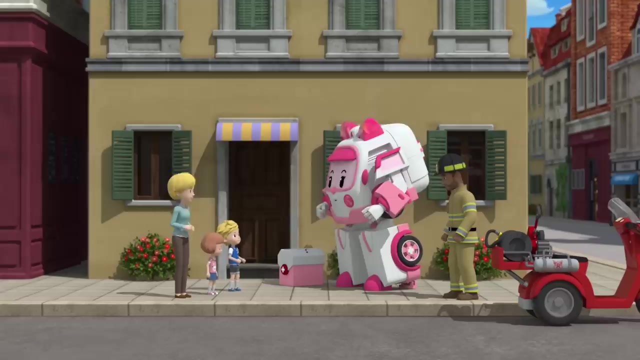 The candy must be stuck in his throat, Peter. Hang in there, Peter, Feel better. Yeah, Phew, Thank you so much. You're lucky. you're all right, Peter. Thank you, Amber, You're very lucky. I happened to be near. 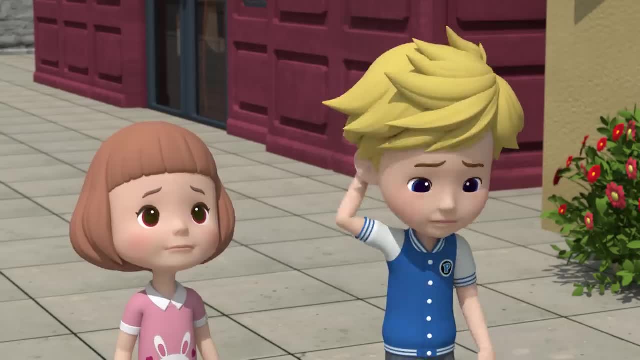 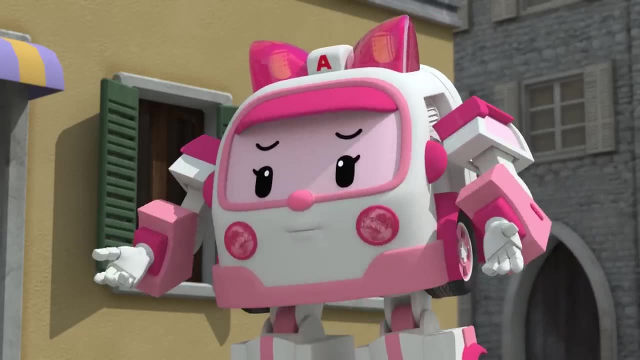 That was a really close call. I'll be careful from now on, Peter. Getting food caught in your throat is quite dangerous Because it makes you unable to breathe When you eat. you can't do it lying down. You must only eat sitting up straight. 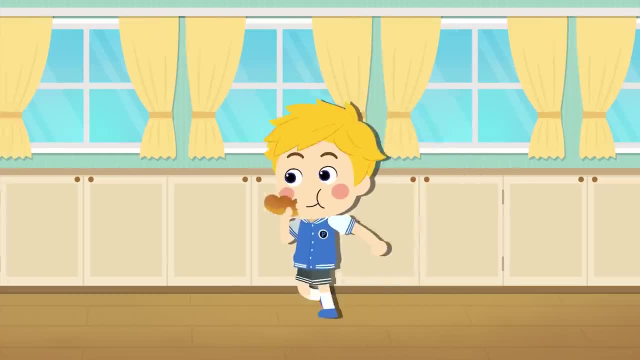 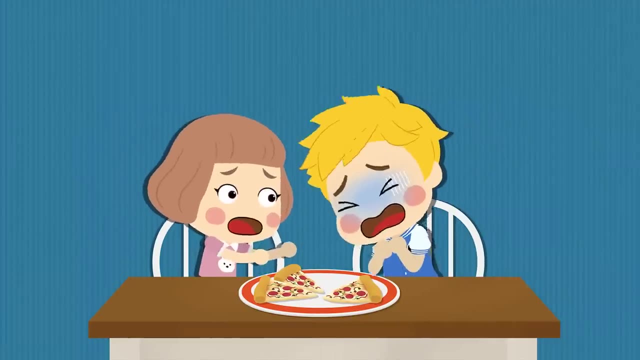 Never eat while you're walking around. Don't talk when you have food in your mouth, Because there's a chance the food will get caught in your throat. If food does get caught in your throat and you can't breathe, you should let someone know right away. 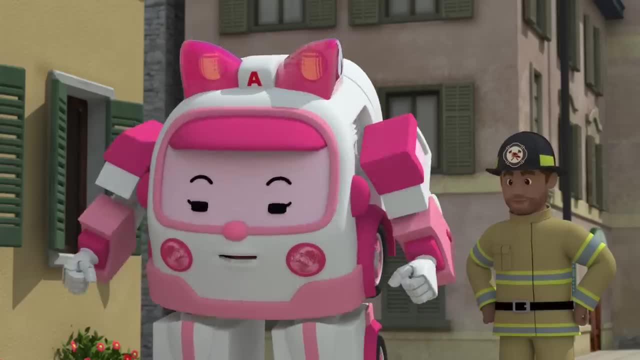 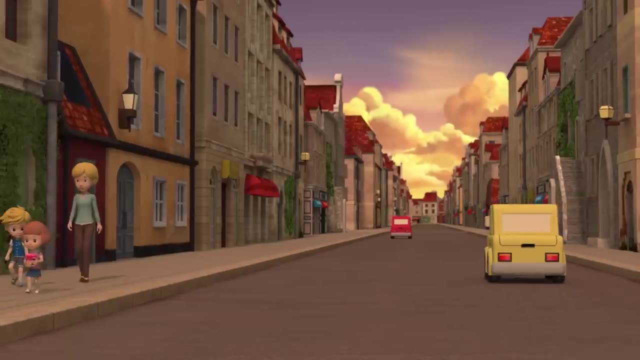 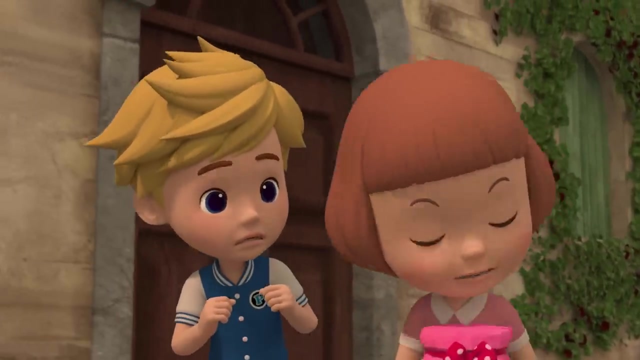 If you can remember that everything should be fine, all right. Oh, I will Amber, Me too. This candy's all mine, Lucy. can I have one? Just one, Amber. just finished explaining to you not to eat while you walk around. 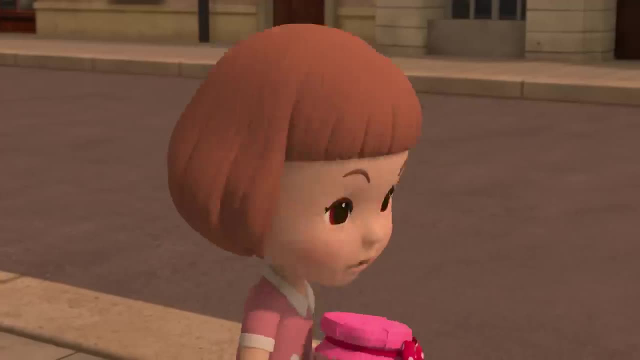 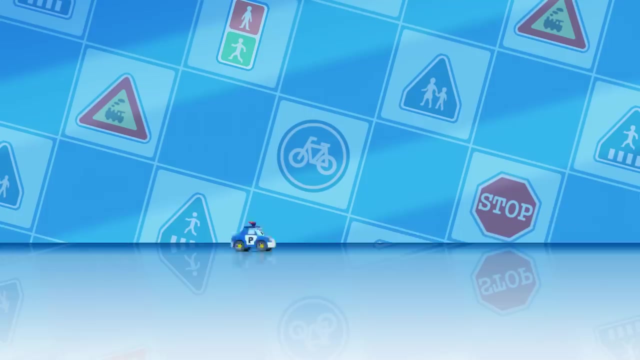 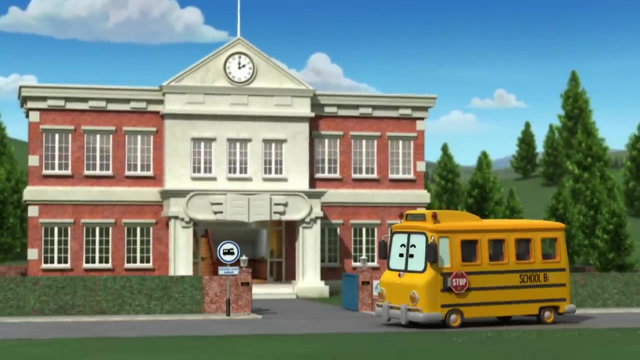 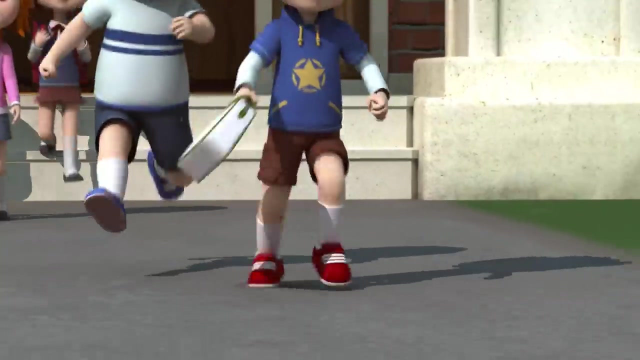 You already forgot. Can I have one at home then? Not a chance, Lucy. please just give me one Please. But I'm begging. Oh, I sure wish Gin would hurry. The kids will be out soon, Look. 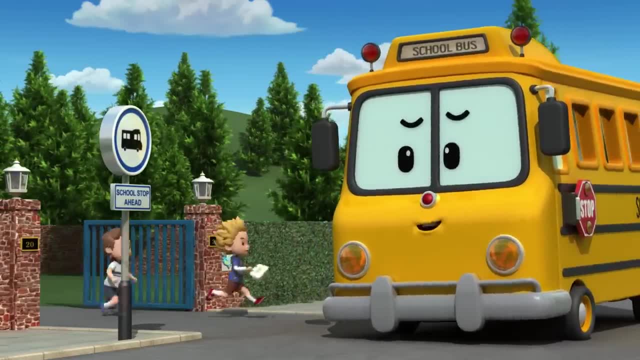 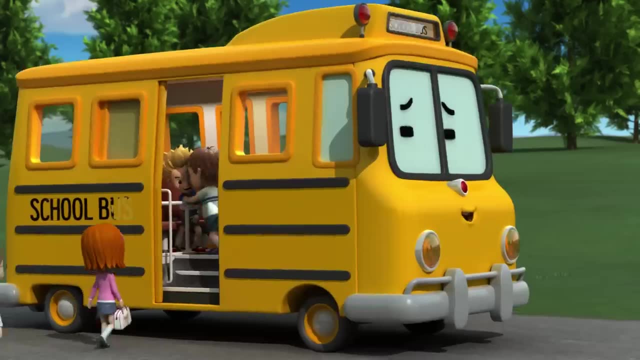 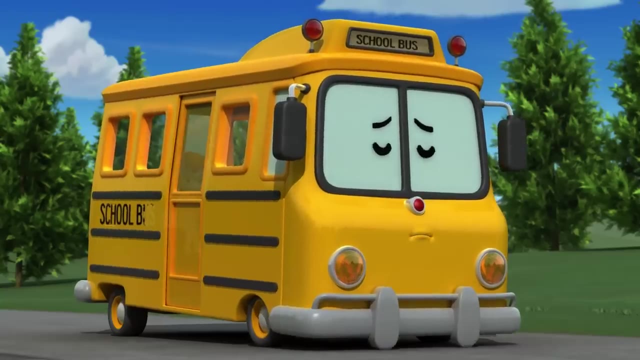 Kevin and Doug are here. Hi, Scooby. Been waiting long, Scooby. No, not really, I get the window No way. Um, excuse me, it isn't safe to misbehave on the bus. boys, Let's go. 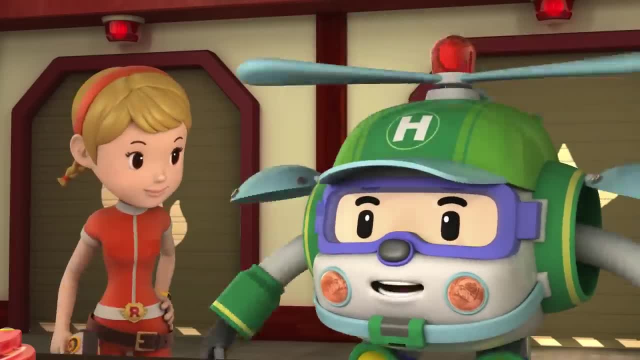 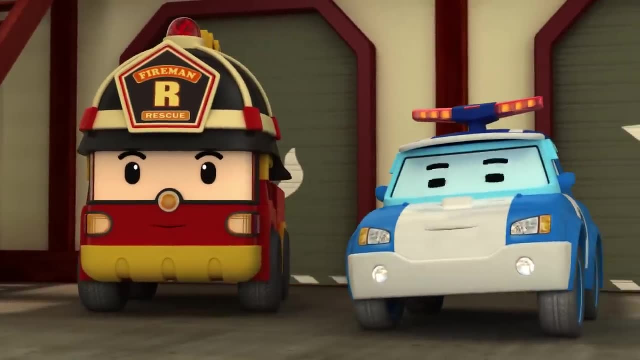 All right, that should do it. What did you make this time? Gin Scooby asked me to come up with a boarding guard. so, Ta-da, What's a boarding guard? Well, it's a safety device that'll help kids. 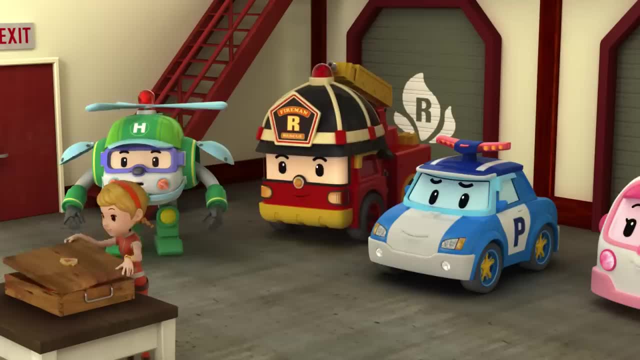 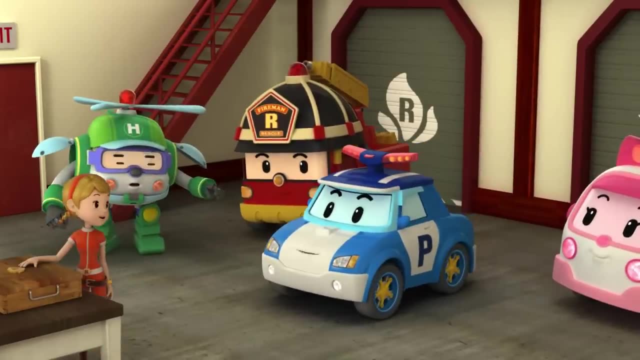 get on and off the bus safely. Oh, what time is it. I was supposed to get this to Scooby. I'll take it to him, Gin. I'm going out on patrol now. Thank you, Polly. Scooby will be so pleased. 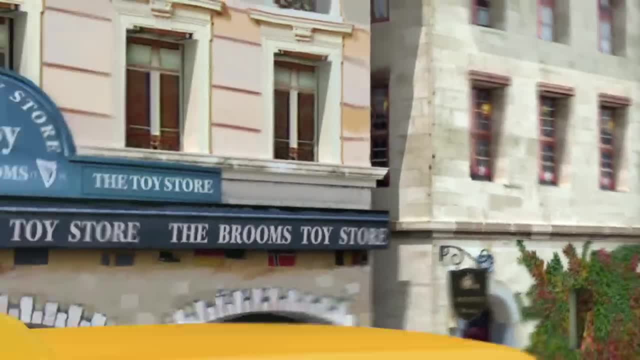 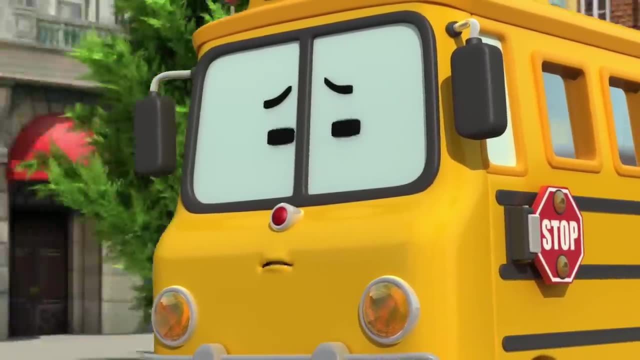 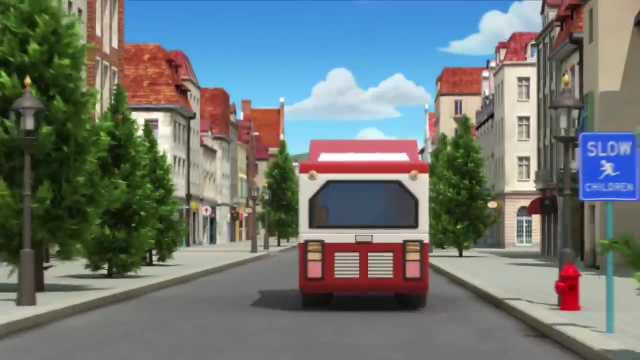 I hope so. Faster, Scooby, Faster, Come on, step on it. Scooby, Please, guys, don't Sticking your heads out the window is something you should never do. He was right, wasn't he? Yeah? 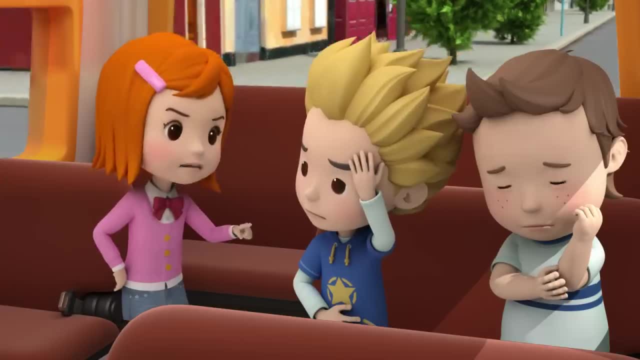 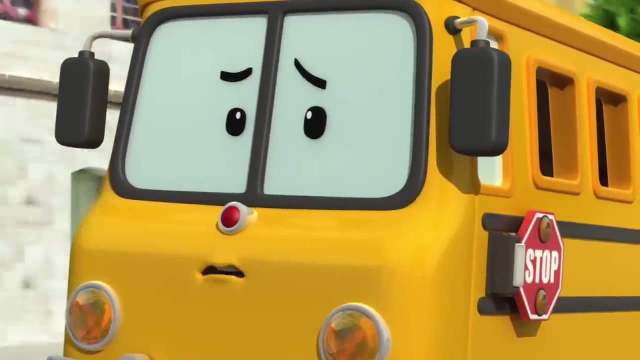 Can't you two just sit still when we're in here? What's the matter with you? I'm listening to you. Please settle down. I need to focus on driving. Please get back to your seat, Ginny. Yes, Scooby. 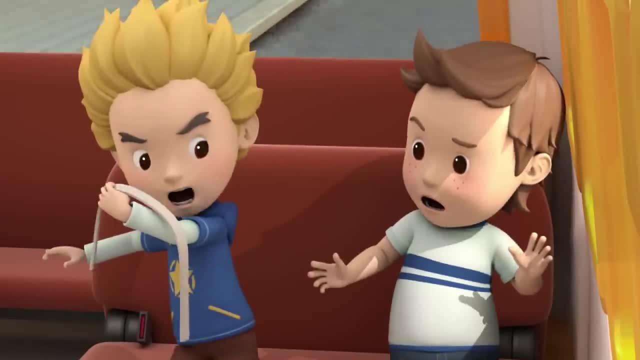 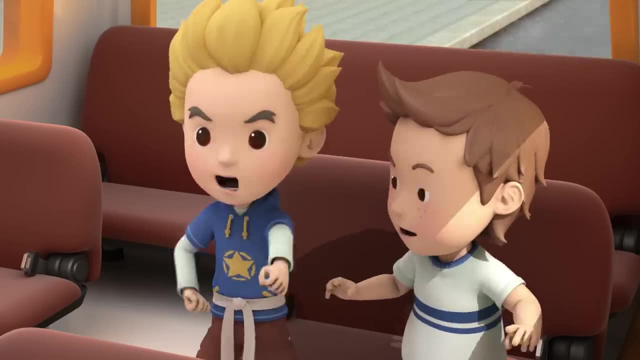 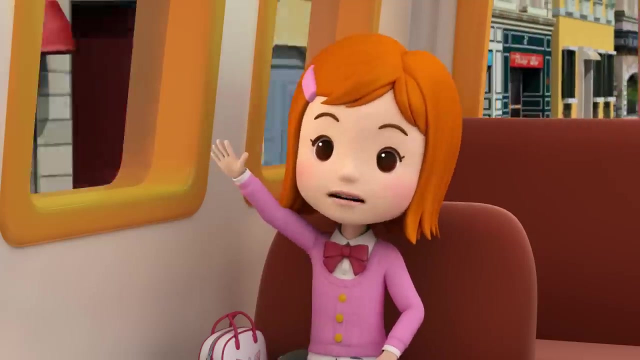 Kev. what's this? Hey, don't touch it, That's mine. This is the belt I wear for Taekwondo. Taekwondo Three, two, one. No, Please stop it. boys, Scooby, I get off here. 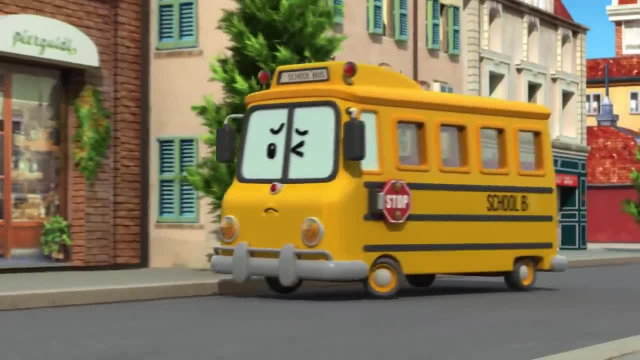 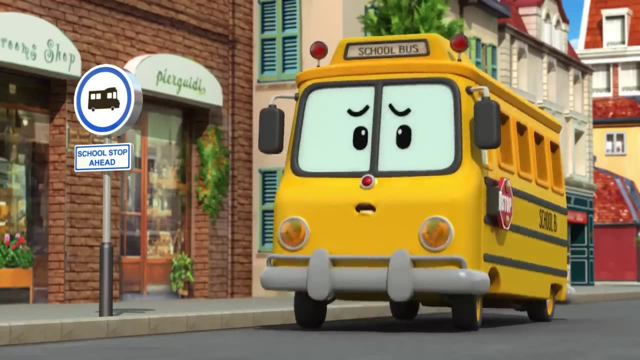 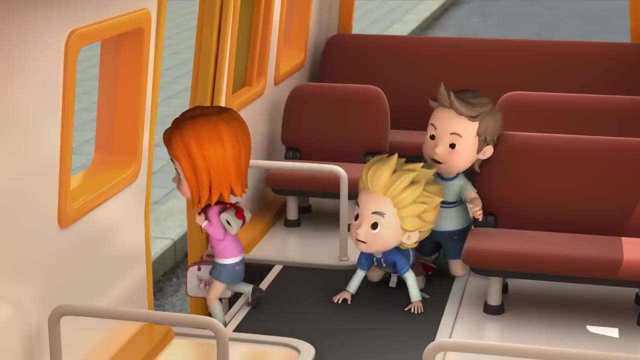 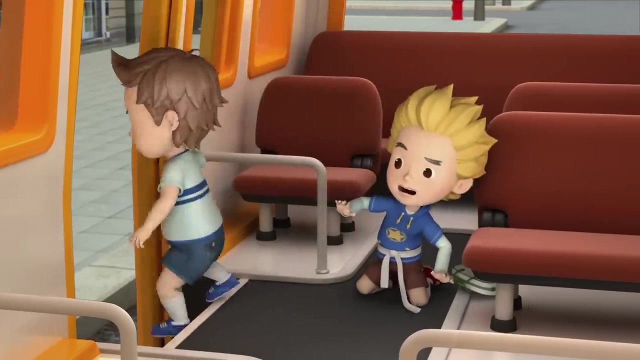 Okay, Ginny Scooby, Are you all right? boys, Excuse me, Whoa A red belt. We're at the gym. Kevin, You need to get off here too. That's right, Me too. Wait for me. 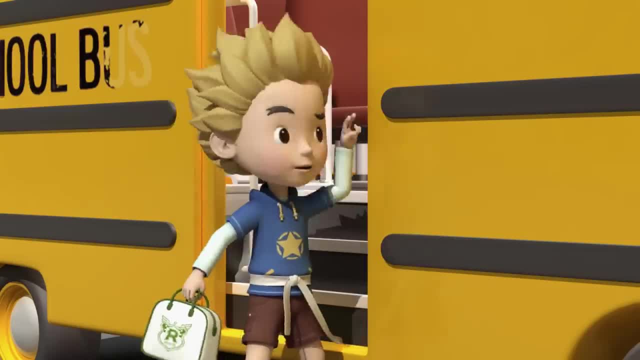 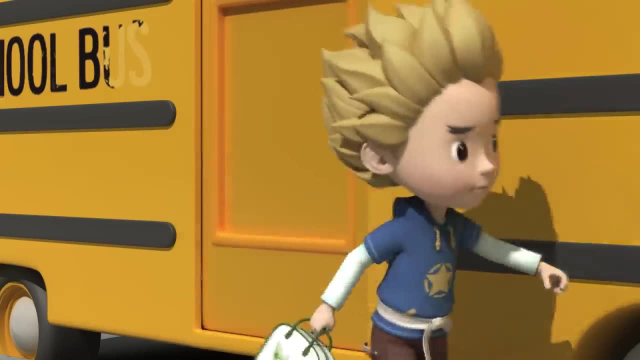 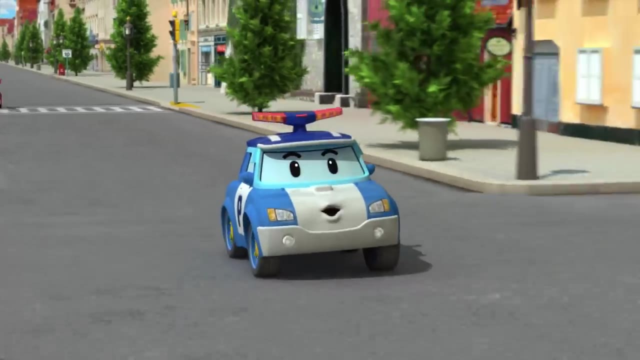 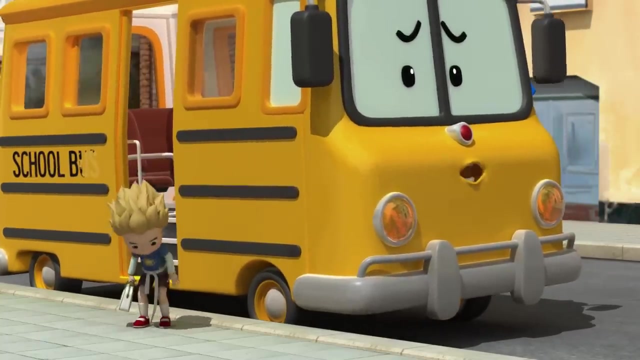 Doug and Kevin are off. What a relief that is. See you tomorrow, Scooby, Oh yeah, Hey, Wait up guys. What's wrong? Kevin? Oh, Scooby, Sorry, Are you okay? Yeah, I'm okay. 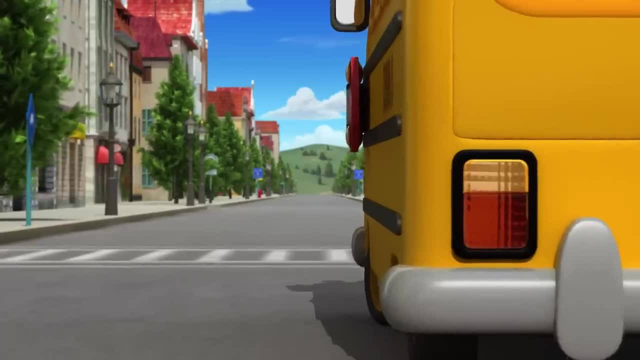 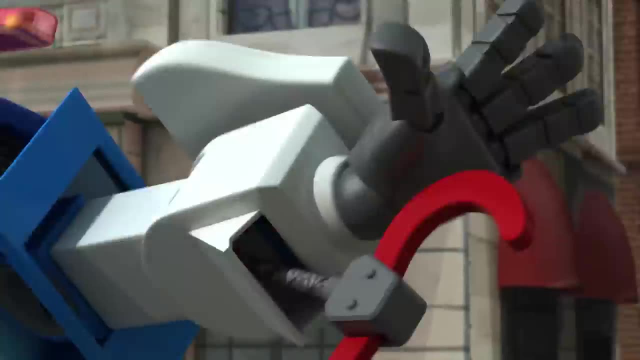 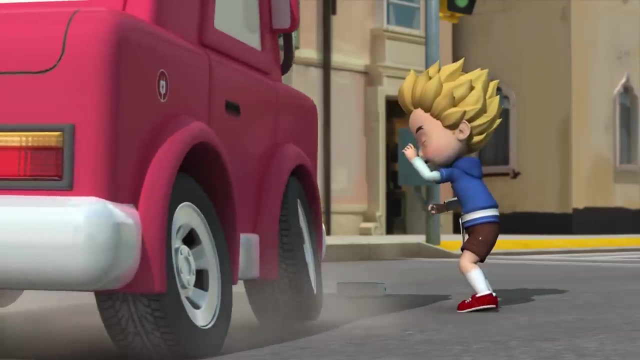 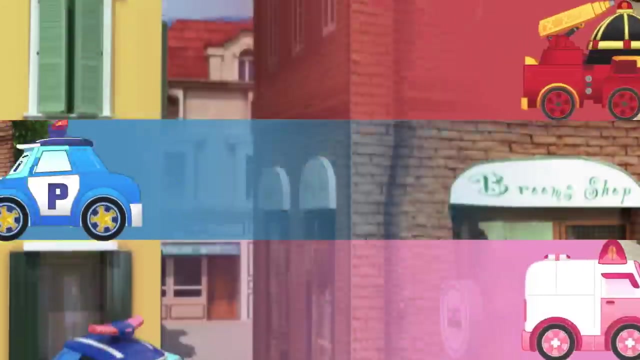 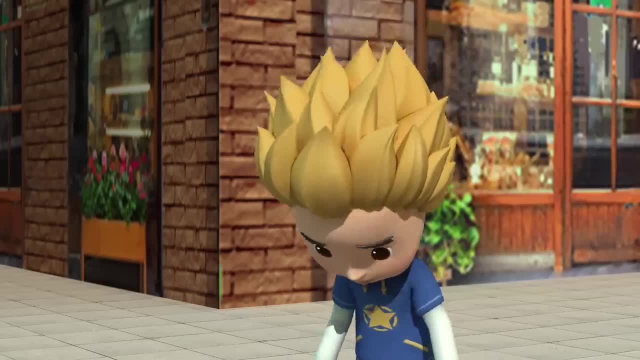 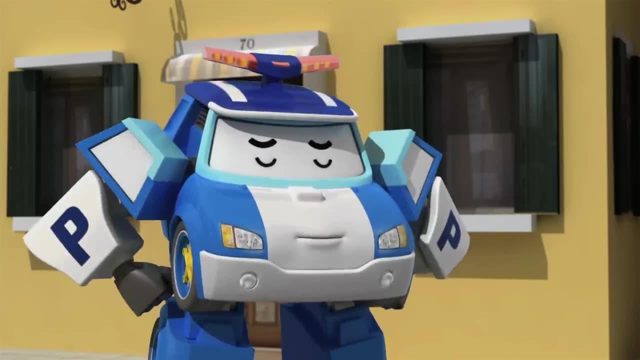 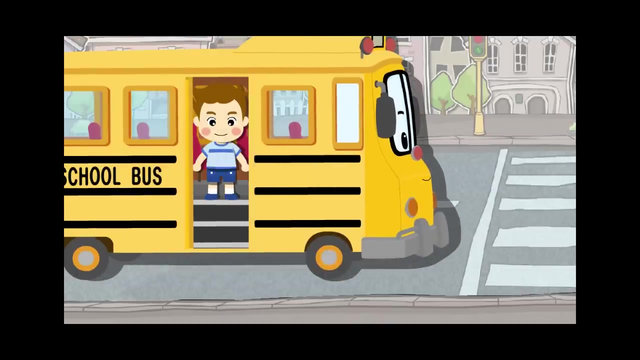 It just isn't safe. Yeah, But I didn't see the car coming. Polly, That's my point. You didn't follow the safety rules. Okay, Can we go through them again? Yeah, When you get off the bus, a motorcycle or bicycle might be coming. 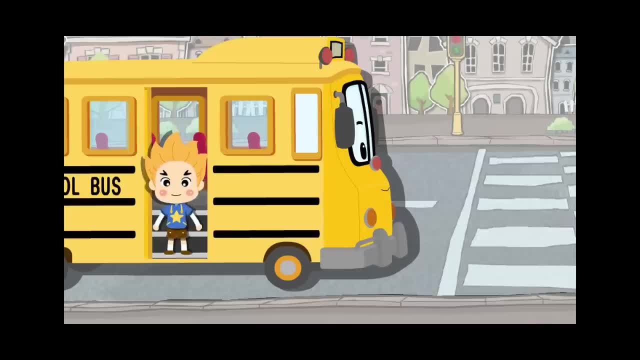 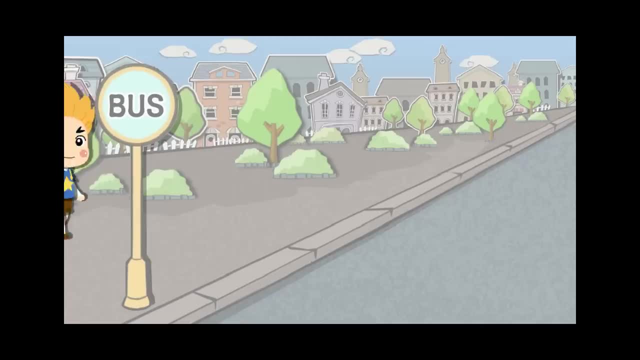 Always look both ways first, then get off slowly. When you get off the bus, never run around the front to cross the street. Drivers can't see you and that's dangerous. Always remember that the doors on a bus or van can be very dangerous too. 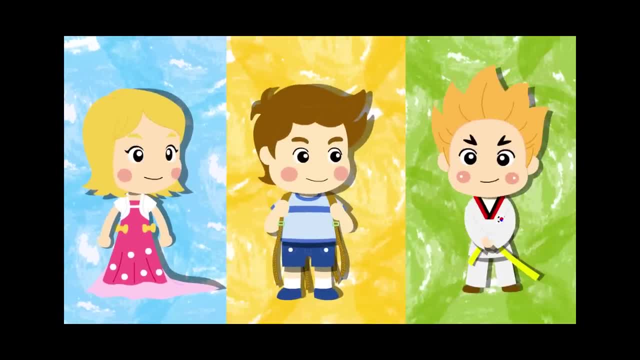 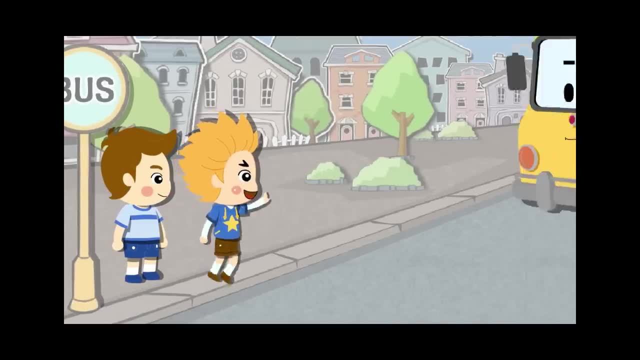 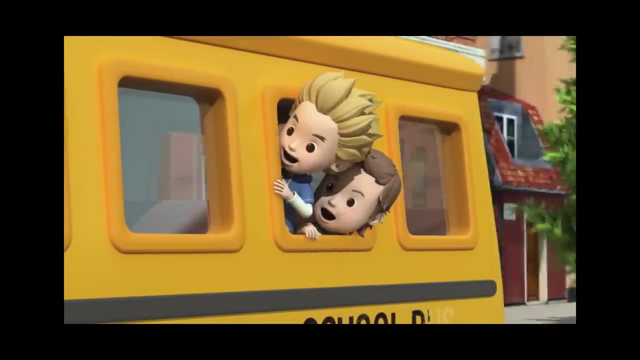 If loose clothes or bags or even belts are hanging out, they can get caught in the doors. Don't let that happen to you. Always wait on the sidewalk for the bus. Never step into the street Playing, fighting, loud talking or leaning out the windows. 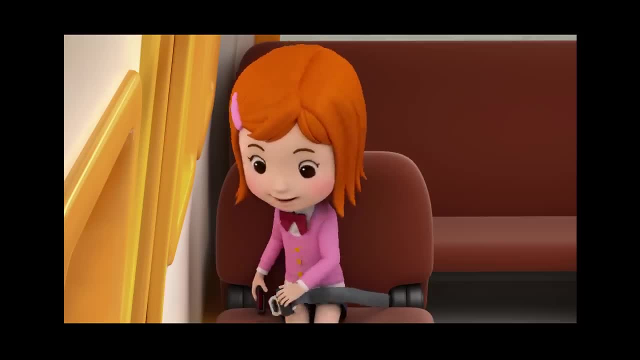 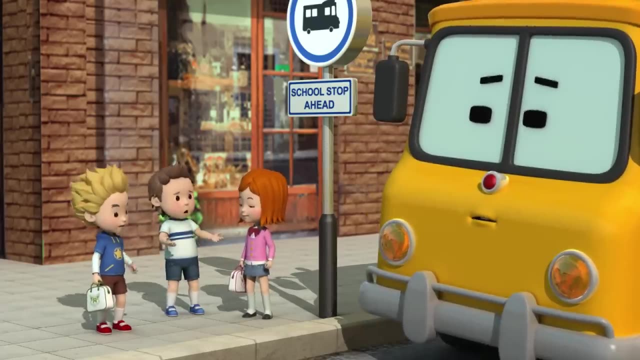 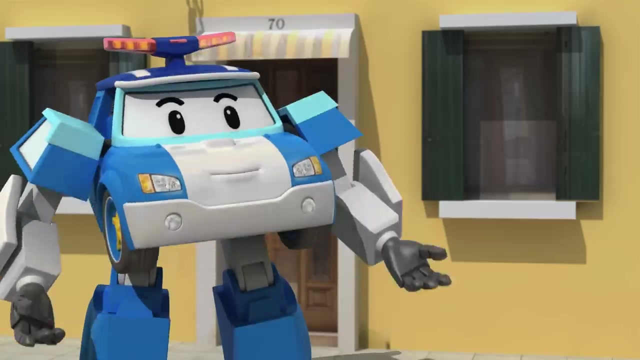 can distract the bus driver and cause accidents. So sit quietly and always wear your seat belt. Scooby, I'm sorry. Yeah, me too. I promise I'll behave from now on, Thanks, boys, And I promise to pay even more attention to safety. 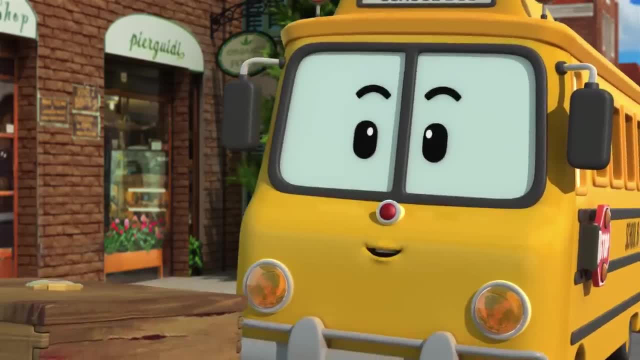 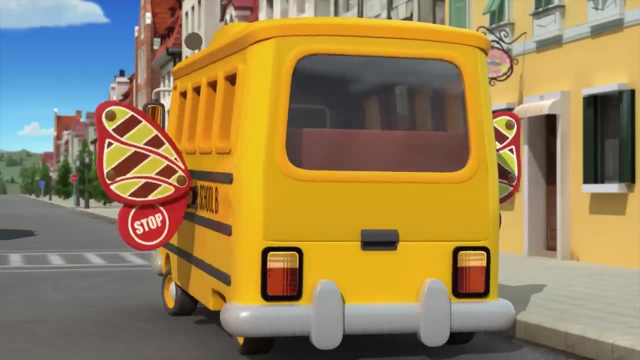 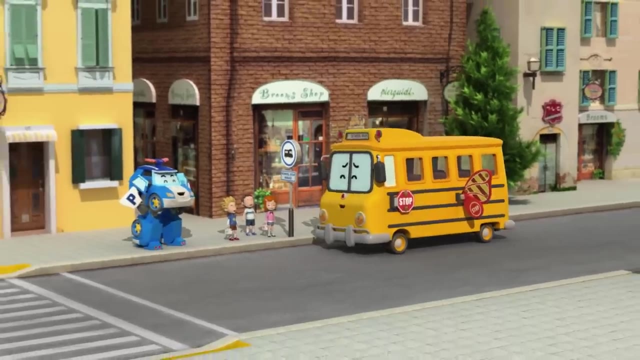 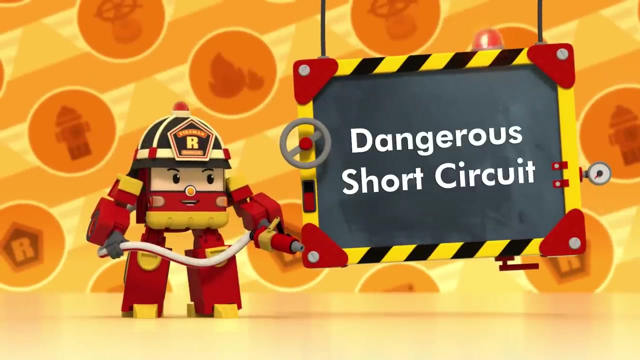 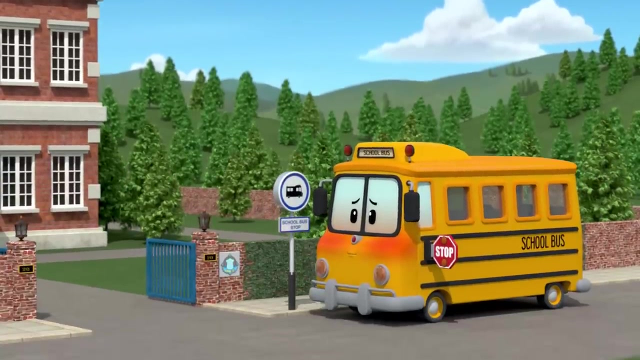 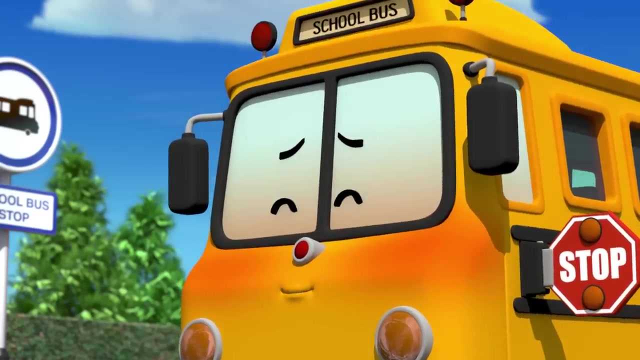 Oh, Scooby, a present for you, A present for me. These look like wings. I'm a bus, not a plane. Goodness, Scooby, Are you sick? No way, I'm all right, Let me off first. 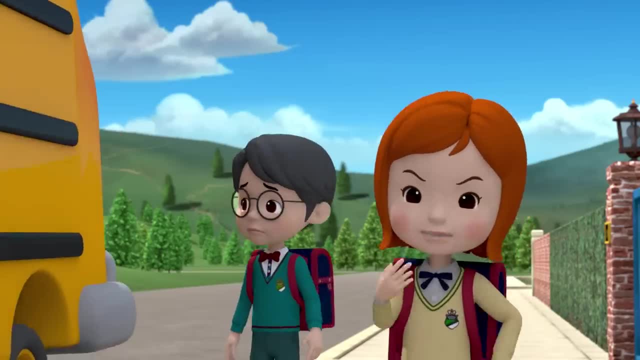 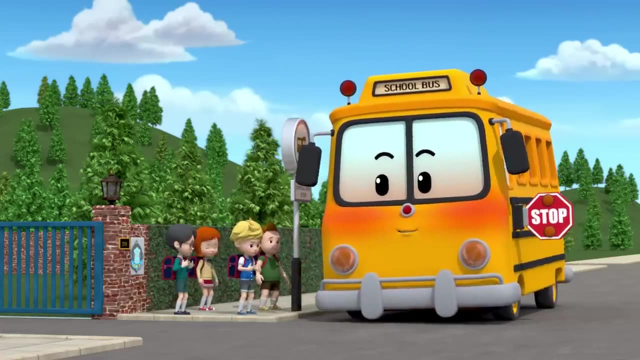 Geez, I got here first, Cut it out. You guys are making Scooby feel even sicker. What Scooby, are you sick? Thanks, but I'm all right, guys, You don't need to worry at all. 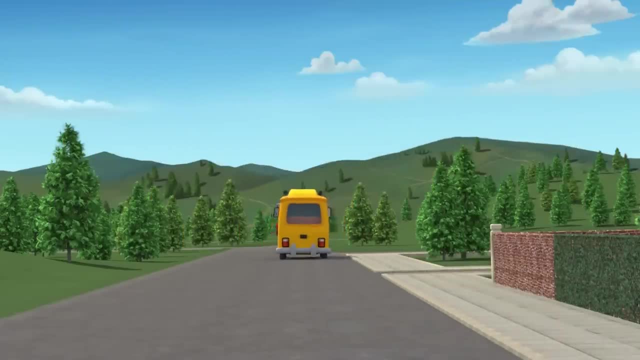 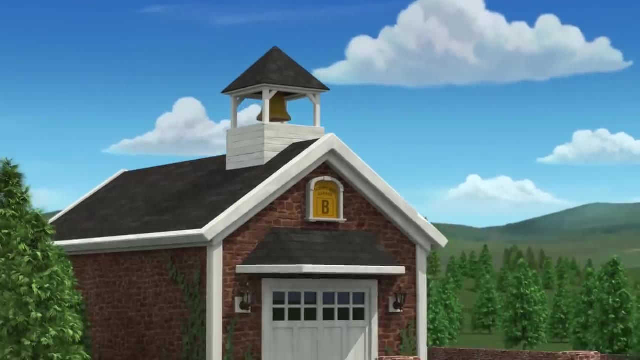 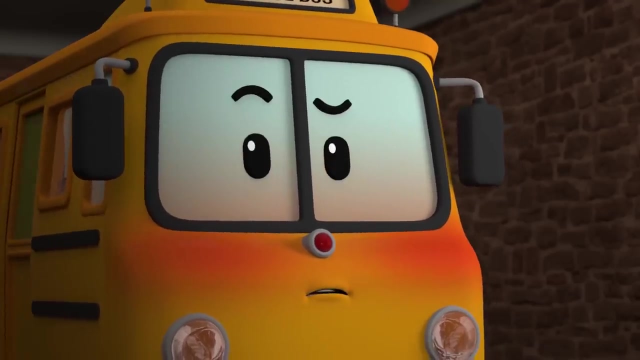 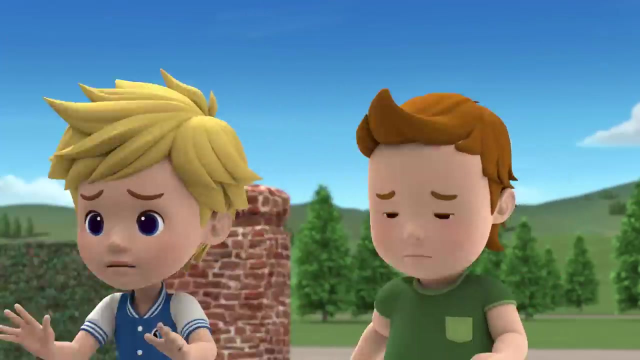 See you after a while. Scooby doesn't look good at all. We made him feel even worse. Nice work, Hmm, Scooby Scooby. Huh, Kids, Scooby Scooby. we were really worried about you. 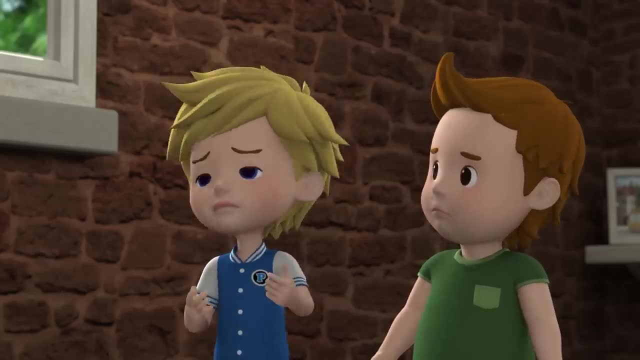 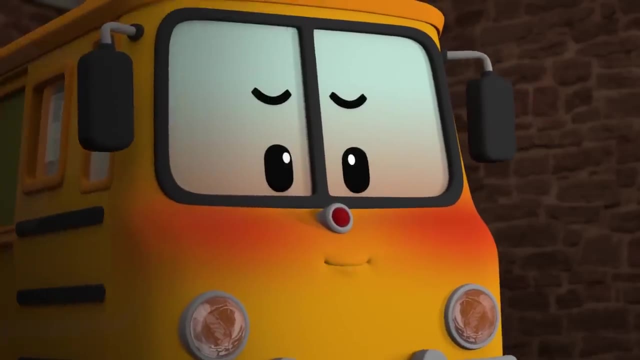 You were Scooby. we're sorry for earlier. Yeah, we're sorry. I didn't know that you were sick. It isn't your fault at all, guys. I've just got a little cold. I just need rest. But thank you all for coming by. 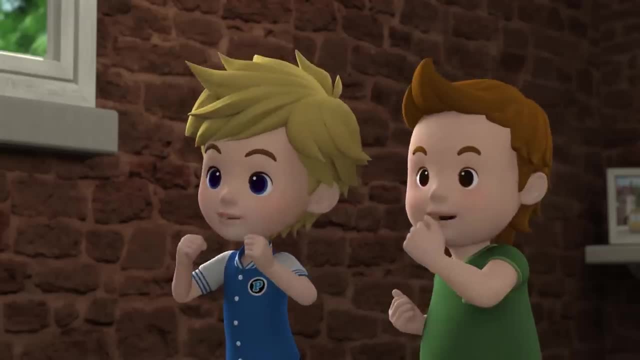 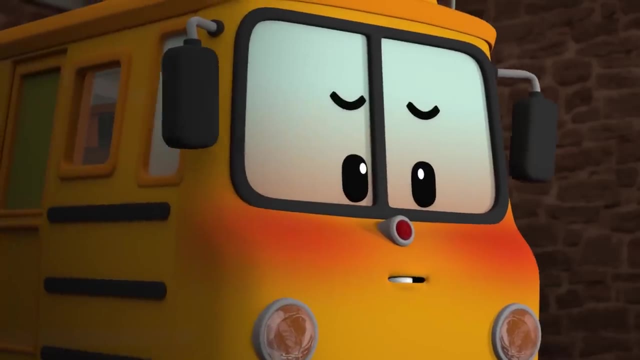 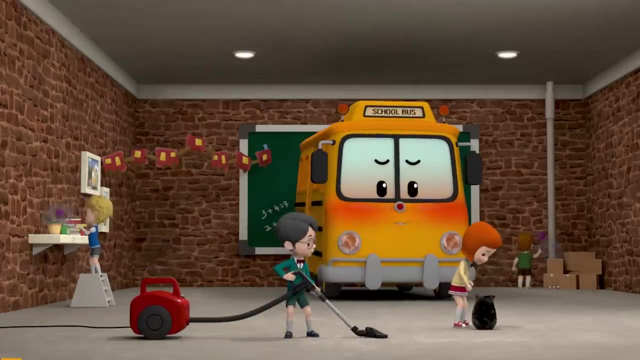 Scooby: Wait, there's more. We brought you some get well stuff. Huh, Just leave it to us, Scooby, We'll take good care of you until you get all better. Yes, we will, Hmm, Hmm. 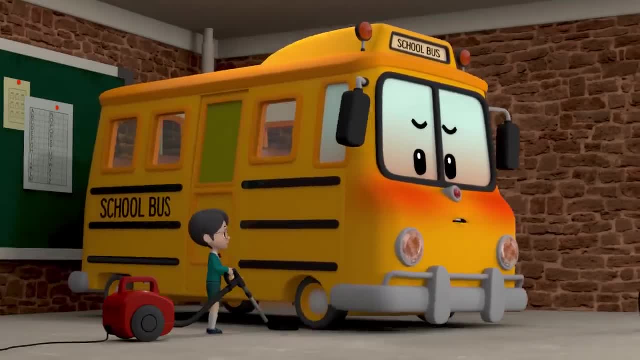 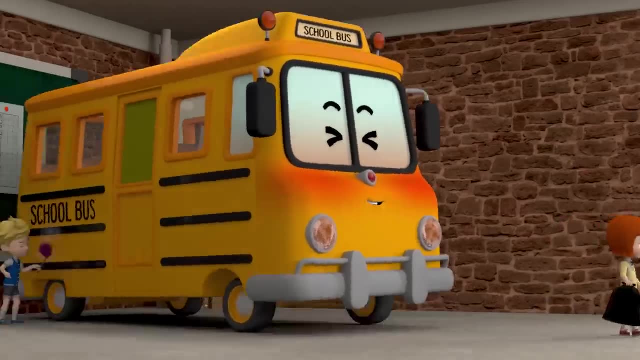 Huh, Scooby, can you please lift your tire up? All right, Scooby. where do you put your garbage? Just right beside the door there. Hahaha, There's dust everywhere. We'll freshen you up, Scooby. 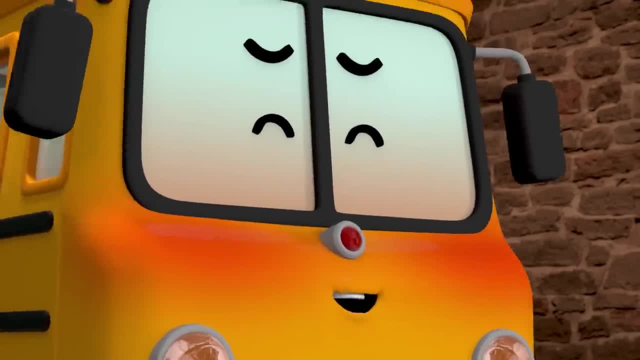 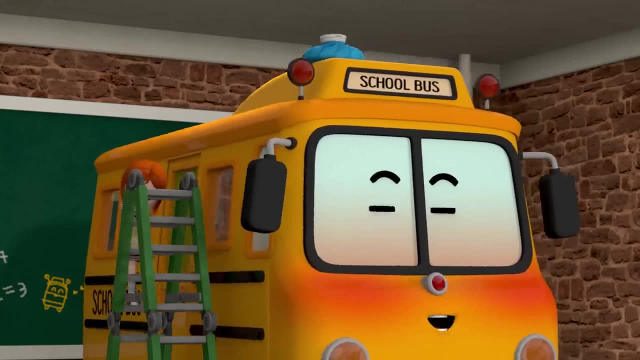 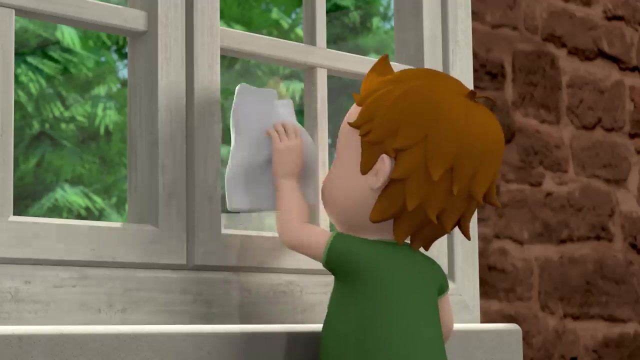 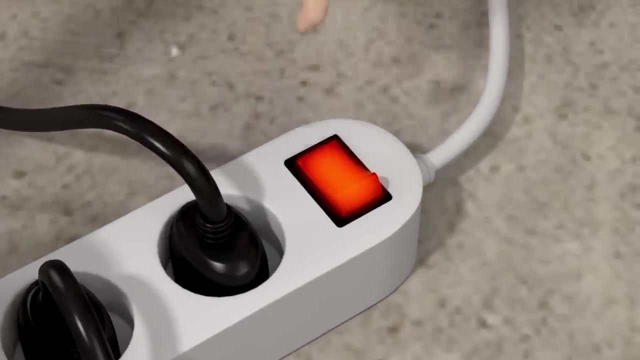 I can't take it. you guys Stop, That's cold. Huh, There, Scooby, How does that feel Cool? That feels nice. Leave everything to us today, There. Yeah, Great work guys, Nice and warm. 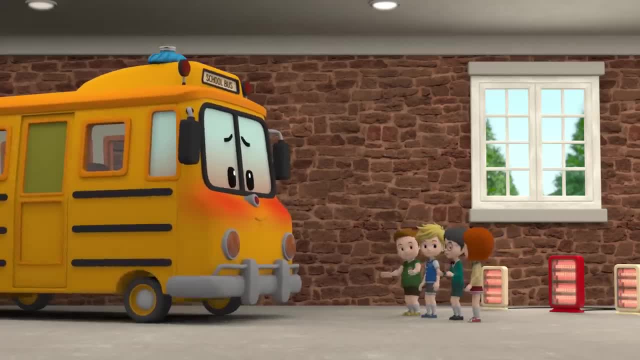 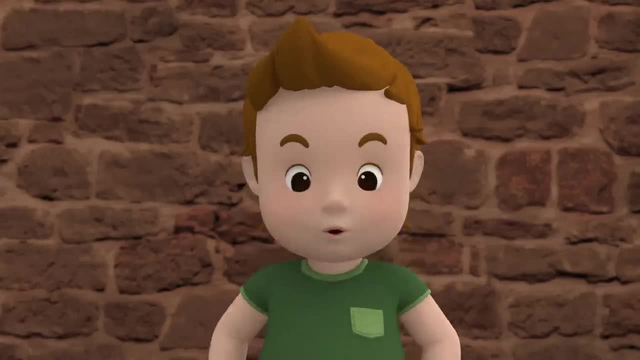 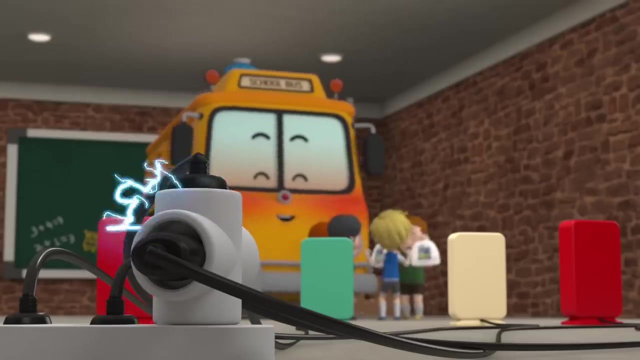 Thanks very much, you guys. You're very welcome. Feel better, Scooby Goodness, I'm really hungry, Me too. Yeah, Good thing I thought to bring a whole bunch of awesome snacks. Haha, Yeah, We have the best. 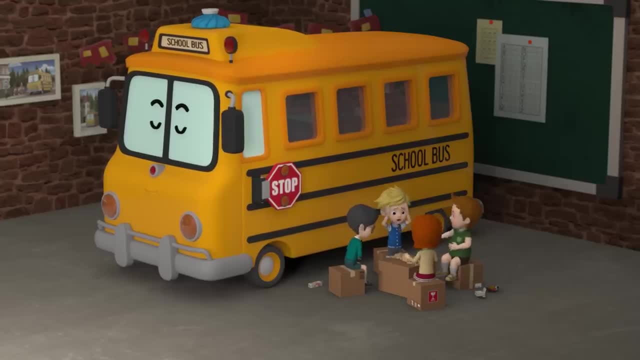 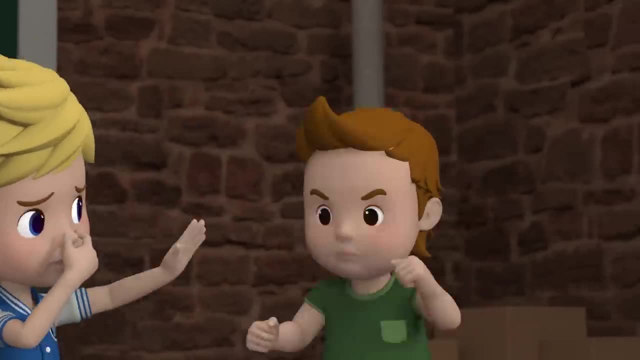 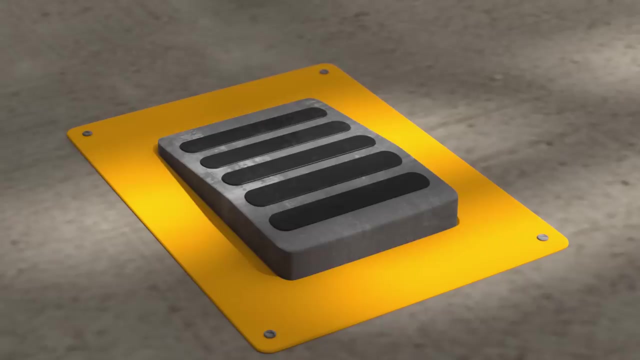 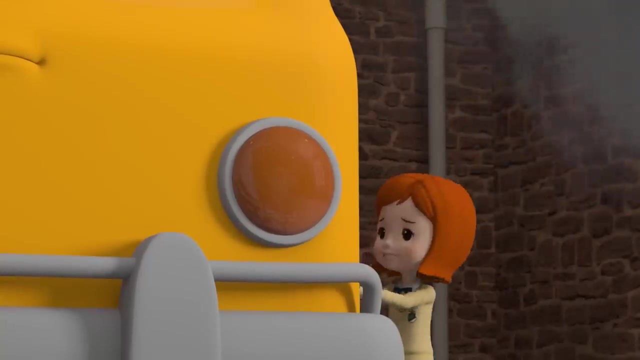 Hahaha, Oh, there it goes. Hahaha, Hey guys, Anybody else smell that? Johnny, stop eating bead dicks. Hey, it's not me. Huh, It smells like fire. Huh, Scooby, Oh, please wake up. 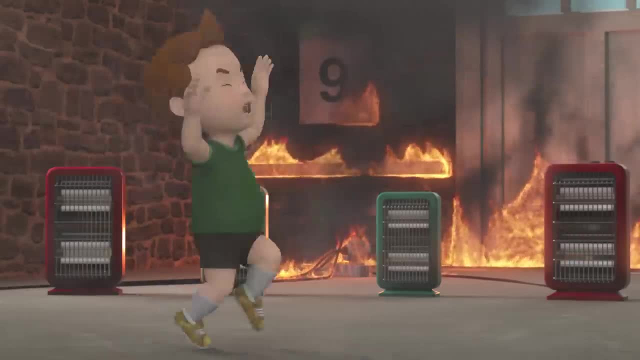 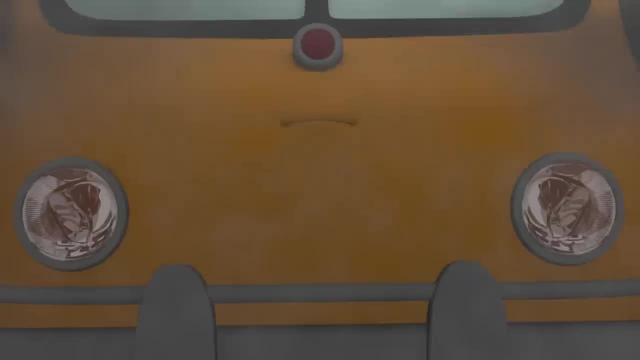 It's a fire, The door won't open. Scooby, Ah, Children, hurry, Climb aboard Now, put on your seat belts and hold on tight. All right, Ah, Huh, Smoke seems to be coming from School Bee's place. 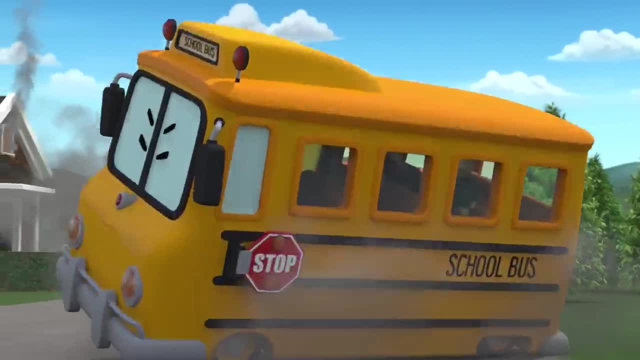 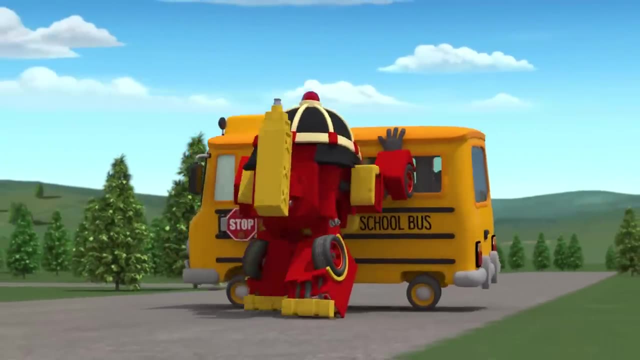 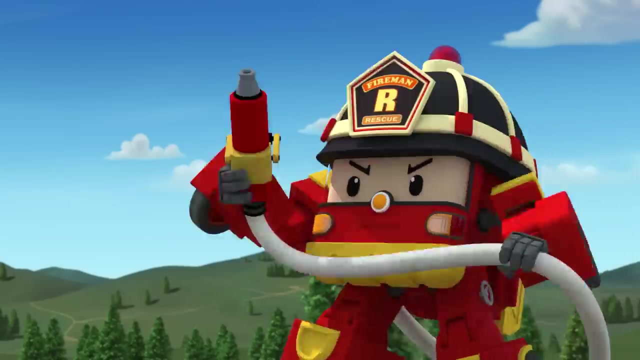 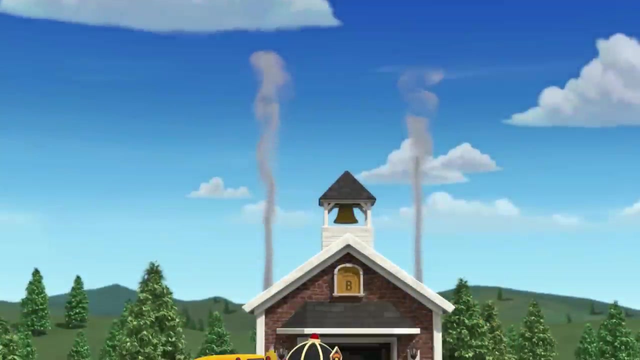 Ah Ah, Look out. Ah Ah Ah. Now, please take the children somewhere safe, Right away. Hmph, Now then That's what happened. It's really good to think of your friends, but you must use your electronics with care. 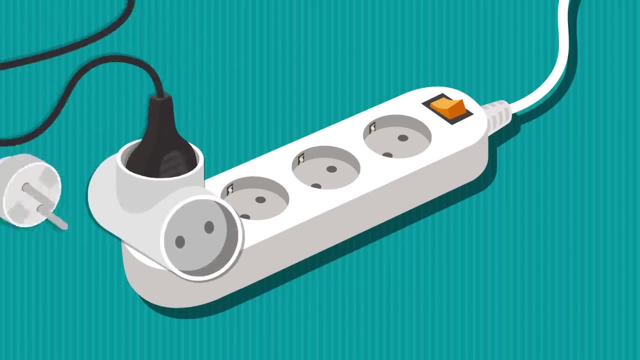 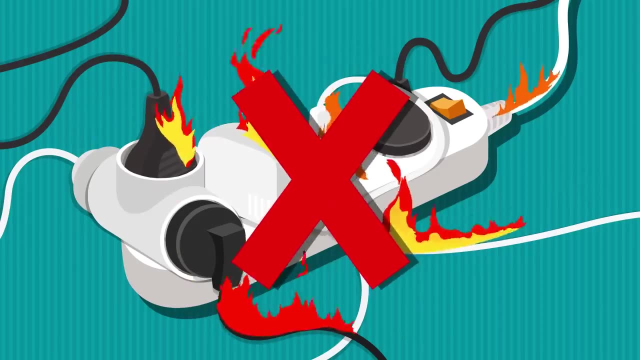 When you plug in devices, don't plug in too many at once. That much current flowing can overheat the outlet, which can lead to a fire. Also, loose plugs can be dangerous. Plugs that aren't pushed in all the way can cause sparks to occur.